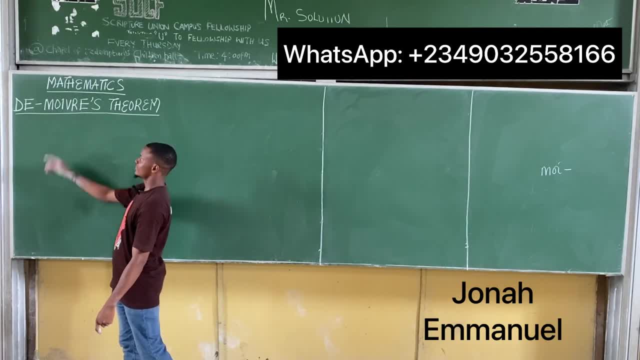 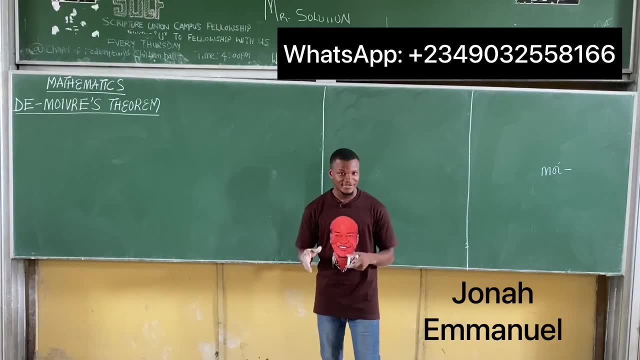 and this one is Moivre. So this is actually the Moivre's theorem, Moivre's theorem as they call it. all right, That's the Moivre's theorem. That's your current pronunciation, But that's, by the way. I think it's quite stressful to pronounce that, isn't it? 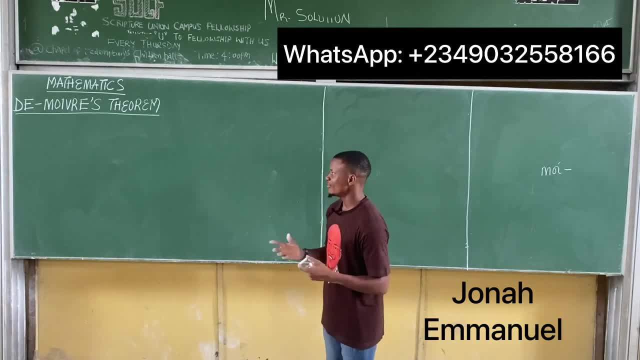 The Moivre's, the Moivre's theorem, the Moivre's theorem. We'll call it in the English form as the Moivre's theorem. It's quite relaxing and much more easier. But that's by the way. Let's get. 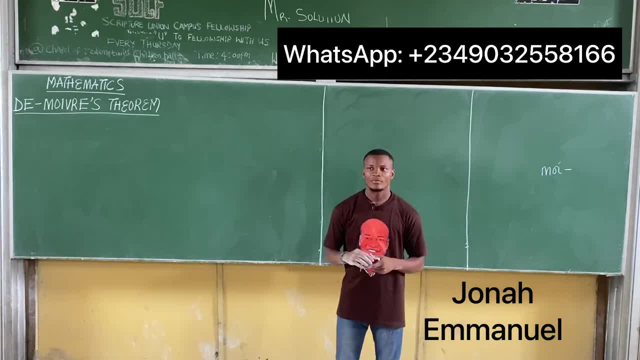 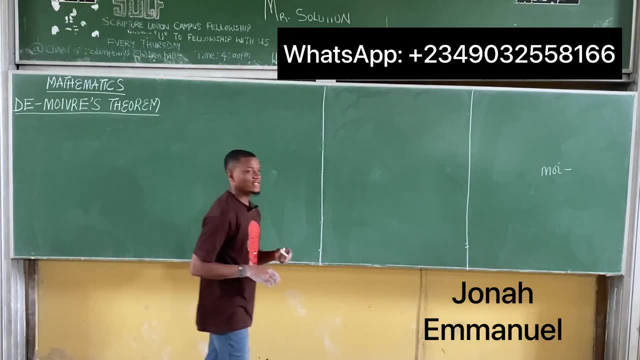 this done, please. What's the concept about the Moivre's theorem? All right, So what does the Moivre's theorem say? For the Moivre's theorem, it helps us to get. the idea of the Moivre's theorem is that it helps us to get the nth power of a complex number. 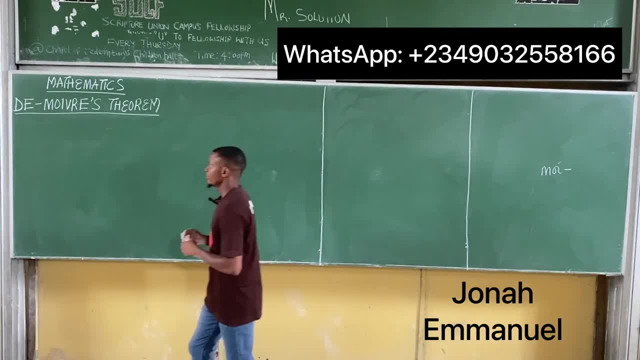 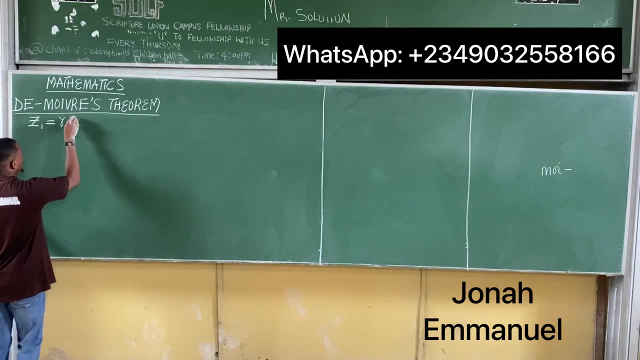 easily and faster too. How do we mean? Remember that in our previous class we talked about the multiplication of complex numbers in polar form. What we say if we have a complex number- z1, and we say z1 is equal to r1, into 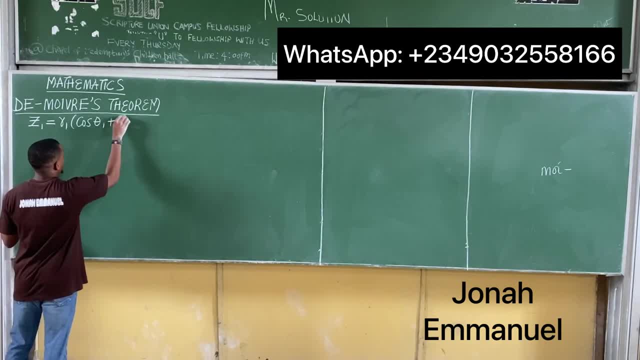 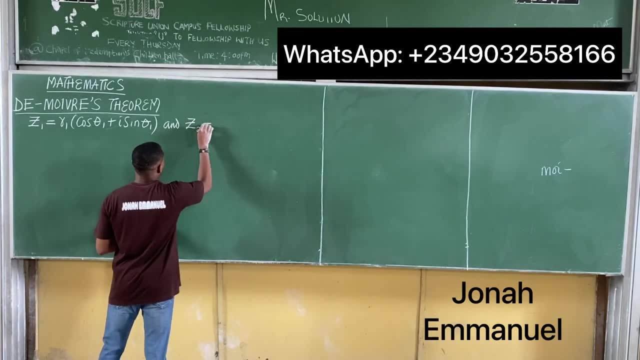 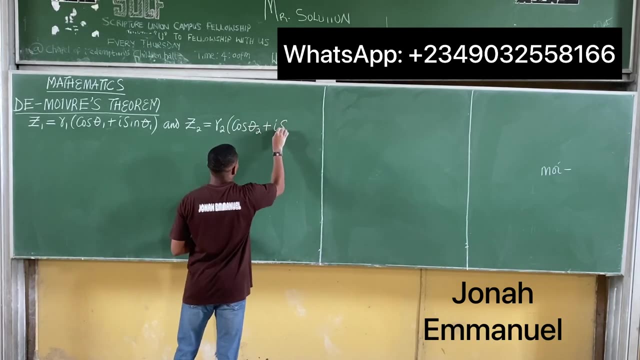 let's say cos theta 1 plus i sine theta 1, and we have z2 has been equal to r2 into cos theta 2 plus i sine theta 2.. So if we have this, then their product z1, z2, their product z1, z2 is equal to. 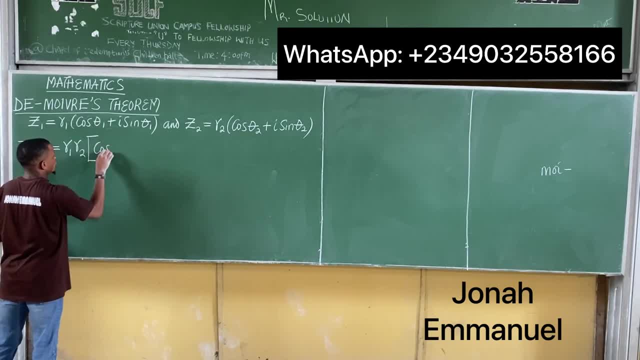 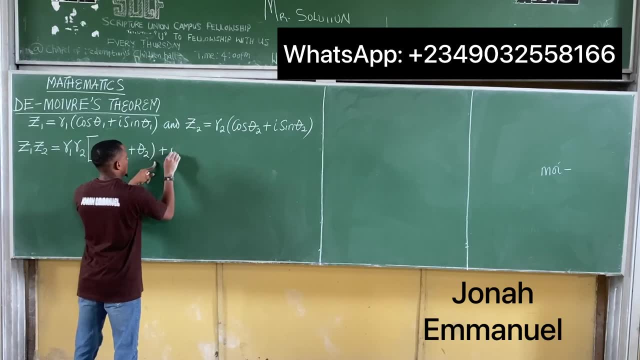 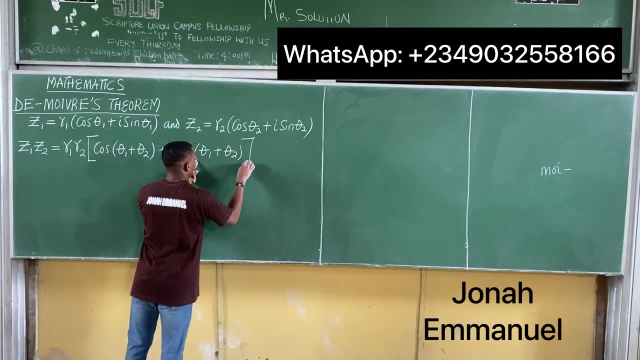 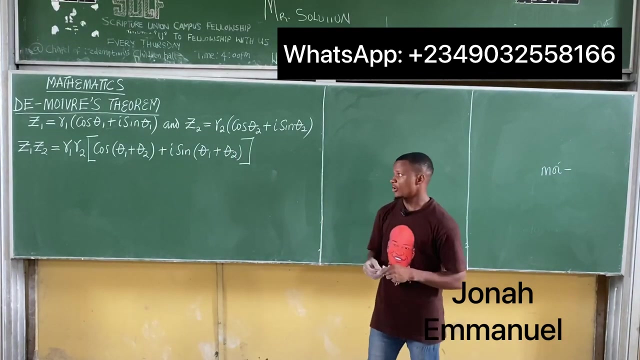 r2 into cos of theta 1 plus theta 2 plus i sine theta 1 plus theta 2.. And you have this. So we talked about this in our previous class, where we did multiplication of complex numbers in polar form. If you missed the, 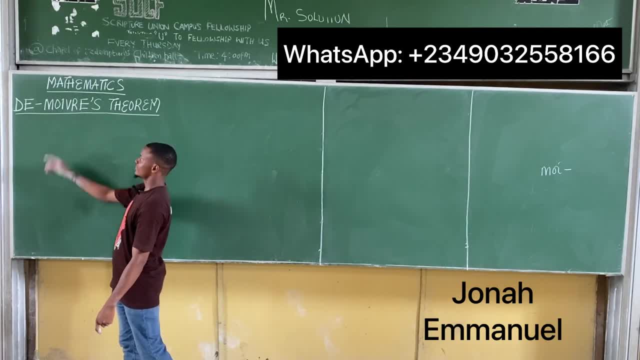 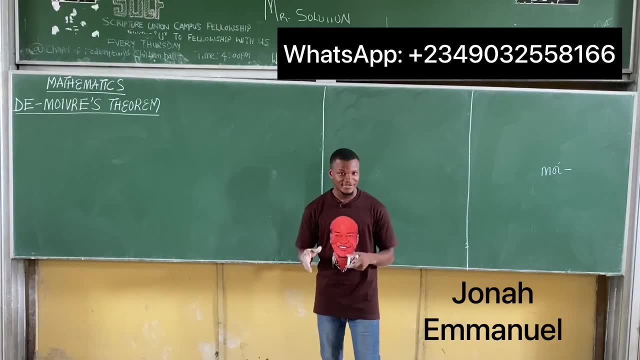 and this one is Moivre. So this is actually the Moivre's theorem, Moivre's theorem as they call it. all right, That's the Moivre's theorem. That's your current pronunciation, But that's, by the way. I think it's quite stressful to pronounce that, isn't it? 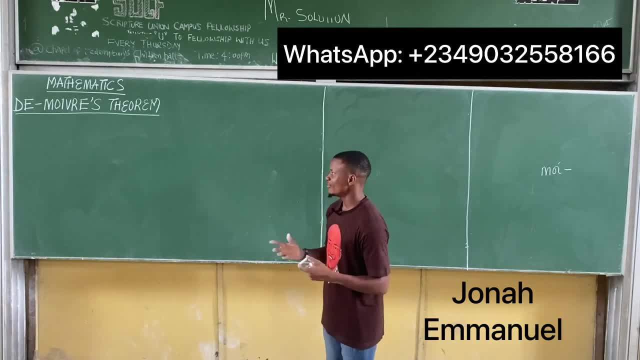 The Moivre's, the Moivre's theorem, the Moivre's theorem. We'll call it in the English form as the Moivre's theorem. It's quite relaxing and much more easier. But that's by the way. Let's get. 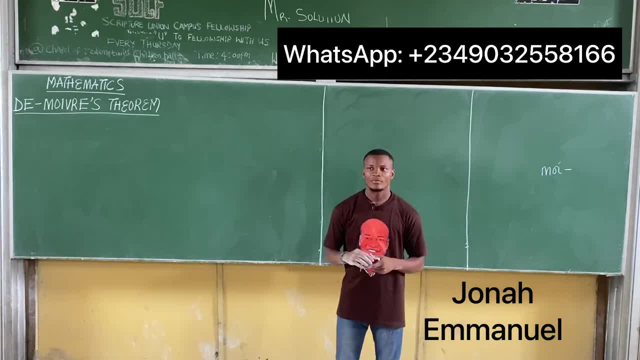 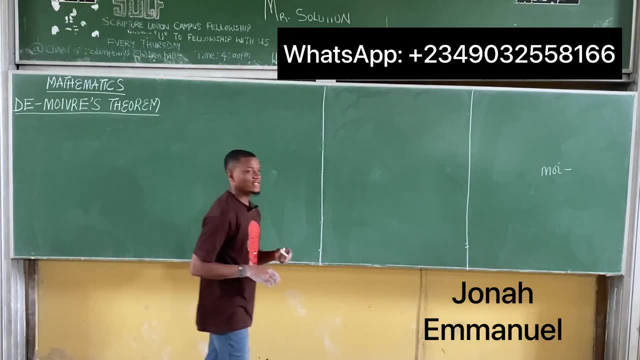 this done, please. What's the concept about the Moivre's theorem? All right, So what does the Moivre's theorem say? For the Moivre's theorem, it helps us to get. the idea of the Moivre's theorem is that it helps us to get the nth power of a complex number. 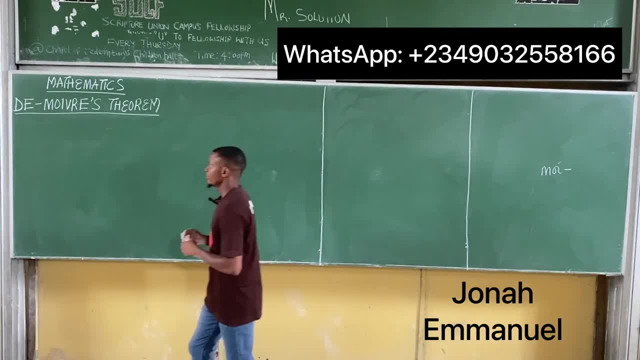 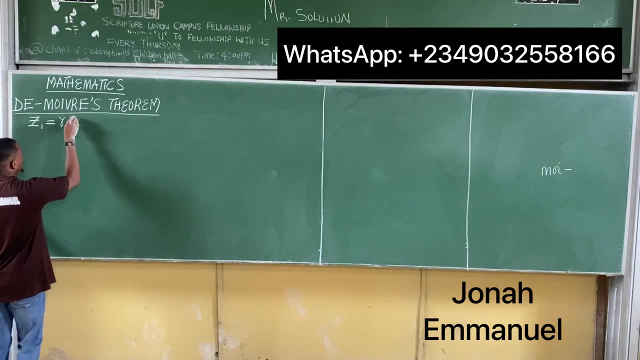 easily and faster too. How do we mean? Remember that in our previous class we talked about the multiplication of complex numbers in polar form. What we say if we have a complex number- z1, and we say z1 is equal to r1, into 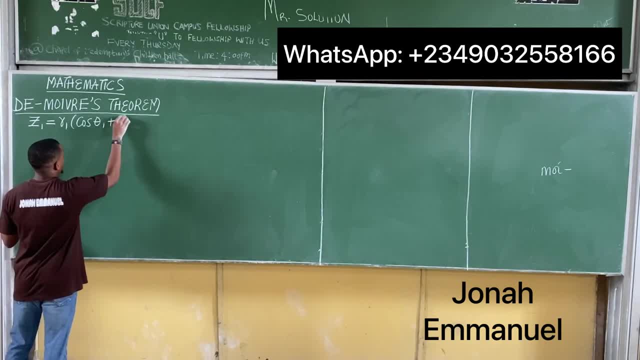 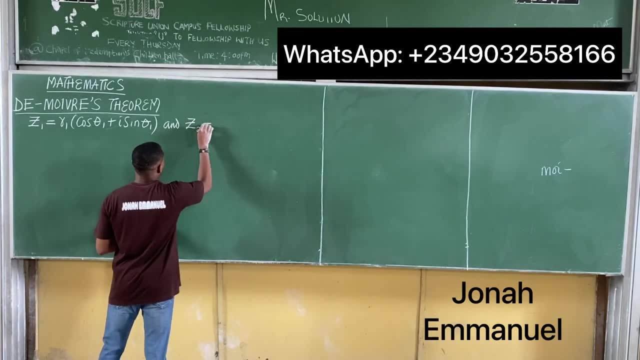 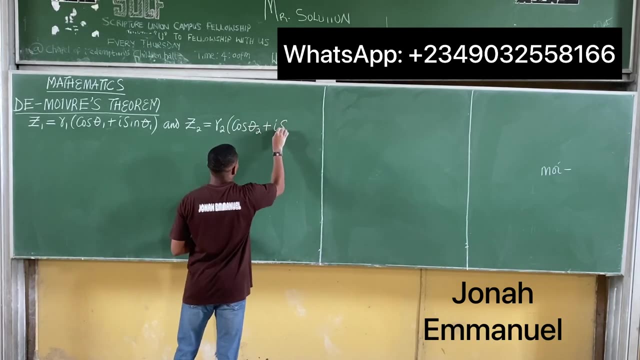 let's say cos theta 1 plus i sine theta 1, and we have z2 has been equal to r2 into cos theta 2 plus i sine theta 2.. So if we have this, then their product z1, z2, their product z1, z2 is equal to. 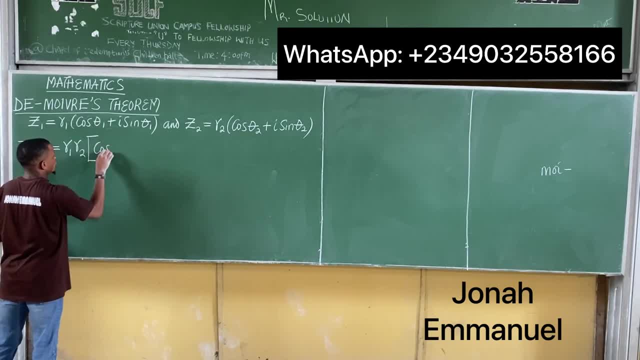 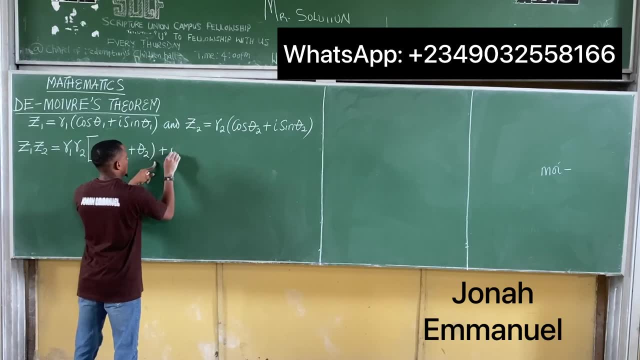 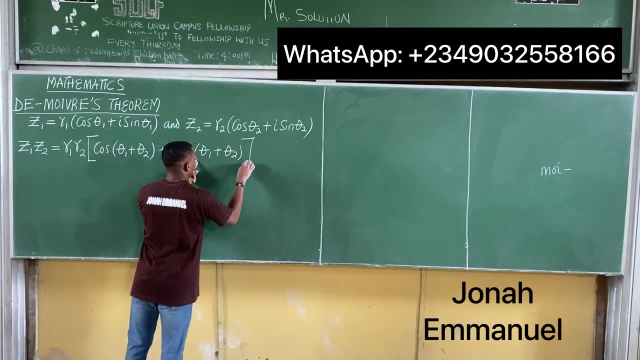 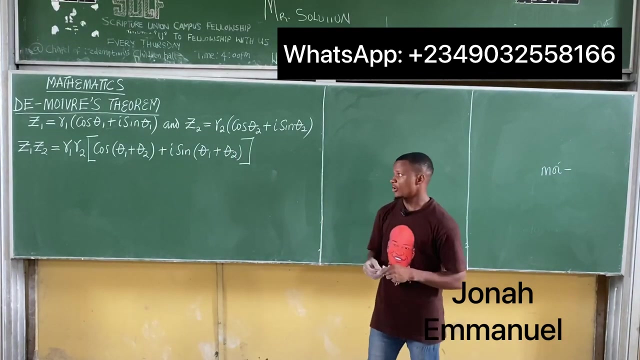 r2 into cos of theta 1 plus theta 2 plus i sine theta 1 plus theta 2.. And you have this. So we talked about this in our previous class, where we did multiplication of complex numbers in polar form. If you missed the, 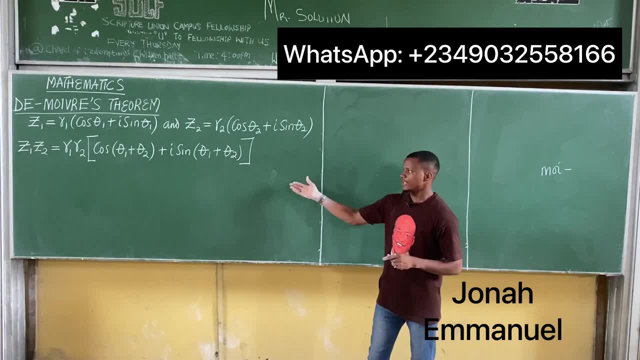 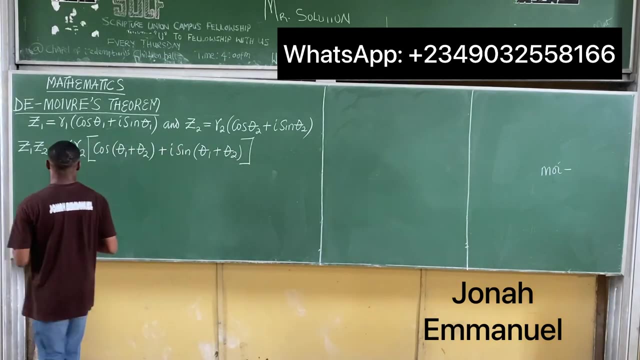 class on this. I'll leave a link to this class in the description of this video. So simply check the description of this video and you'll see a link to this class. Now that's by the way. let's proceed with this. What if, in this case, z1 was equal to z2?? What if z1 and z2 were the? 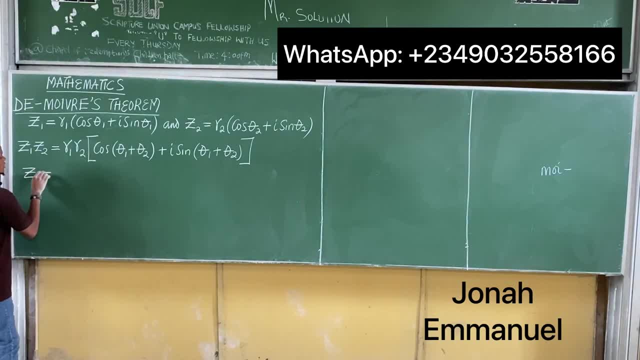 same thing. So let's say z1 was equal to z2 and that's equal to r. no longer r, no longer r1,, just r into cos, theta 1, or let's just call this theta. no longer 1 and 2,, just theta plus i, no longer. 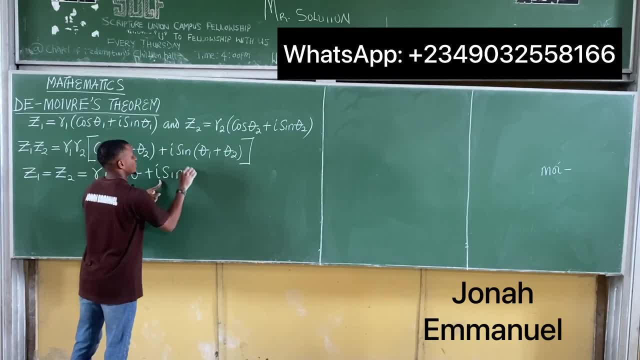 sine theta- 1 and 2, but just sine theta. So I have this. So if z1 is equal to z2, and that's equal to this one here, no longer 1 and 2,- if I multiply them I'll have z1 dot z2.. Since they're the same, 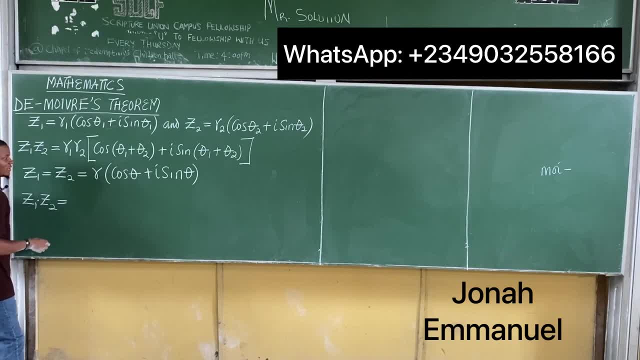 thing. we can call them. just one thing, Perhaps we can call them. let's just call them z right, So z squared, for instance, because z1 and z2 are the same thing. So if it's z1 times z2, whichever way, let's just call it z. 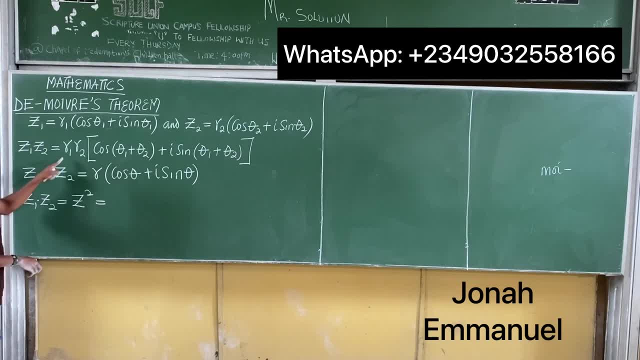 all right. If it's being squared, this will be equal to now. you have r1 times r2, but we said r1 and r2 are the same thing, So it becomes r times r, which is r squared into now. this will become: 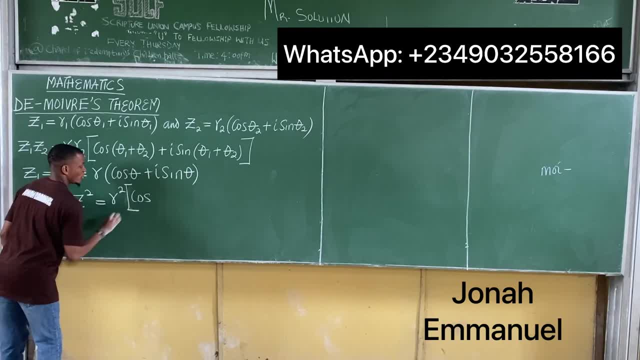 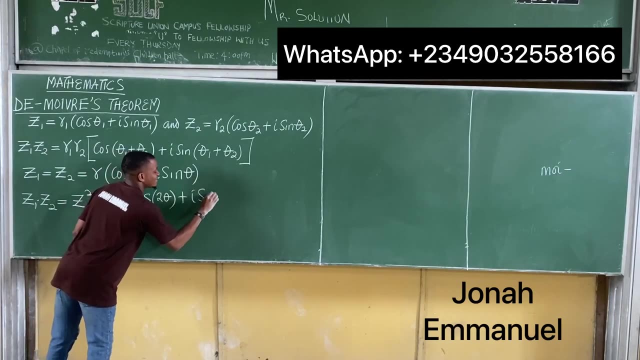 cos now I'll be having theta 1 plus theta 2, but theta 1 and theta 2 are the same thing. So it will be what there? Theta plus theta, that's 2, theta plus i sine- same thing here. 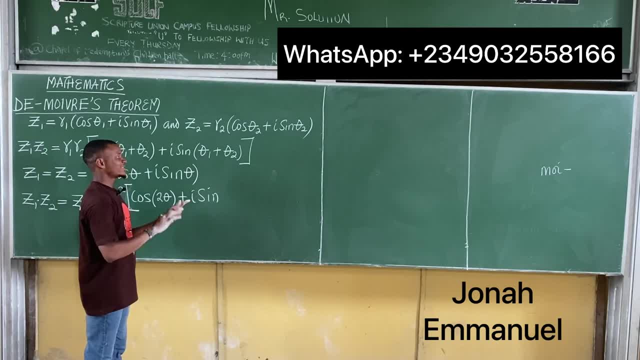 we are saying that theta and theta are the same thing, no longer theta 1 and theta 2.. So I'll be having theta plus theta. that will give you 2 theta, So I will have this one here. So please. we are saying that z1 and z2 are the same thing, So z1 times z2. 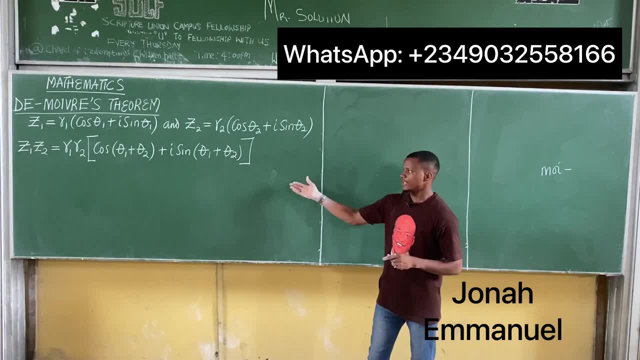 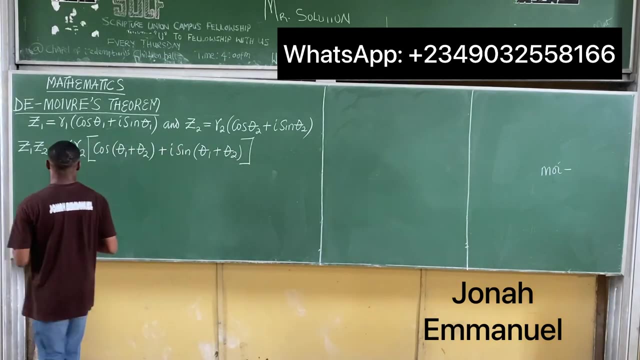 class on this. I'll leave a link to this class in the description of this video. So simply check the description of this video and you'll see a link to this class. Now that's by the way. let's proceed with this. What if, in this case, z1 was equal to z2?? What if z1 and z2 were the? 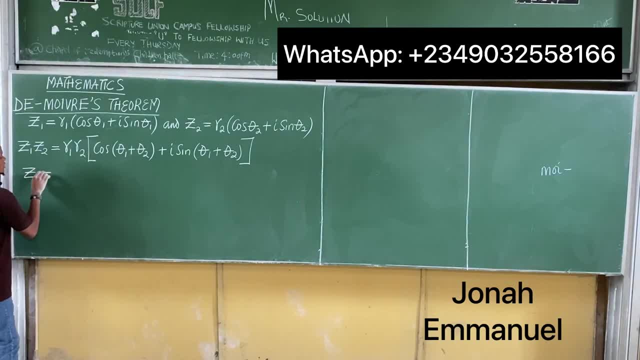 same thing. So let's say z1 was equal to z2 and that's equal to r. no longer r, no longer r1,, just r into cos, theta 1, or let's just call this theta. no longer 1 and 2,, just theta plus i, no longer. 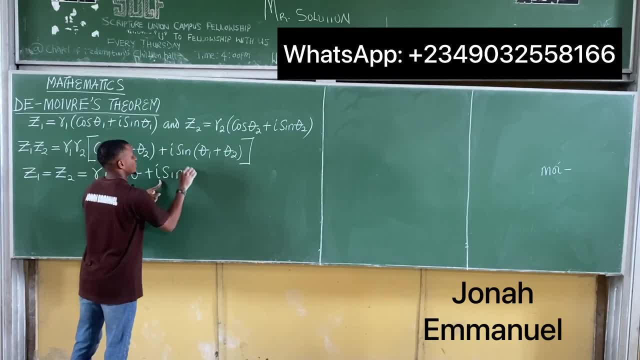 sine theta- 1 and 2, but just sine theta. So I have this. So if z1 is equal to z2, and that's equal to this one here, no longer 1 and 2,- if I multiply them I'll have z1 dot z2.. Since they're the same, 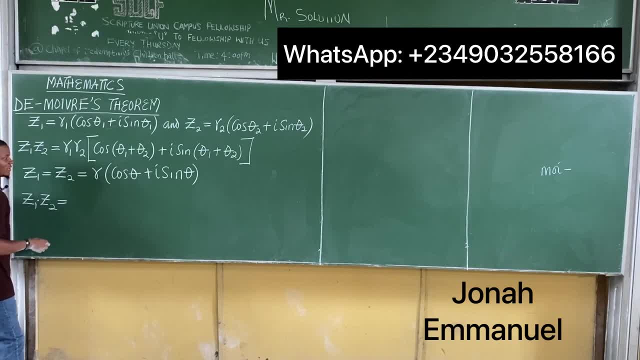 thing. we can call them. just one thing, Perhaps we can call them. let's just call them z right, So z squared, for instance, because z1 and z2 are the same thing. So if it's z1 times z2, whichever way, let's just call it z. 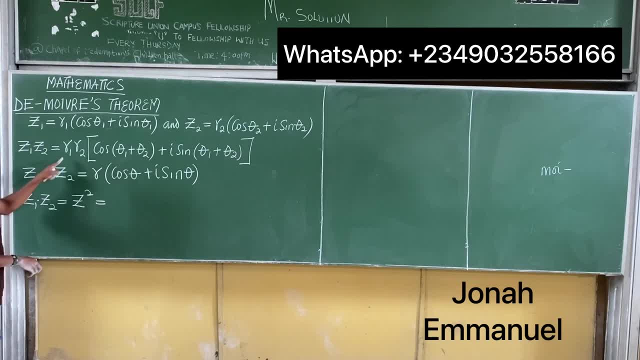 all right. If it's being squared, this will be equal to now. you have r1 times r2, but we said r1 and r2 are the same thing, So it becomes r times r, which is r squared into now. this will become: 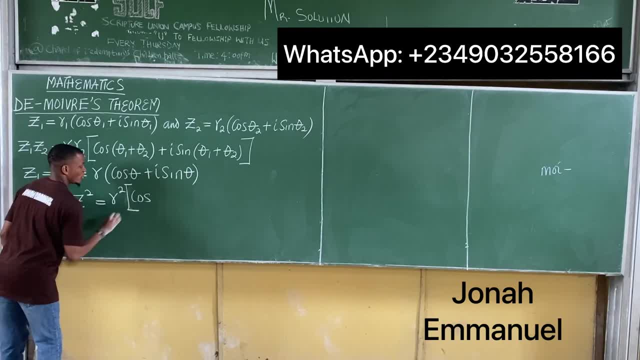 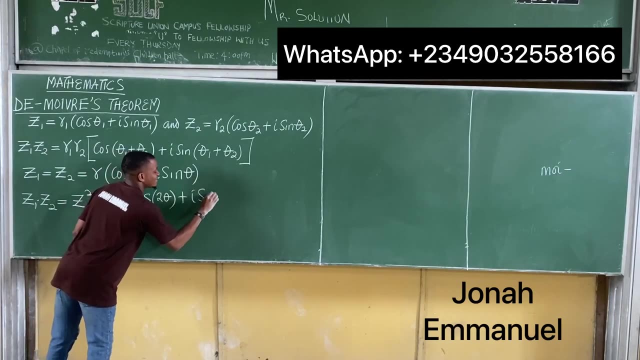 cos now I'll be having theta 1 plus theta 2, but theta 1 and theta 2 are the same thing. So it will be what there? Theta plus theta, that's 2, theta plus i sine- same thing here. 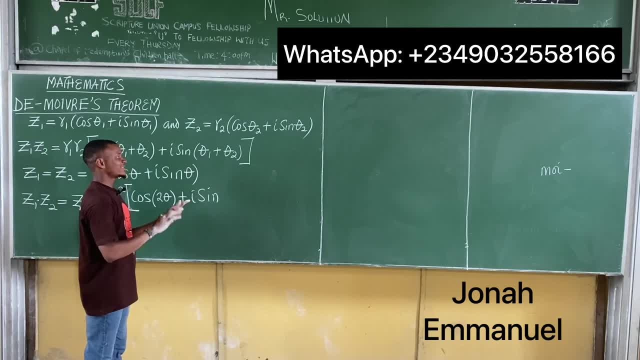 we are saying that theta and theta are the same thing, no longer theta 1 and theta 2.. So I'll be having theta plus theta. that will give you 2 theta, So I will have this one here. So please. we are saying that z1 and z2 are the same thing, So z1 times z2. 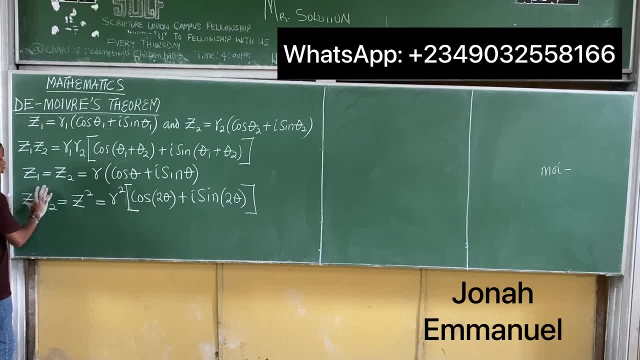 is a number multiplying itself. We want to call it as z, all squared, so I have this. So that will give me this one here. So it will be r1, r2, that's r times r, that's r squared into this one here. If you want, you can see the long multiplication, but I'm trying to save time. 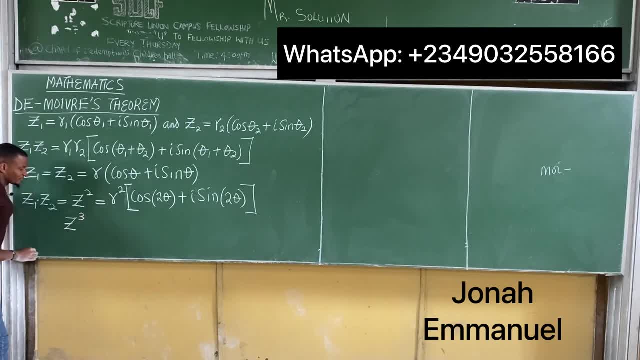 here. Let's use z cube. where will z cube be? Z cube will be equal to. of course, that will be r times r times r, that's r to power 3, into this will now be cos. if it's cubed, that means 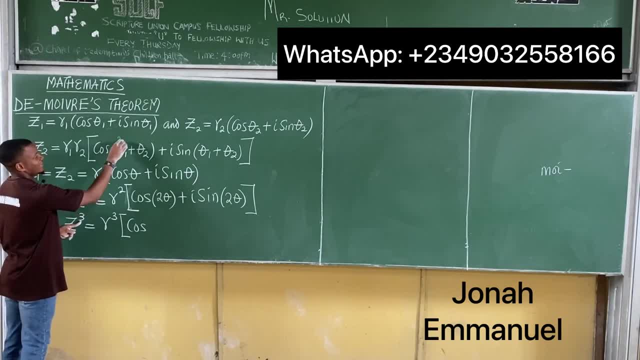 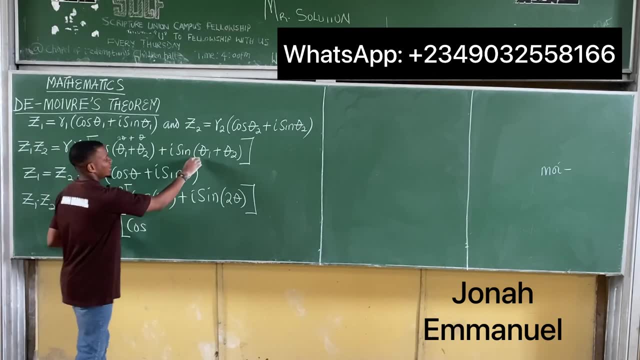 I'm having. in one side I'll have 2 theta. that's 2 theta in one side, plus in the other side I'll have another theta. alright, That will give me 3 of theta. Same thing here in one side I'll have. 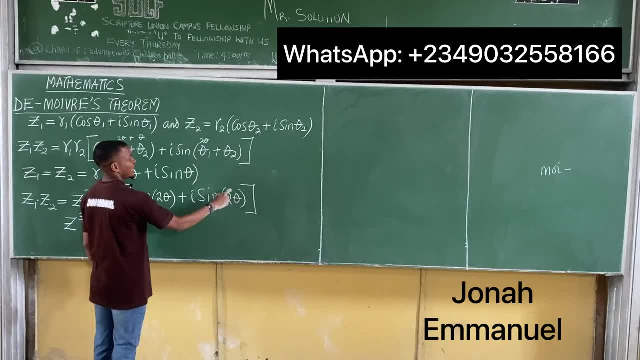 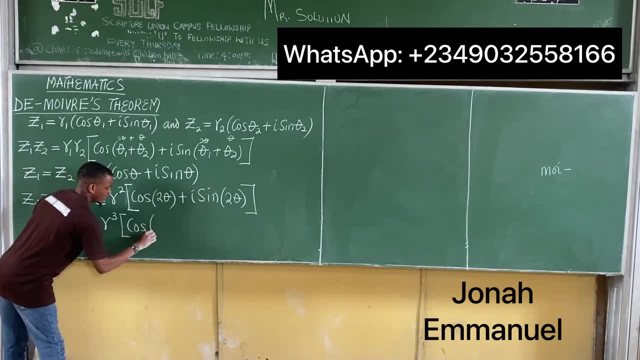 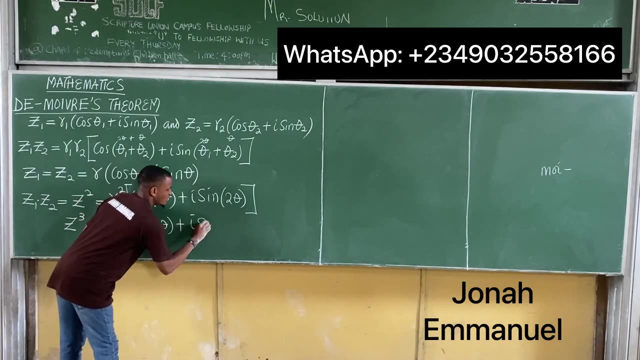 2 theta. as you can see here, 2 theta's from this and then another theta. that's the third one which I'm multiplying. So this will now give me something like 2 theta plus theta. gives you 3 theta plus i into sine. 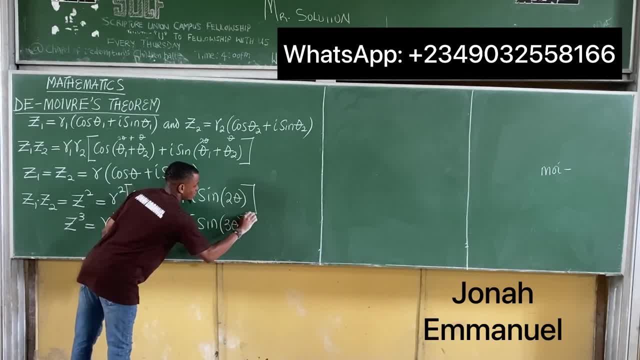 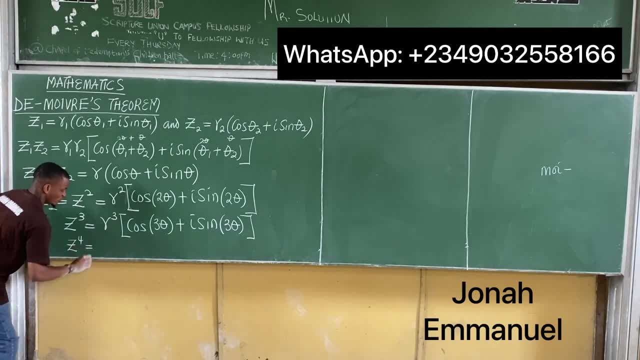 2 theta plus theta gives you 3 theta. So if you look at this progression perhaps you can guess the value of z to the power of 4.. z to the power of 4 will be equal to r to the power of 4, into cos. 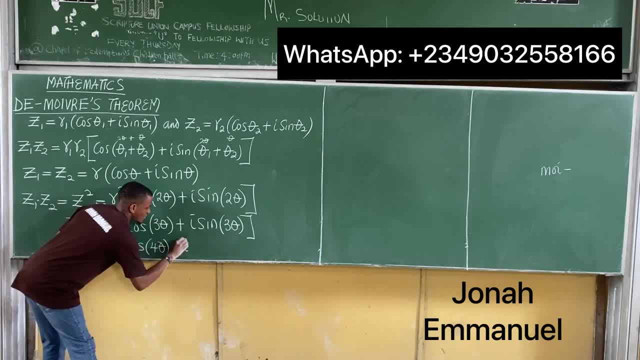 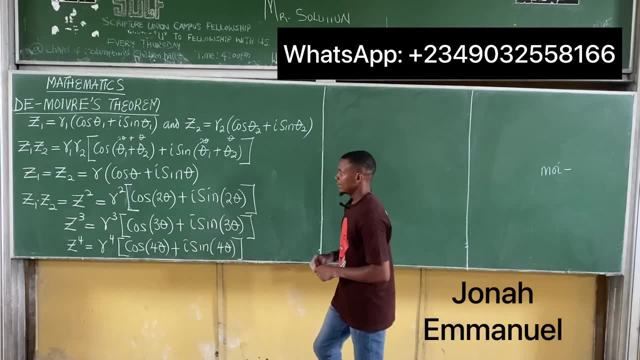 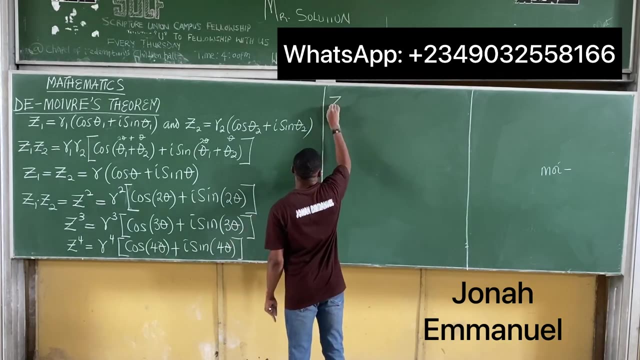 4 theta plus i sine 4 theta. So this is like the correlation of how this will work in this case. So if this is true, that means if the part there is n, I'll have that z to the power of n is equal to r. so when this 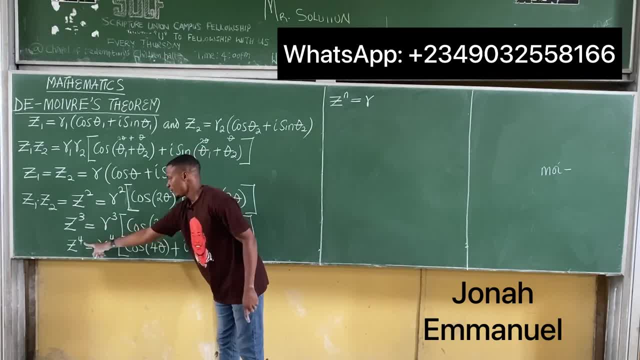 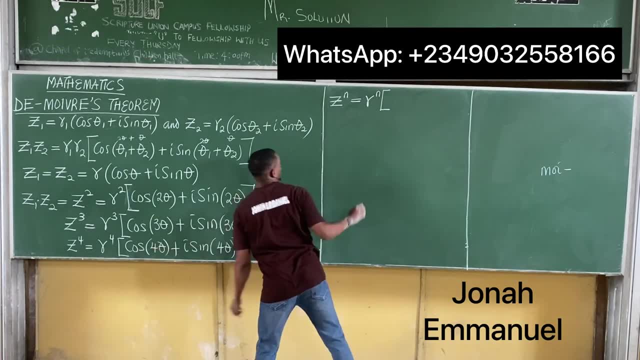 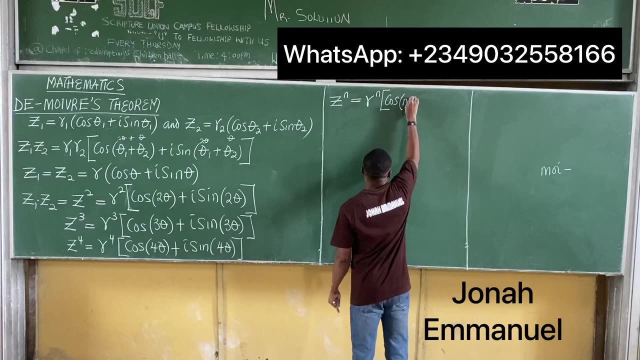 was 2, I had 2,, 3,, 3,, 4,, 4,. so when this is n, it becomes r to the power of n into cos of no longer 4 times theta. but we said this should be n, so it becomes n theta plus i sine n theta. 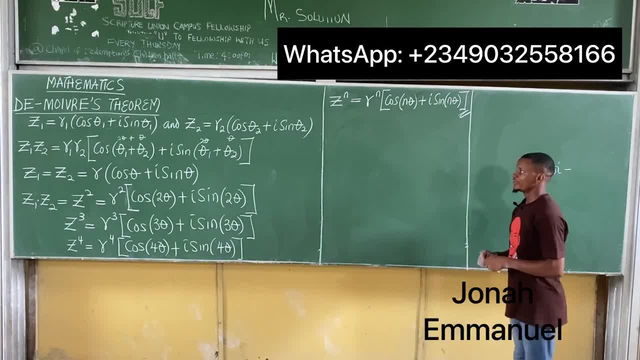 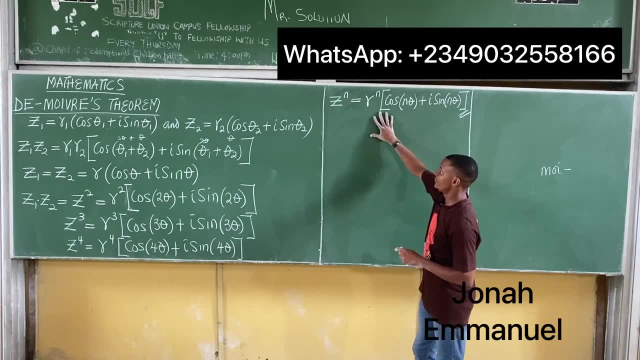 I would have this. So this is what is known as the Moivre's Theorem. The Moivre's Theorem will help us to do large expansion for complex numbers, Alright, so this is the Moivre's Theorem. This is the expression. 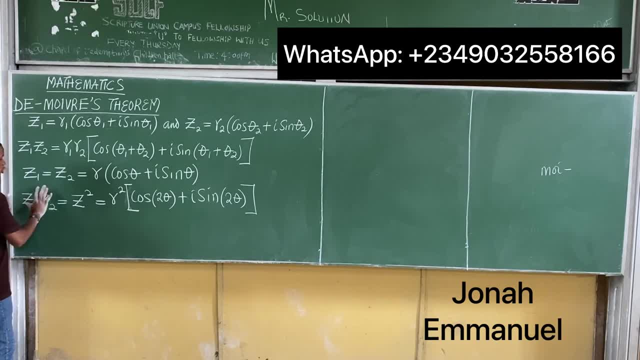 is a number multiplying itself. We want to call it as z, all squared, so I have this. So that will give me this one here. So it will be r1, r2, that's r times r, that's r squared into this one here. If you want, you can see the long multiplication, but I'm trying to save time. 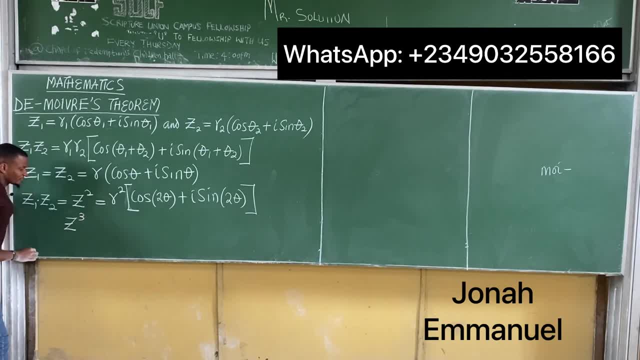 here. Let's use z cube. where will z cube be? Z cube will be equal to, of course. that will be r times r times r, that's r to the power 3, into this will now be cos. if it's cubed, that means I'm having in one side. I'll have 2 theta, that's 2 theta in one side. 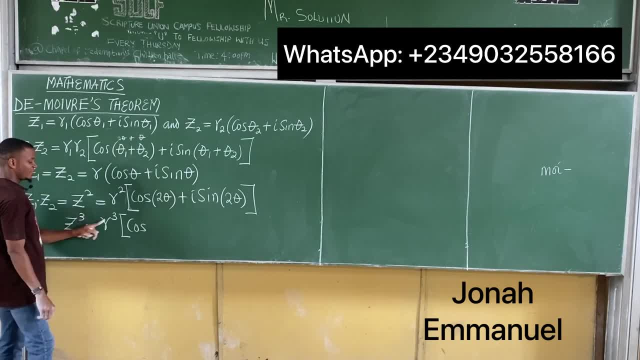 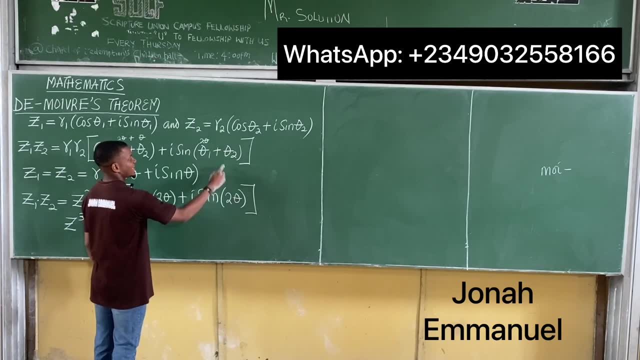 plus, in the other side I'll have another theta. alright, That will give me 3 of theta. Same thing here in one side. I'll have 2 theta, as you can see here: 2 theta's from this and then another theta. that's the third one which I'm multiplying. 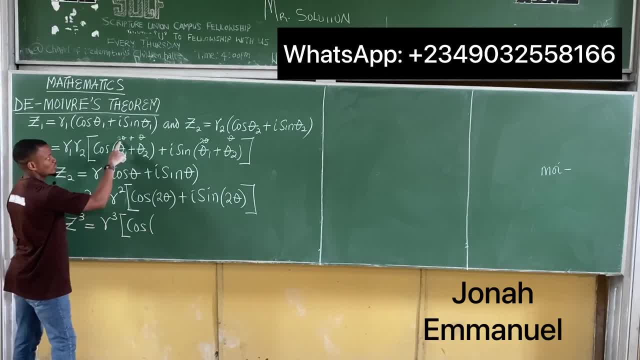 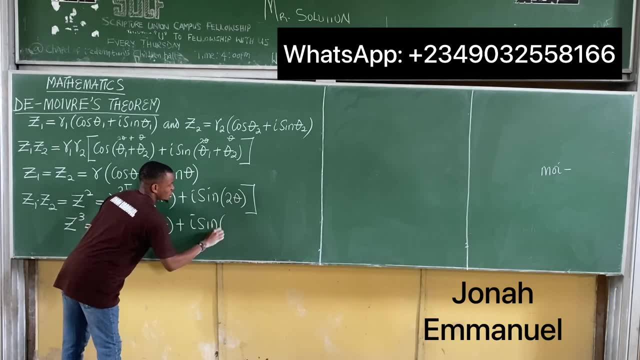 So I'll be having this. So this will now give me something like 2 theta plus theta gives you 3 theta plus i into sine: 2 theta plus theta gives you 3 theta. So if you look at this progression perhaps you can guess the value of z to the power 4.. 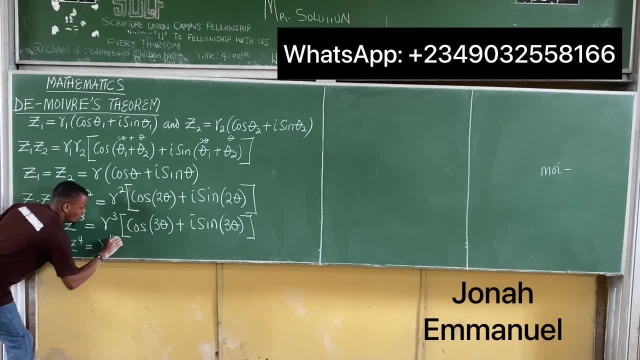 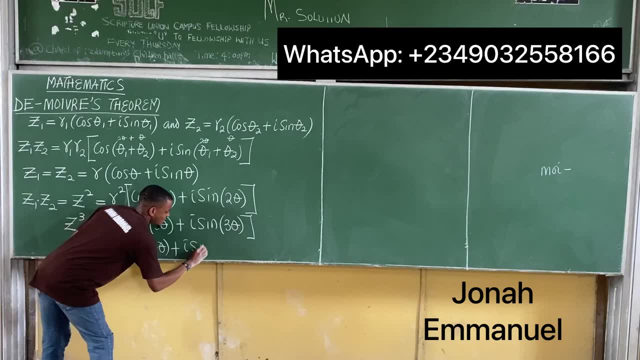 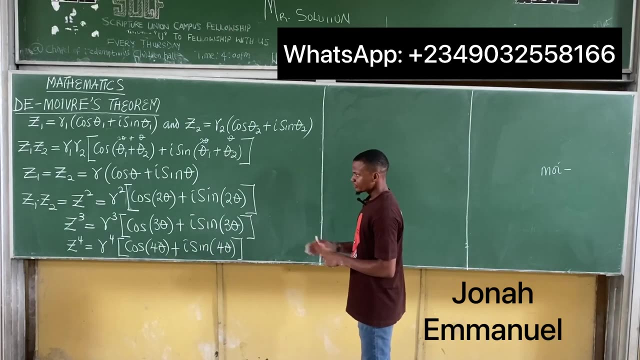 z to the power 4 will be equal to r to the power 4, into cos 4 theta plus i sine 4 theta. So this is like the correlation of how this will work in this case. So if this is true, that means 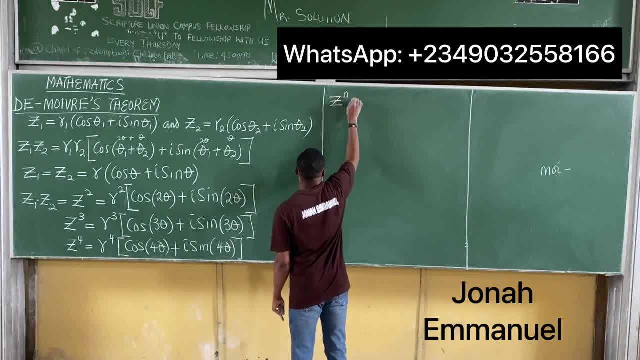 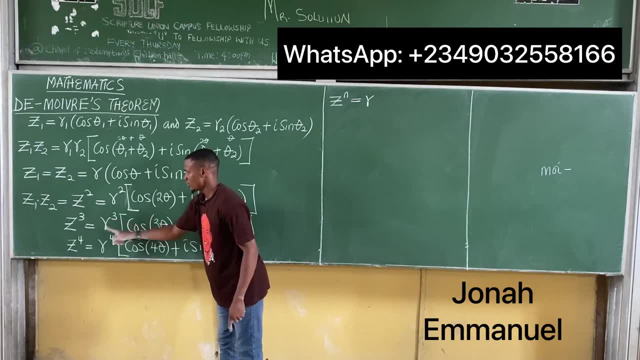 if the part there is n, I'll have that z to the power n is equal to r. so when this was 2,, I had 2,, 3,, 3,, 4,, 4, so when this is n, it becomes r to the power n. 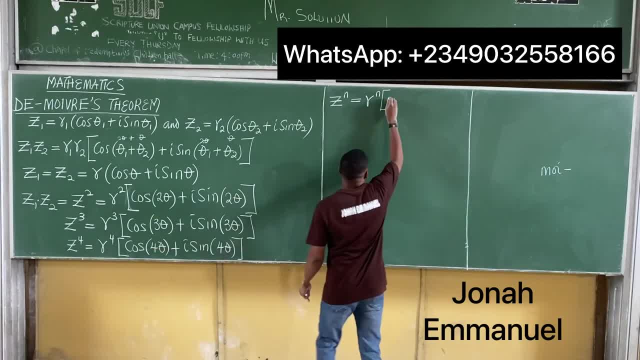 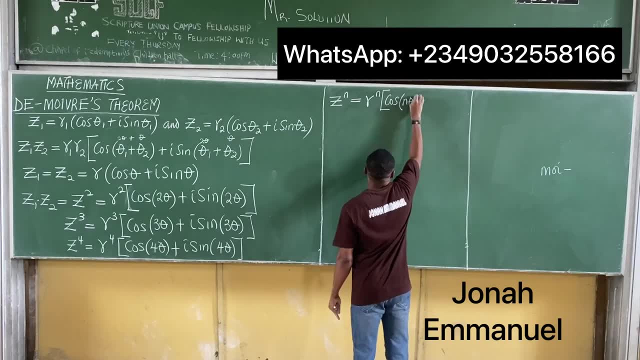 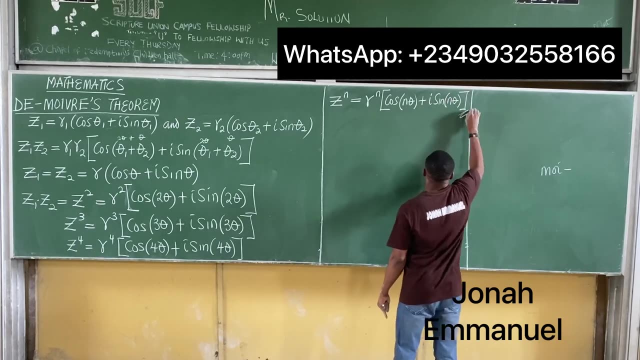 into cos of no longer 4 times theta. but we say this should be n. it becomes n theta plus i sine n theta. I'll have this. So this is what is known as the Moivre's theorem. The Moivre's theorem has helped us do large expansion for complex numbers. 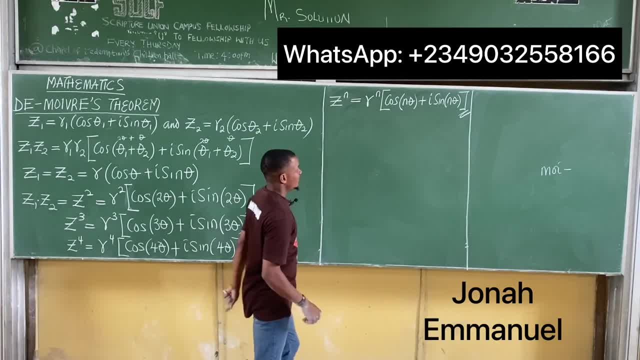 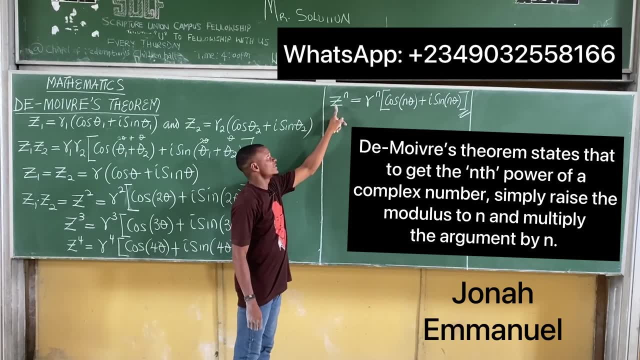 Alright, so this is the Moivre's theorem. This is the expression In words. the Moivre's theorem says: to take the nth power of a complex number, the nth power of a complex number. to take the nth power of a complex number. 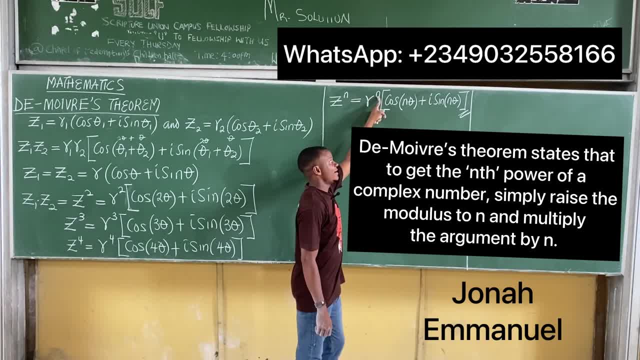 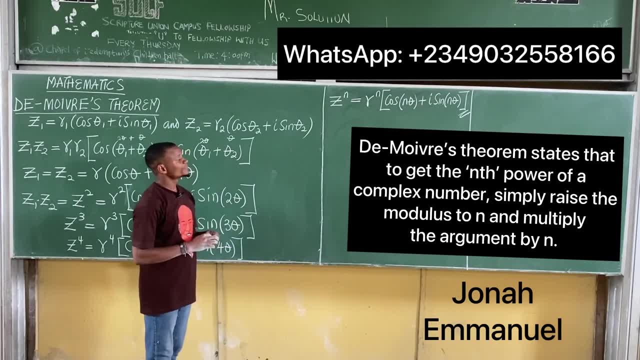 simply raise the modulus to power n and multiply the argument by n. That's all. So that's what the Morbius theorem states. It states that to raise or to find the nth power of a complex number, simply raise the modulus to n. 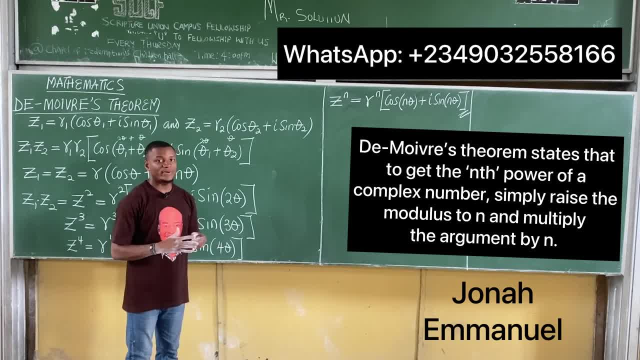 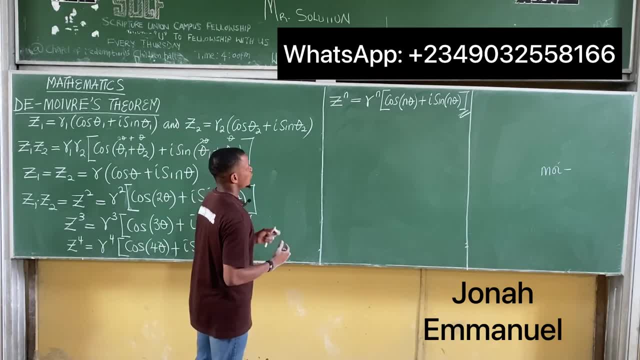 and, of course, multiply the argument or the amplitude by n. That's the statement of the Morbius theorem. All right, so, having said that, what does this help us to do? Now we'll take an instance. Let's say z is equal to. 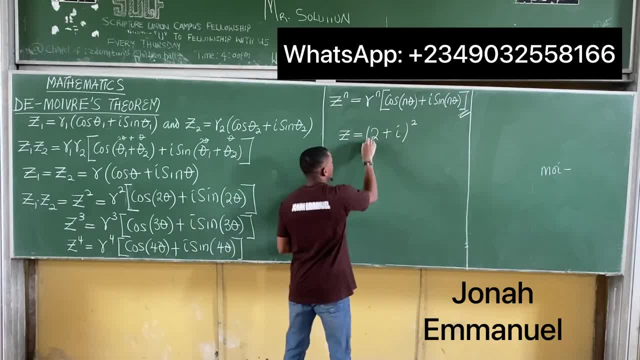 2 plus i to power 2.. This would be easy to solve because I simply multiply this as 2 plus i, multiplying 2 plus i. That's easy to do. But what if I change this to 35,, for instance? 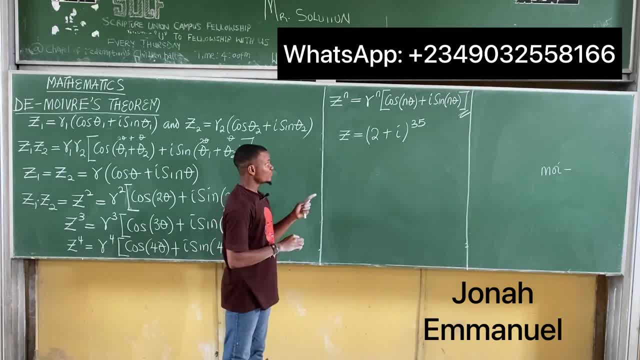 So z is equal to 2 plus i to power 35. Now this would be multiplying 2 plus i, multiplied by 2 plus i, multiplied by 2 plus 5, up to 35 places, And that's way too long. 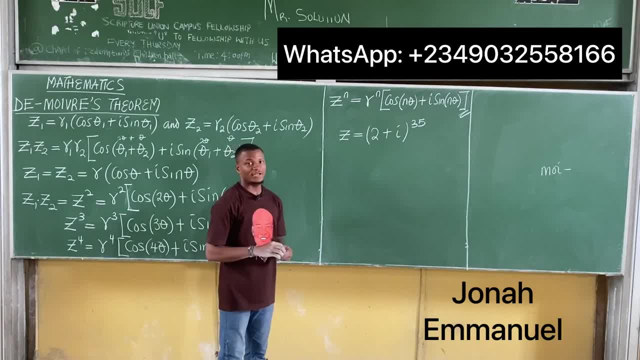 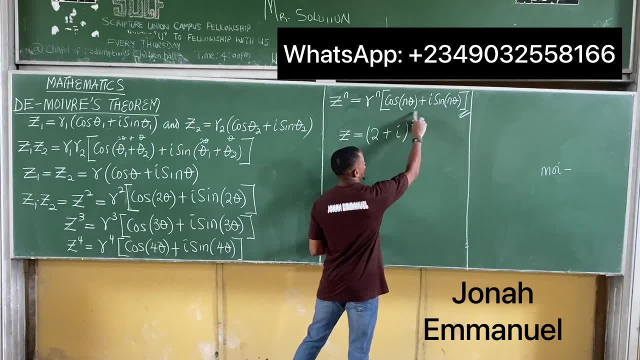 and tasky to do So. in this case, now employ the Morbius theorem, And that's why the Morbius theorem is very, very important. It helps us to do, or it helps to take, the nth power of a complex number in an easy way. 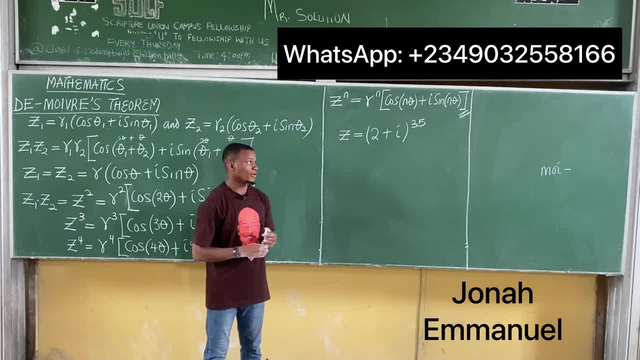 So this is why the Morbius theorem is very, very important. All right, so, having said this, let's see how we can take the. let's see how the Morbius theorem can actually help us in doing some calculations. 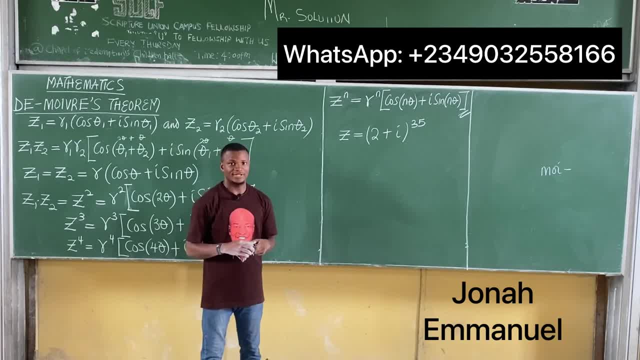 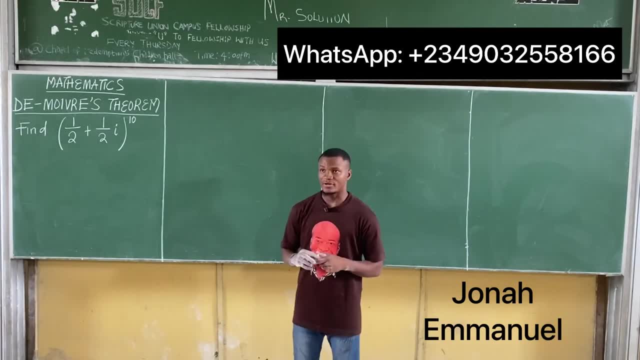 So we'll take some examples and work with the Morbius theorem. All right, so let's look at an example on the Morbius theorem and how it helps us to solve problems pertaining to the nth power of a complex number. So let's say we're given 1 plus 2,. 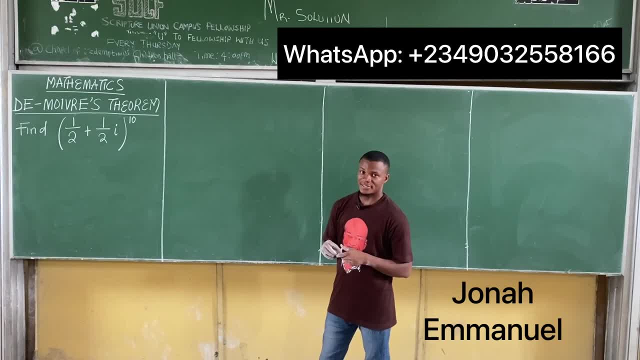 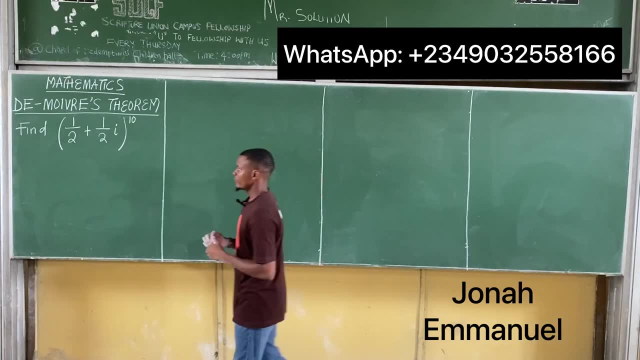 that's half plus half. i. We're asked to find the 10th power of this. Of course, having to expand this 10 times can be very cumbersome, So we'll have to use the Morbius theorem From the Morbius theorem. 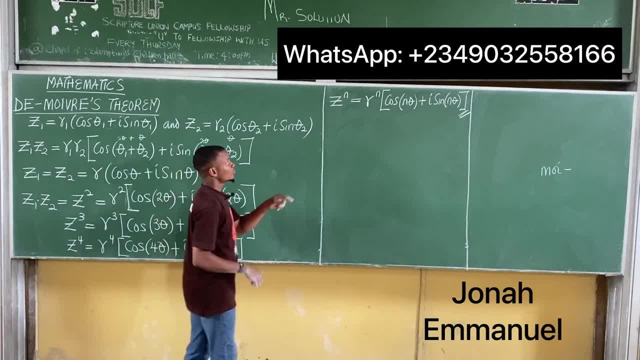 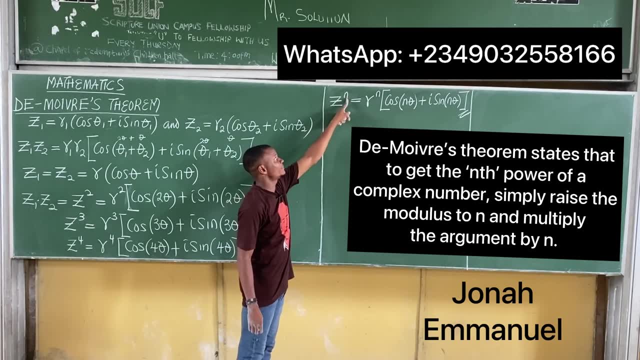 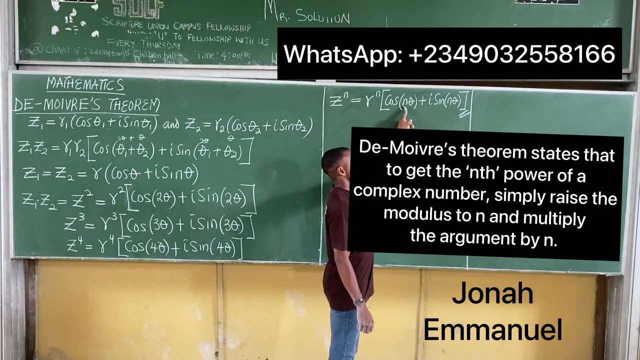 In words, the Moivre's Theorem says: to take the nth power of a complex number, the nth power of a complex number. to take the nth power of a complex number, simply raise the modulus to power n and multiply the argument by n. 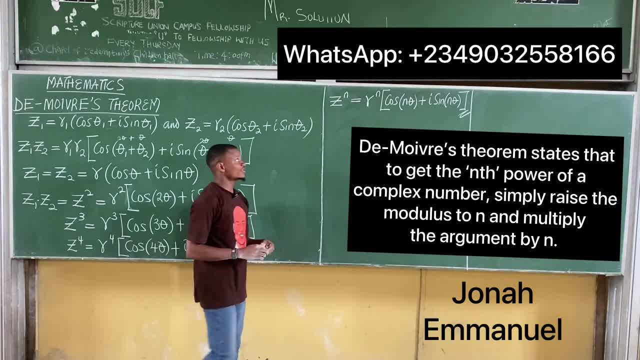 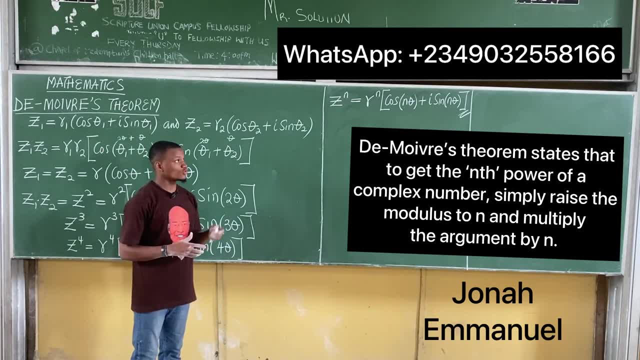 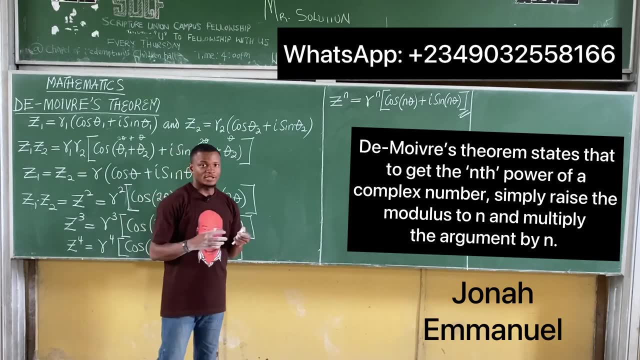 That's all. So that's what the Morbius theorem states. It states that to raise or to find the nth power of a complex number, simply raise the modulus to n and, of course, multiply the argument or the amplitude by n. That's the statement of the Morbius theorem. 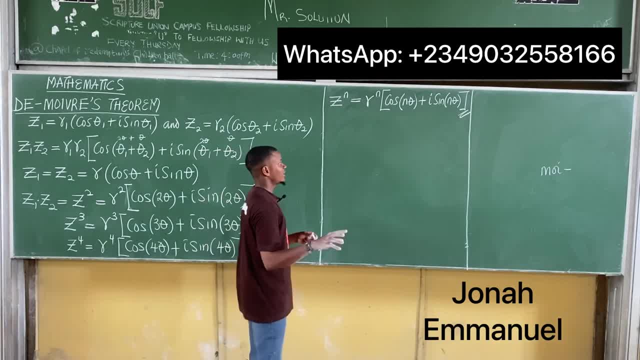 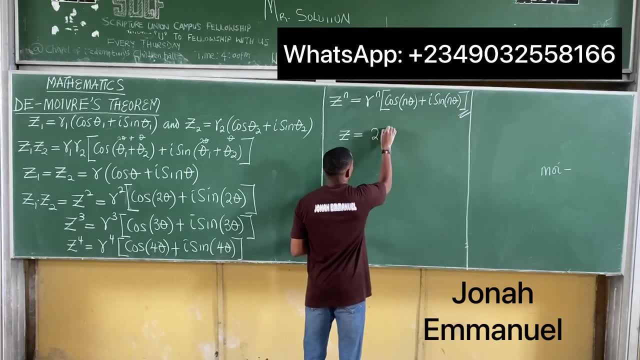 Alright. so, having said that, what does this help us to do Now? we'll take an instance. Let's say z is equal to 2 plus i to power 2.. This would be easy to solve, because I simply multiply this as 2 plus i, multiplying 2 plus. 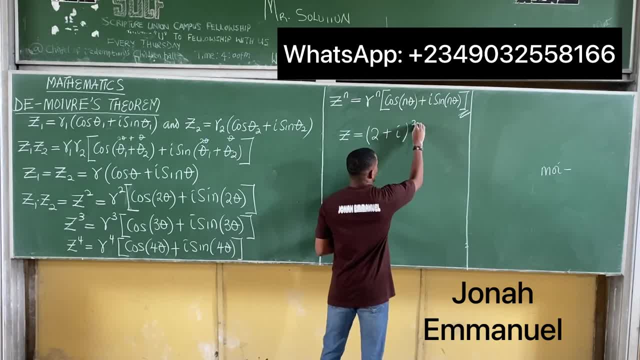 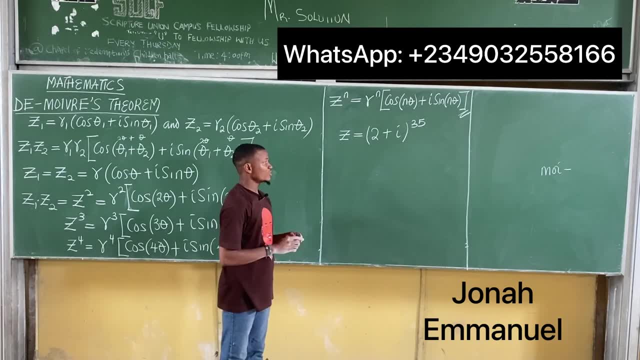 i. That's easy to do. But what if I change this to 35, for instance? So z is equal to 2 plus i to power 35. Now this would be multiplying 2 plus i, multiply by 2 plus i multiply by 2 plus 5, up to 35. 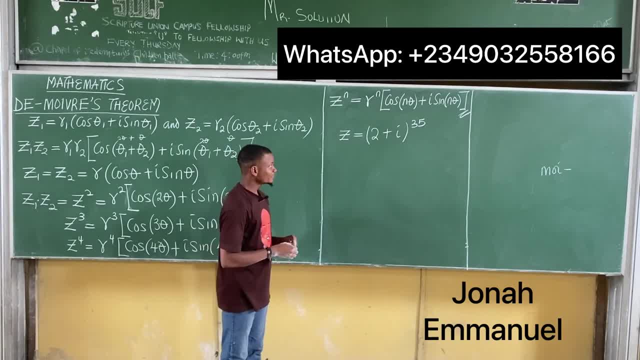 places And that's way too long and tasky to do So in this case, now employ the Morbius theorem, And that's why the Morbius theorem is very, very important. It helps us do, or it helps to take the nth power of a complex number in an easy way. 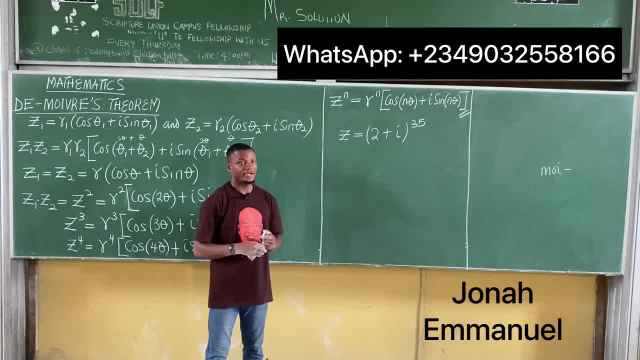 So this is why the Morbius theorem is. It's very, very important, Alright. so, having said this, let's see how we can take the. Let's see how the Morbius theorem can actually help us in doing some calculations. 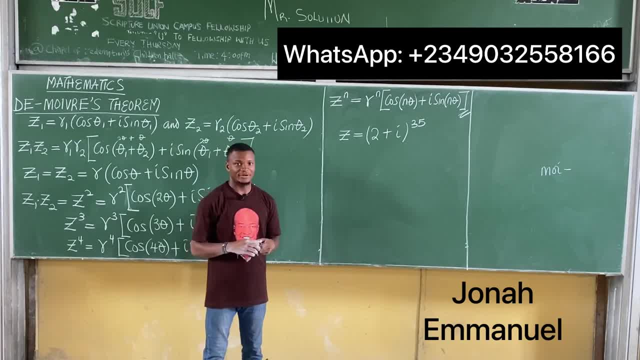 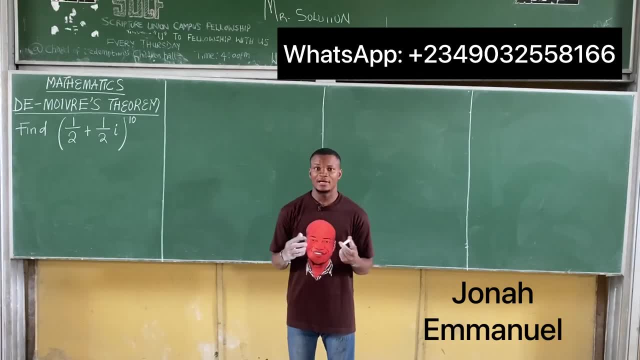 So we'll take some examples and work with the Morbius theorem. Alright, so let's look at an example on the Morbius theorem and how it helps us to solve problems pertaining to the nth power of a complex number. So let's say we're given 1 plus 2, that's half plus half i. 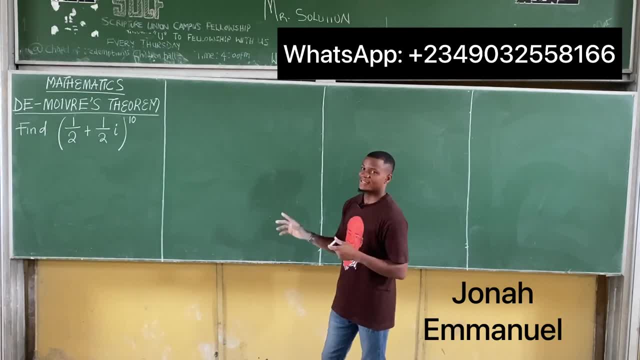 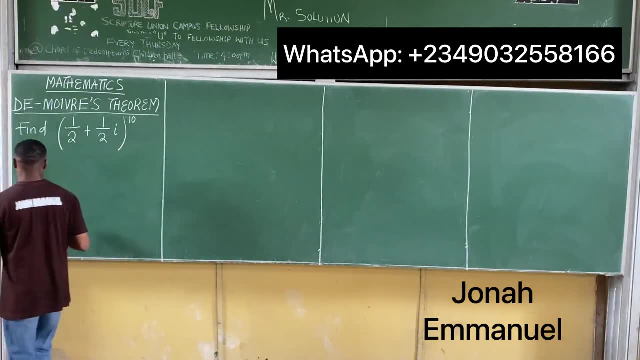 We're asked to find the tenth power of this. Of course, having to expand this ten times can be very cumbersome, so we'd have to use the Morbius theorem. From the Morbius theorem we said z to power n, a particular complex number to power n. 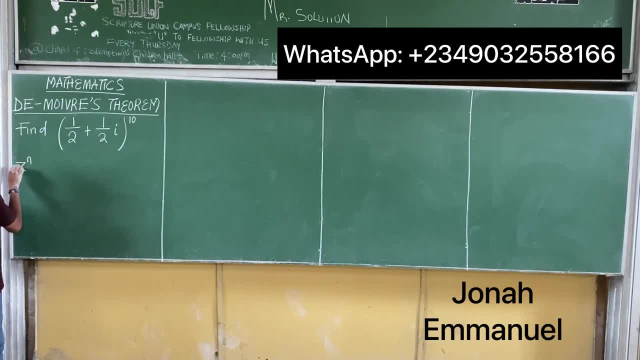 we said z to the power n. a particular complex number to the power n is equal to r to the power n into cosine of n theta plus i sine n theta. We said this: All right. so if this is true, let's get n. 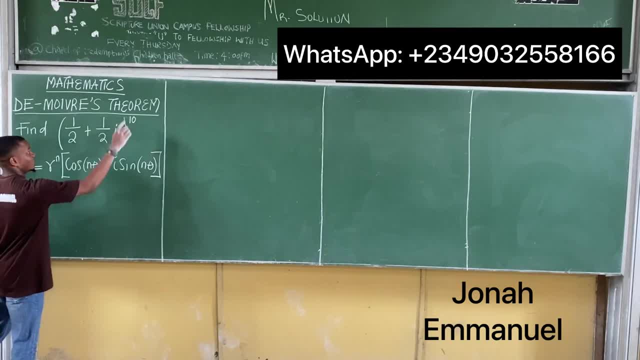 Of course, from here n is equal to the power, that's 10.. Let's get r, So r will be equal to the modulus square root of this, so square root of 1 over 2 r squared, plus 1 over 2 r squared. 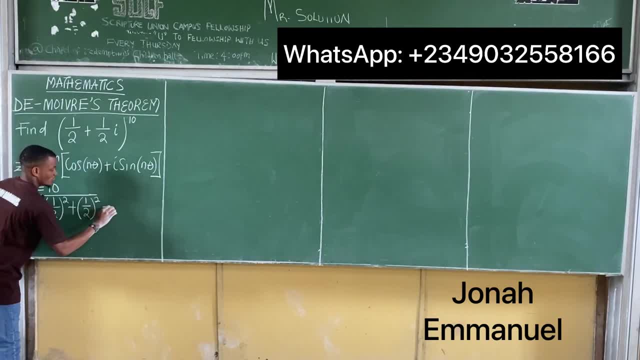 So d squared plus d squared, So that will be equal to square root of 1 over 2. squared is 1 over 4 plus 1 over 2 squared r squared is 1 over 4.. That means r is equal to. 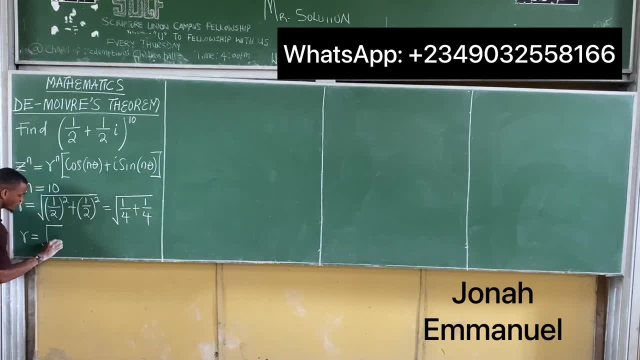 square root of same denominator, so 4.. I will simply add up the powers. that's 2.. So 1 plus 1 gives me 2.. So if you do 1 over 4 plus 1 over 4, you have 2 over 4,. 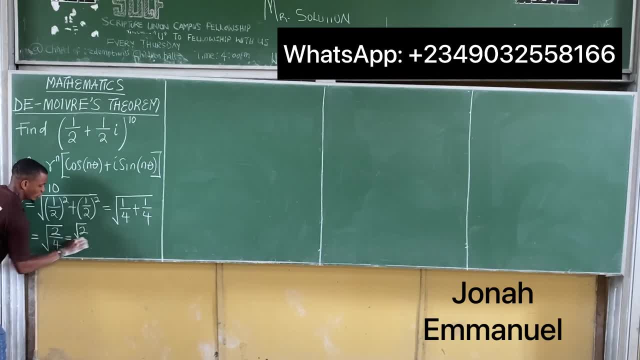 and that's equal to. in short form, this is root 2 all over, this is root 4, and that's equal to root 2, all over. root 4 is 2.. So r is equal to root 2 over 2.. 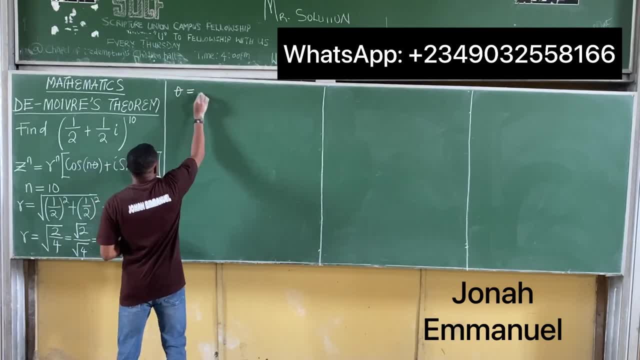 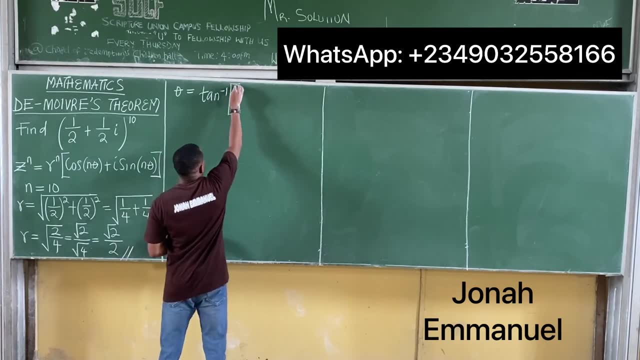 Next up, let's find the angle. Theta is equal to the tan inverse, so tan inverse of b over a and tan inverse of b is 1 over 2.. That's this all over a, also 1 over 2,. 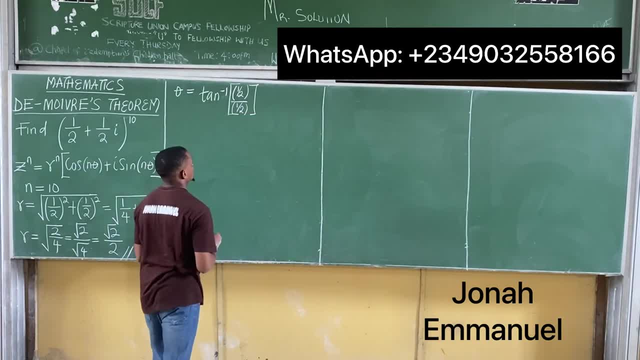 1 all over 2.. I have this tan inverse of b over a and that's equal to. of course this can cancel this. That's mathematically correct. I have 1 over 1, so that means theta is equal to. 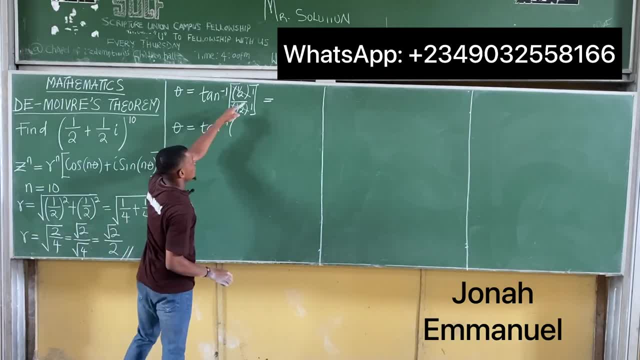 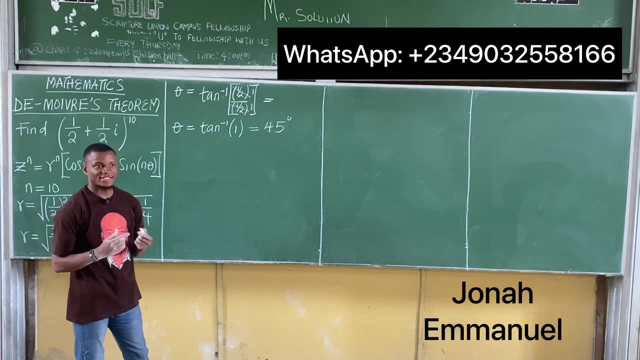 tan inverse of 1 over 1 gives you 1.. Tan inverse of 1 is equal to 45 degrees. so we have this one here. We've worked so much with degrees. How about we work with radians? that's pi. 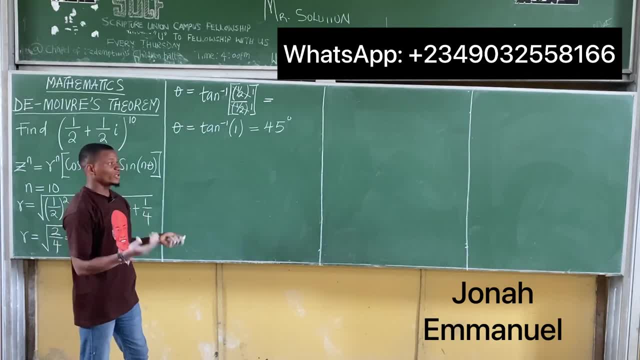 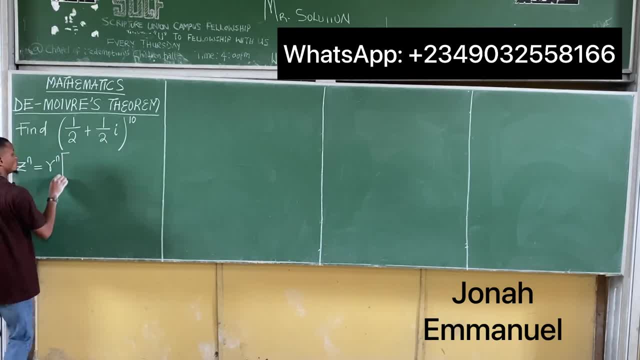 is equal to r to power, n into cosine of n theta plus i sine n theta. we said this Alright. so if this is true, let's get n Of course from here. n is equal to the power, that's 10.. 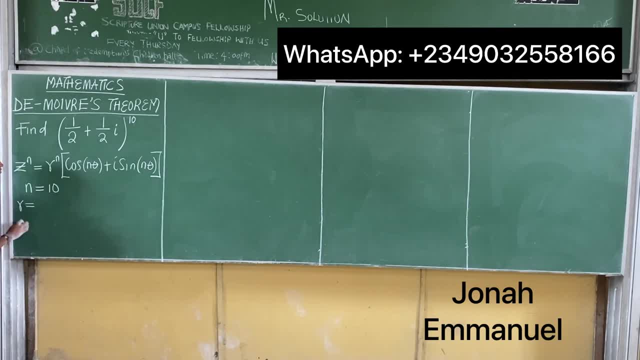 Let's get r. So r will be equal to the modulus square root of this, so square root of 1 over 2 r squared plus 1 over 2 r squared. So d squared plus d squared, So that will be equal to square root of. 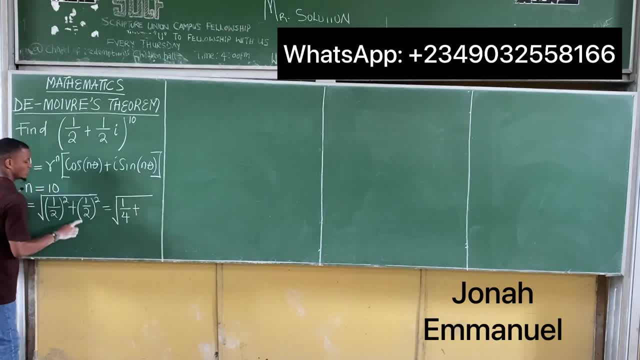 1 over 2 squared is 1 over 2.. 1 over 4 plus 1 over 2 squared r squared is 1 over 4.. That means r is equal to square root of same denominator, so 4.. I'll simply add up the parts. that's 2.. 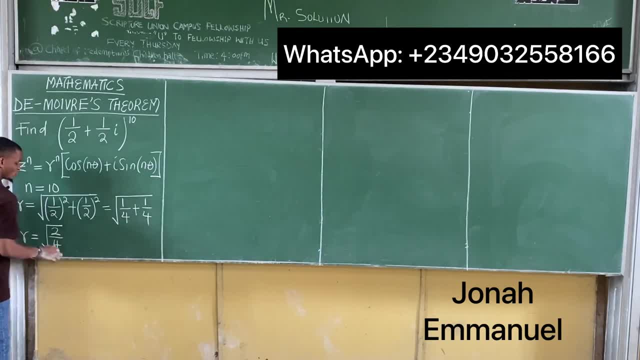 So 1 plus 1 gives me 2.. So if you do 1 over 4 plus 1 over 4, you have 2 over 4, and that's equal to, in short form: this is root 2 all over. this is root 4, and that's equal to root 2 all over. 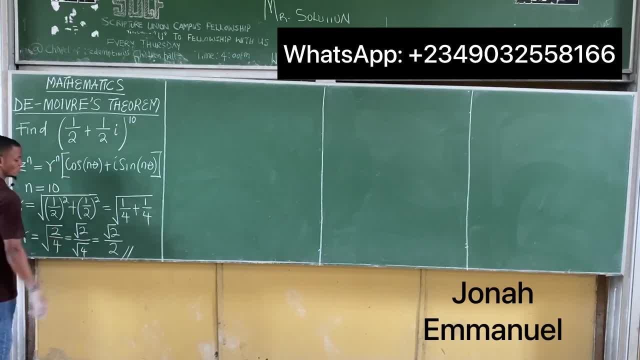 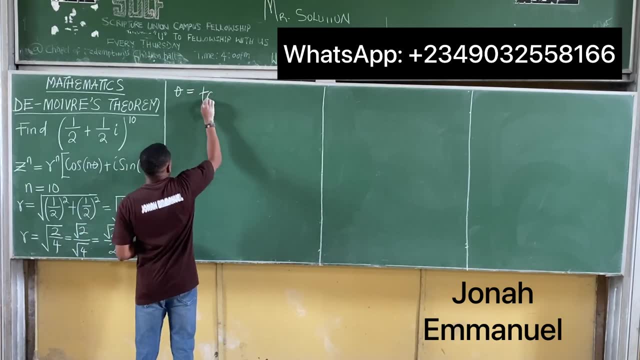 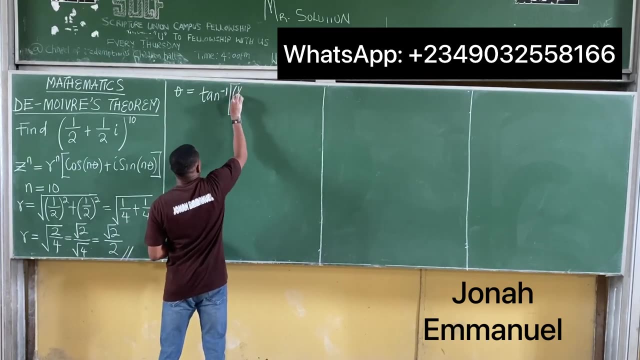 root 4 is 2.. So r is equal to root 2 over 2.. Next up, let's find the angle. theta is equal to the tan inverse, So tan inverse of b over a and tan inverse of b is 1 over 2.. 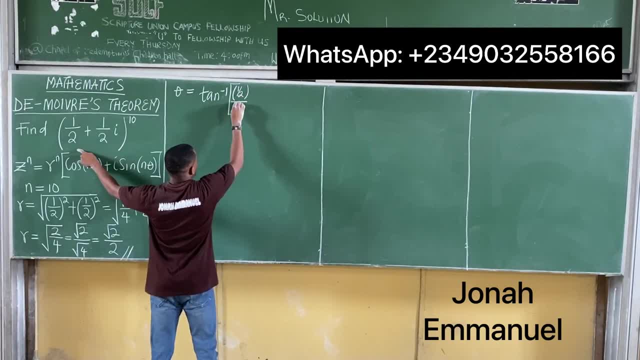 That's this all over a, also 1 over 2, 1 all over 2.. I have this tan inverse of b over a and that's equal to. Of course, this can Cancel this. That's mathematically correct. 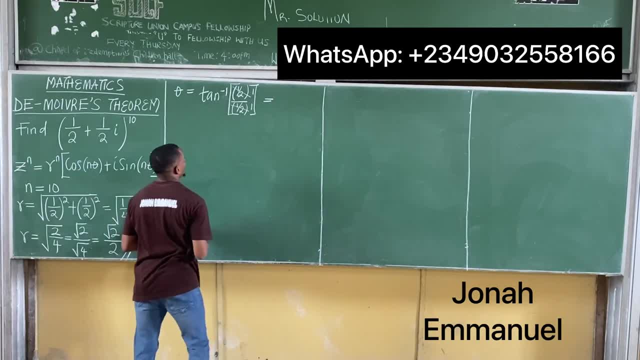 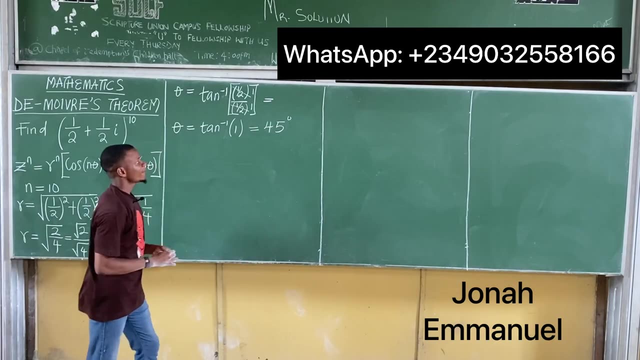 I have 1 over 1, so that means theta is equal to tan inverse of 1 over 1 gives you 1.. Tan inverse of 1 is equal to 45 degrees. so we have this one here. We've worked so much with degrees. 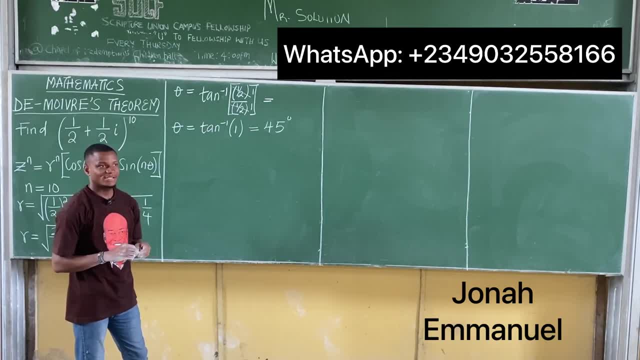 How about we work with radians? that's pi. All right. so let's just work with pi for this. We'll see what happens. We'll work with degrees much more later, but we've worked so much with degrees for this, So let's try pi. 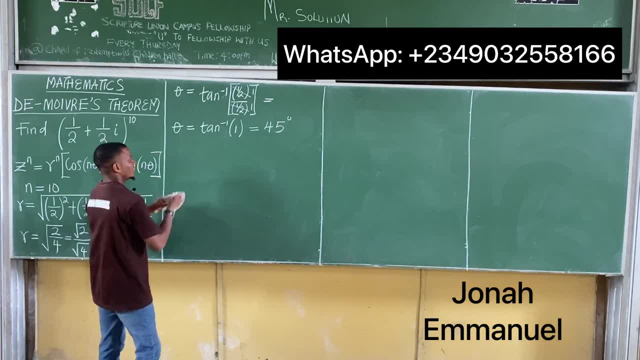 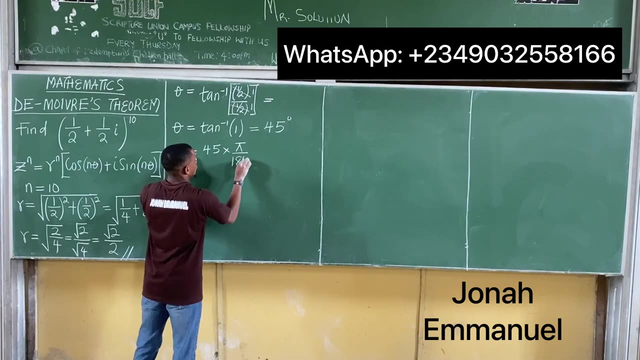 with degrees. for this, Let's try pi. Theta will be equal. to convert this to pi. What will it be? We said the value, the angle will be equal to 45 times pi, all over 180.. To convert from. to convert from degrees. 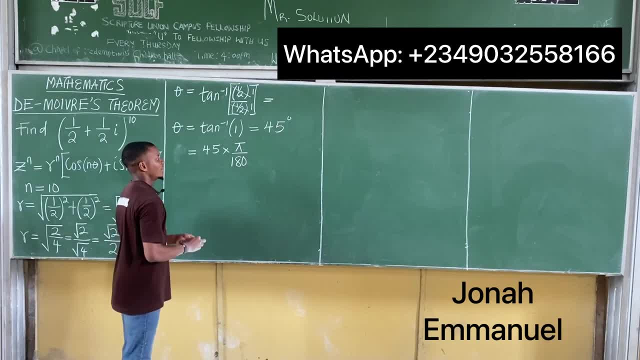 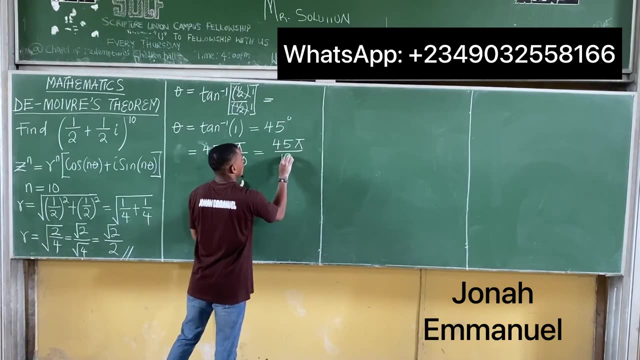 to pi. simply multiply the value by pi. Pi over 180. So that's equal to 45 here. So this is equal to before this. 45 times pi is 45 pi all over 180.. That means the theta in this angle. 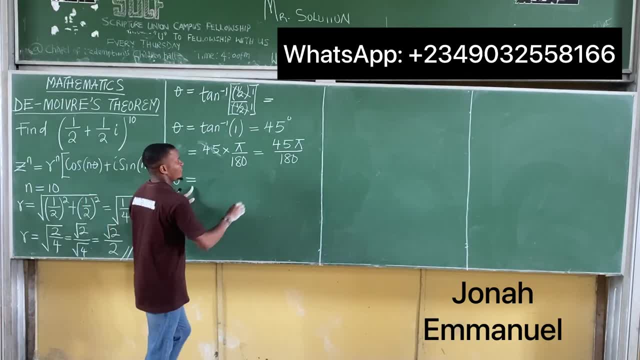 the angle here. theta is equal to 45 here, 1. 45 here that should be. that should give you about 4 times of it. That should be equal to pi over 4.. That should be equal to pi over 4.. 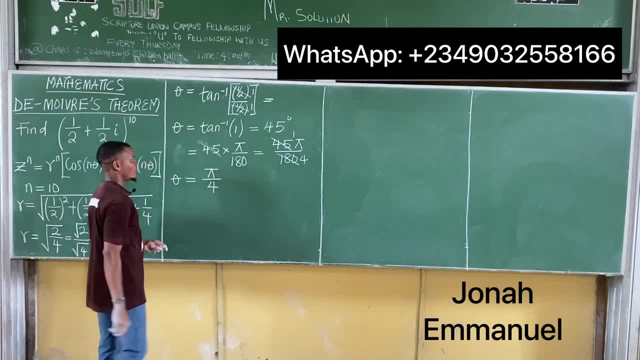 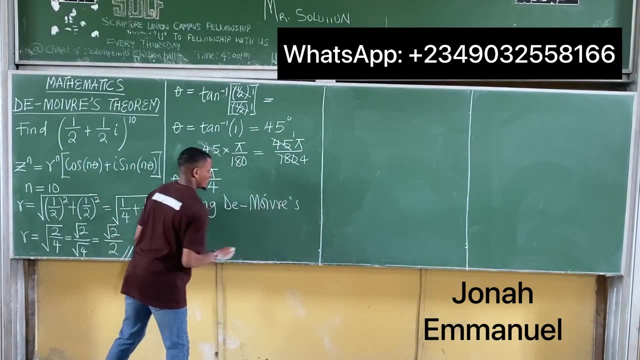 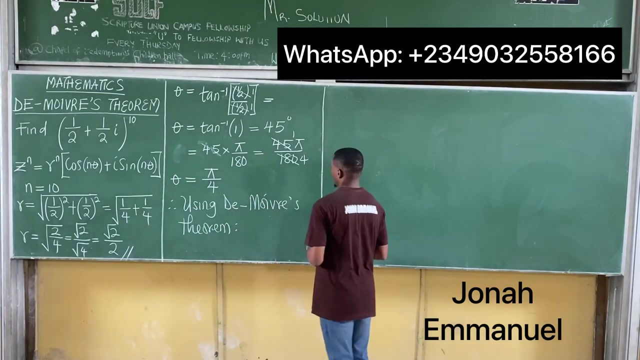 So theta is equal to pi all over 4.. So that's my theta, the angle. So hence using, therefore using the Moivre's theorem, the Moivre's theorem, what do we have? Alright, we have that 1 over 2 plus. 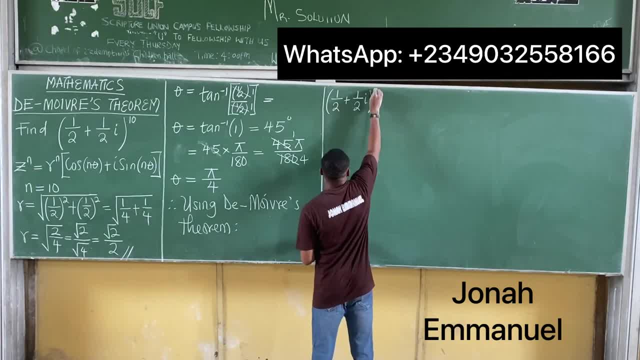 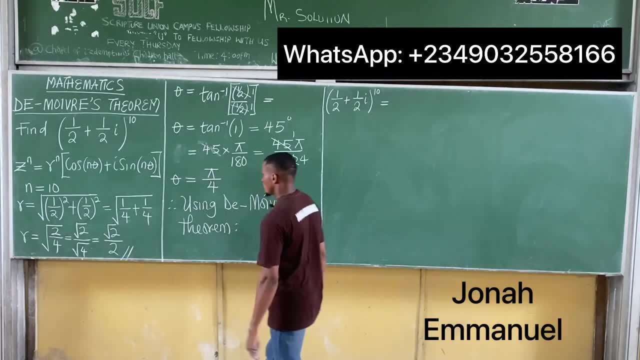 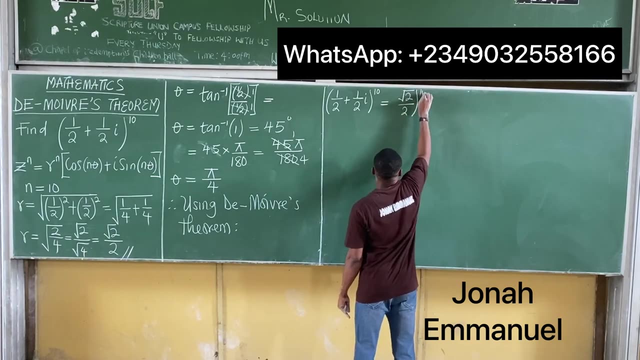 1 over 2i to the power 10 will be equal to r. where's r again This? So 2, that'll give you root 2 all over 2, that's r to the power 10.. Okay. 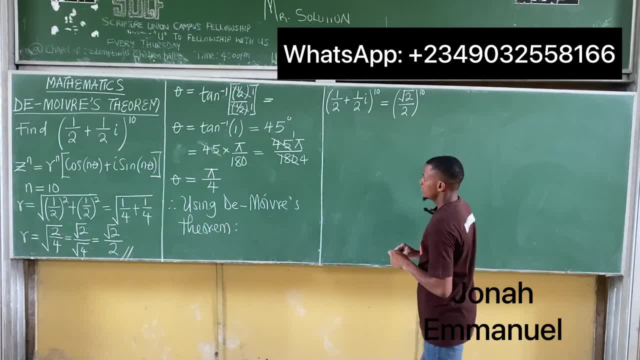 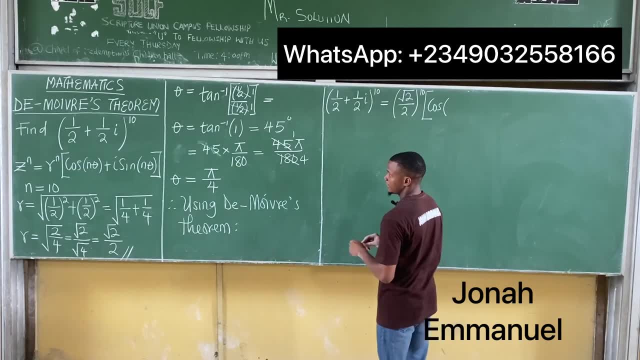 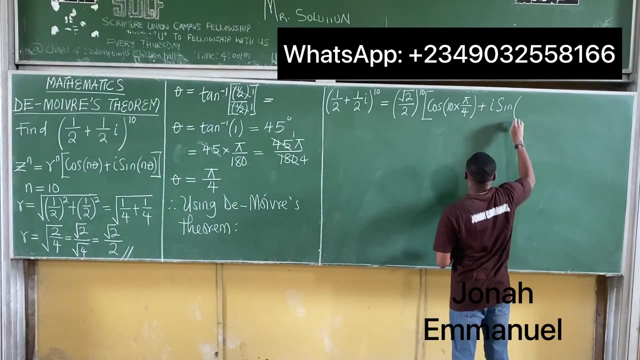 Next up. I said into cos, so into cosine of n. n is 10 there, so 10 times theta. we're using the radian's form, that's pi over 4 plus i sine n. n there is 10, so 10. 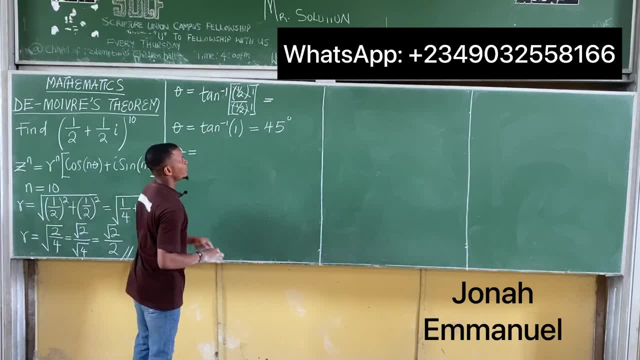 Theta will be equal. to Convert this to pi, What will it be? We said the value. the angle will be equal to 45 times pi, all over 180.. To convert from, To convert from degrees to pi, simply multiply the value by pi over 180.. 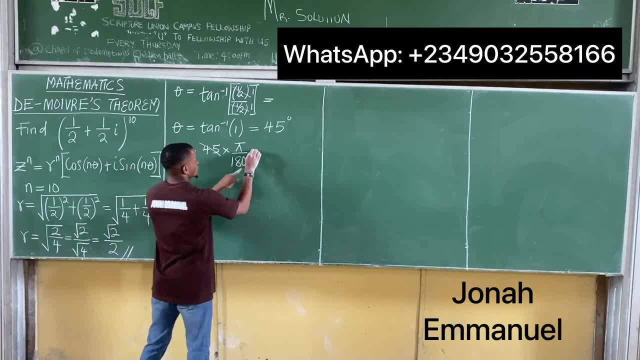 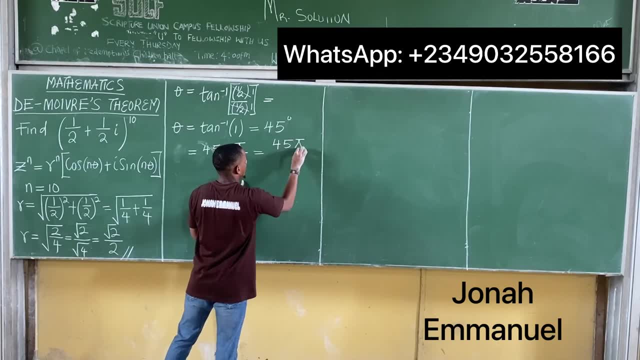 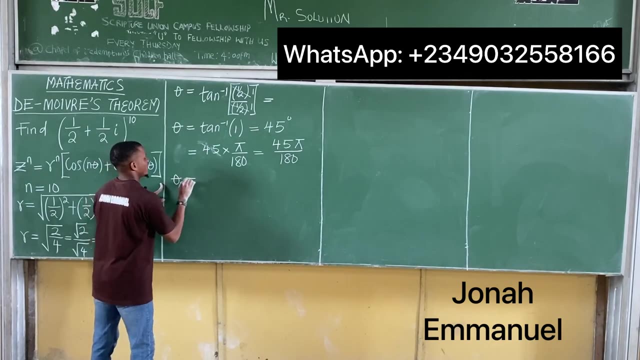 So that's equal to 45 here. So this is equal to Before. this. 45 times pi is 45, pi all over 180.. That means the theta in this angle, the angle here, theta is equal to 45, here 1,, 45 here. 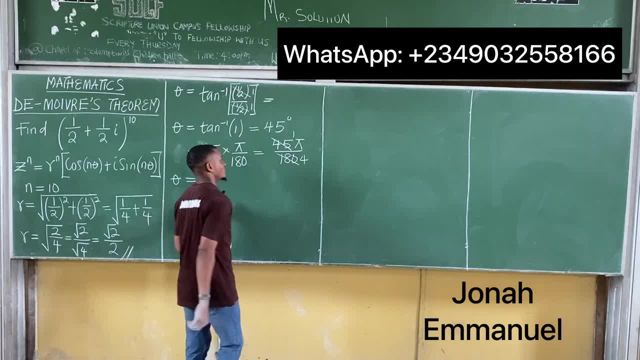 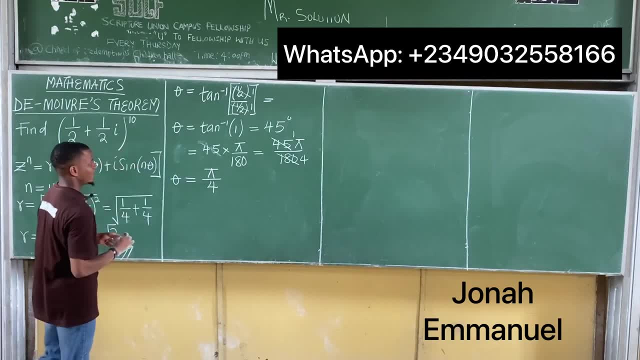 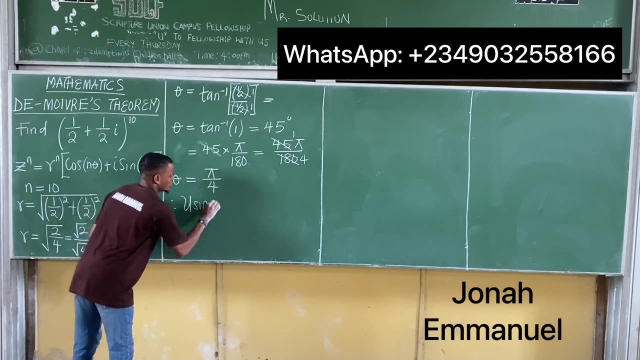 that should give you about 4 times of it. That should be equal to pi over 4.. So theta is equal to pi over 4.. Pi over 4.. So that's my theta, the angle, So, hence using, therefore using the Moivre theorem. 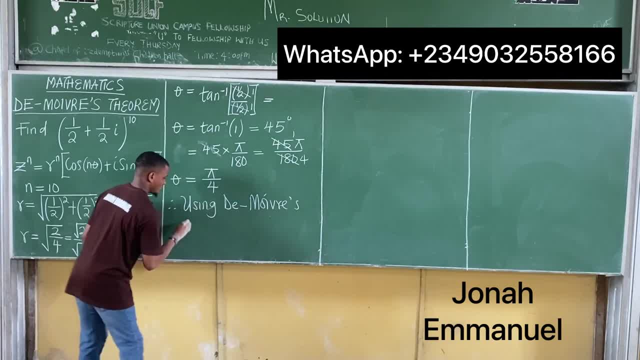 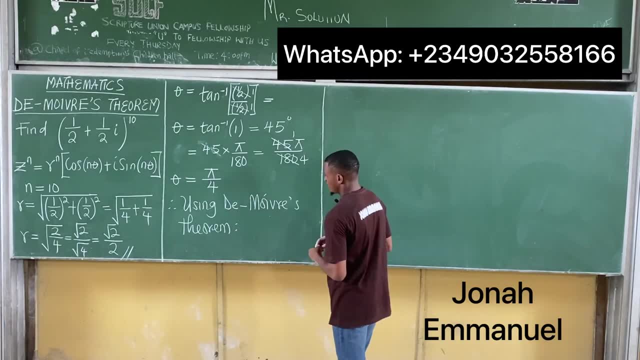 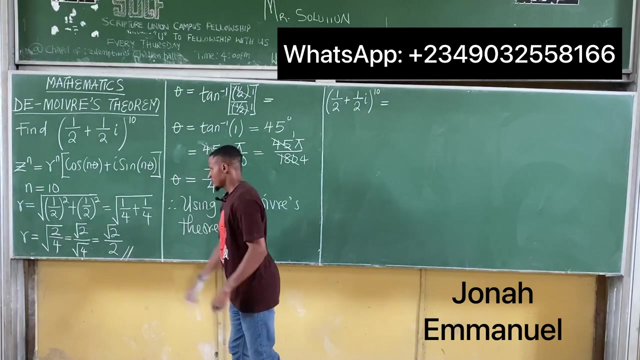 the Moivre theorem. what do we have? All right, we have that 1 over 2 plus 1 over 2.. 2i to the power 10 will be equal to r. Where's r again This? So root 2, I'll give you root 2 all over 2.. 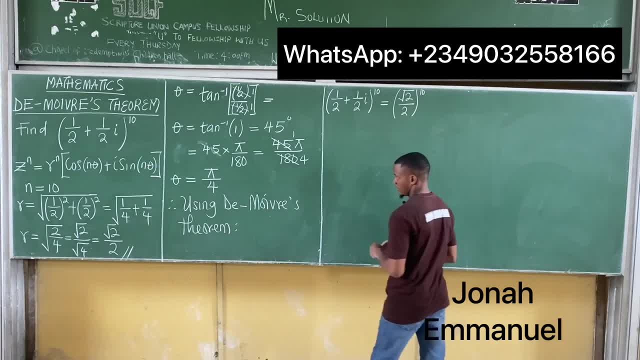 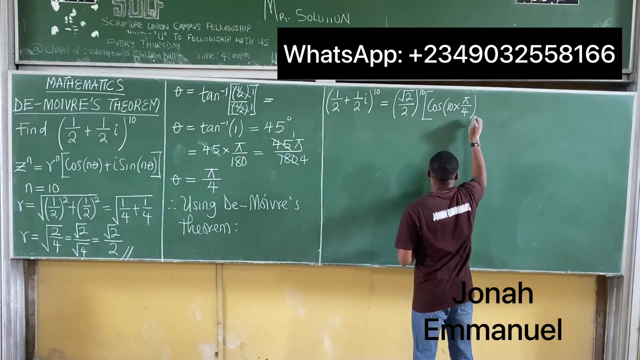 That's r to the power 10.. Okay, Next up, I said into cos, So into cosine of n. n is 10 there, So 10 times theta. we're using the radians form, That's pi over 4 plus i sine n. 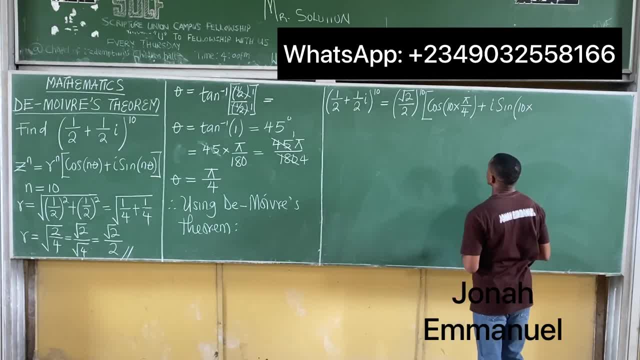 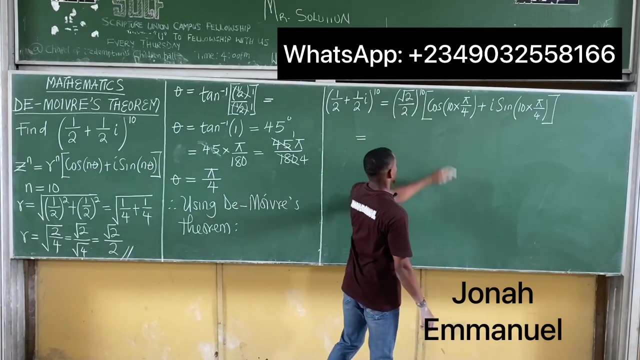 n, there is 10.. So 10 times theta, which we got here as pi over 4.. So I have this Alright. So this is equal to. This is equal to. So let's see if we can simplify this in the calculator. 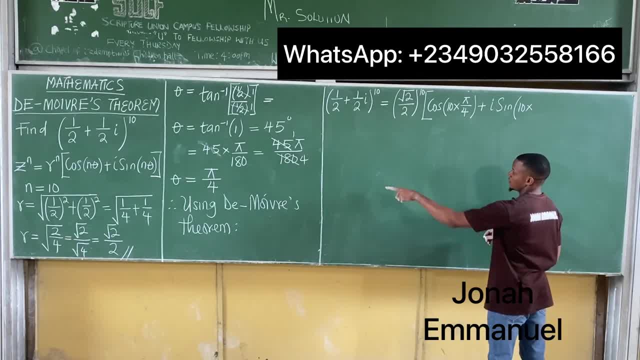 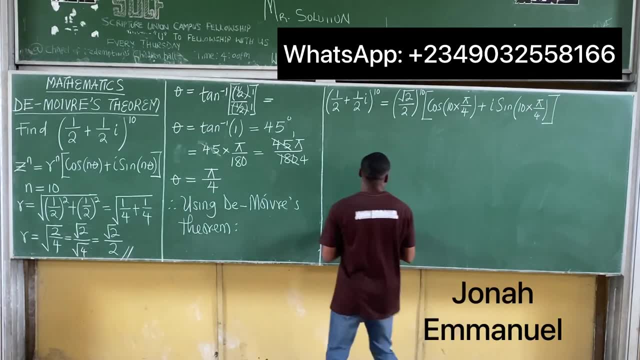 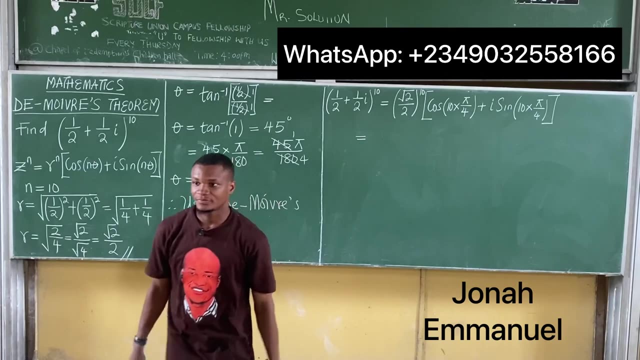 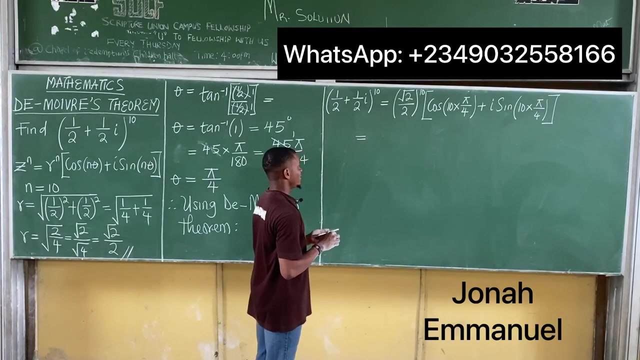 times theta, which we got here as pi over 4.. So I have this. Alright, so this is equal to. this is equal to, let's say, we can simplify this in the calculator. Okay, Alright, so simplifying this in the calculator. 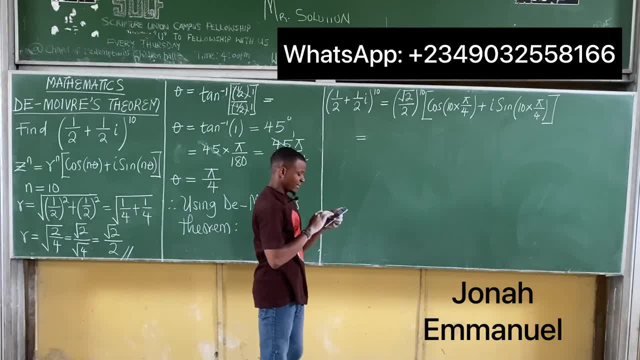 so I'm getting all of this at once. Let me see if I can get this Root 2 all over 2, all to the power, 10.. So if you punch this to the calculator, this to the calculator, this would give you. 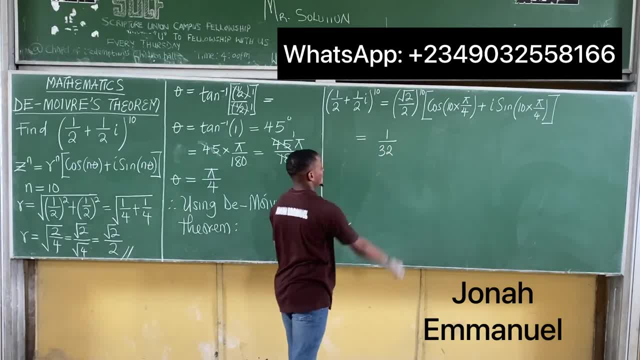 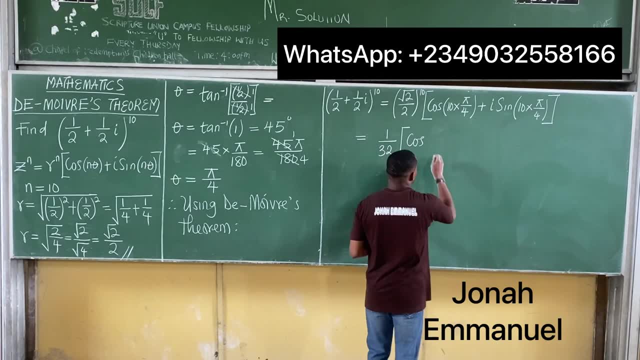 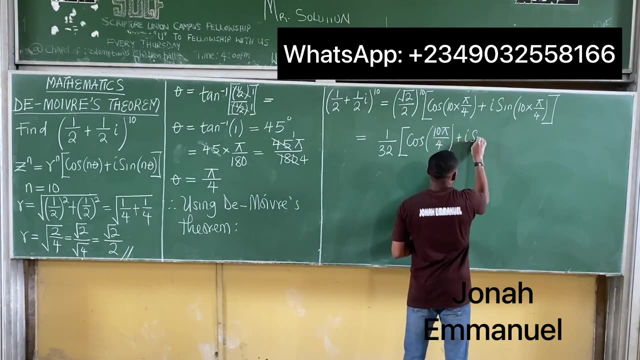 1 all over 32.. So you can go ahead and simplify this Next up. this now gives you into: I have cos 10 pi over 4, plus i sine 10 times pi, 10 pi over 4.. So I have. 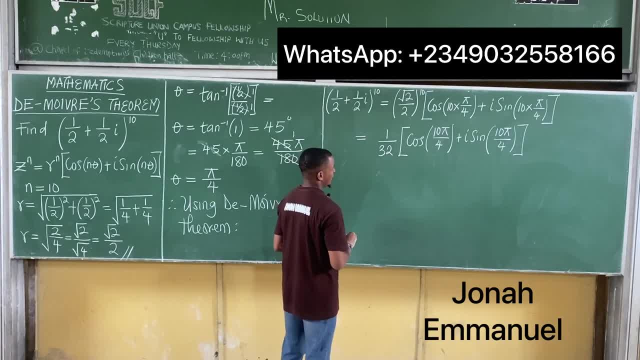 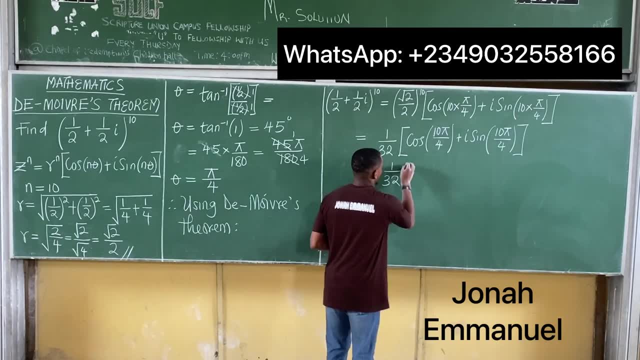 this one here. Alright, so simplify this. What do we have? This is equal to 1 over 32 into cos 4, 2 here, 2, 2 here 5.. That's 5 pi over 2.. 5 pi over 2. 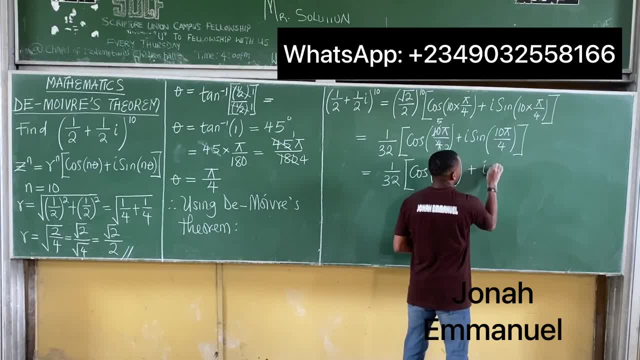 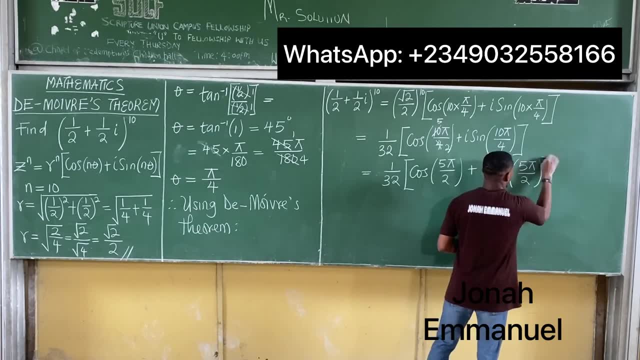 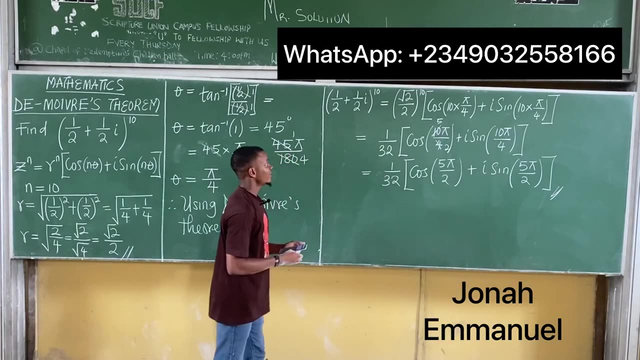 that's in lower stem. plus i sine. same thing here: 5 pi all over, 2 to the lowest stem or to the basic form I have there. So this becomes the answer. This one here is the value of this. This one is in radians. Let's get this in degrees. 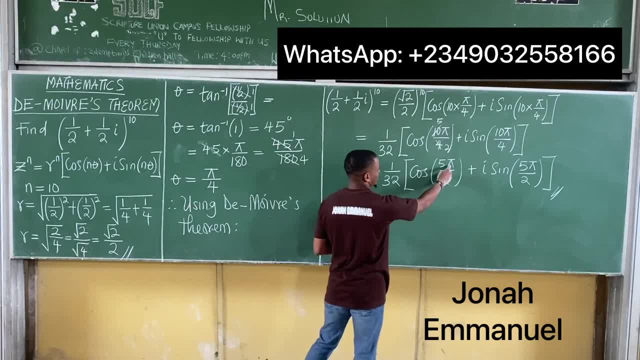 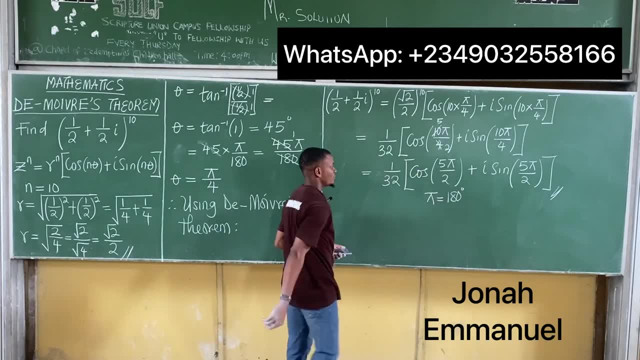 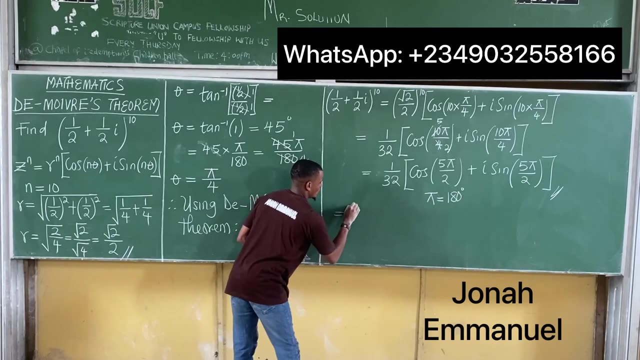 To get this in degrees is very simple: Simply put theta or simply put pi as 180. So pi will be equal to 180 degrees to get this value. So what does that mean? It means that in terms of degrees, this one would be equal to. 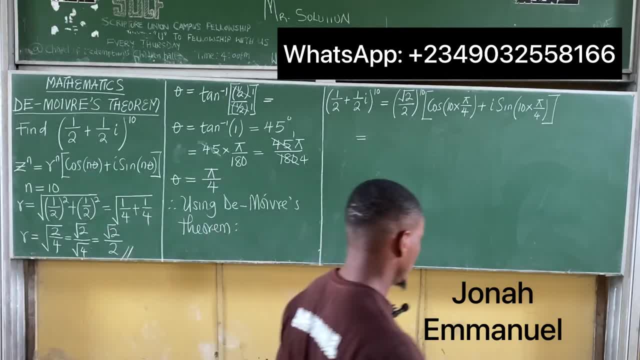 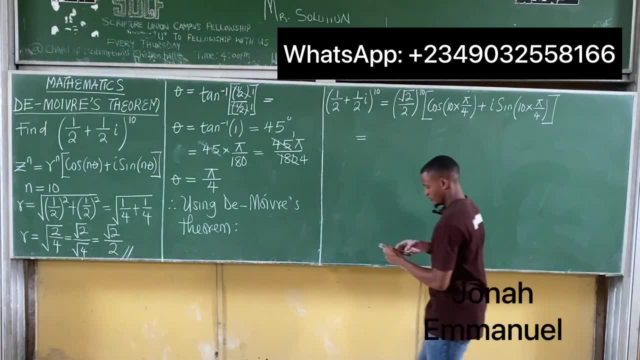 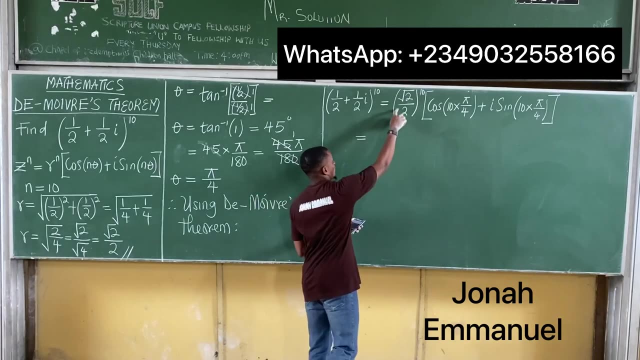 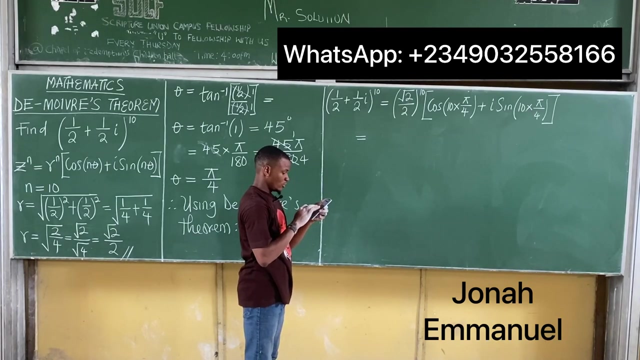 Okay, Alright, So simplifying this is in the calculator, So I'm getting all of this at once. Let me see if I can get this Root 2 all over 2, all to the power 10.. So if you punch this with the calculator, this with the calculator, this would give. 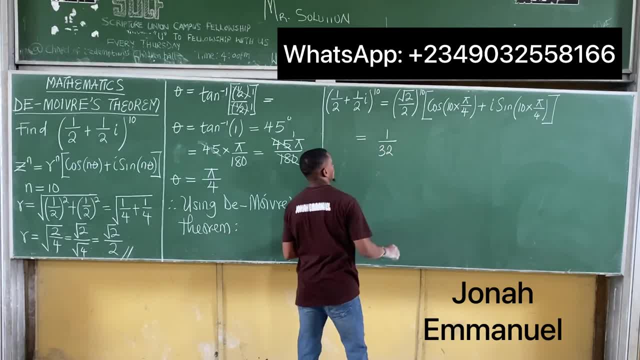 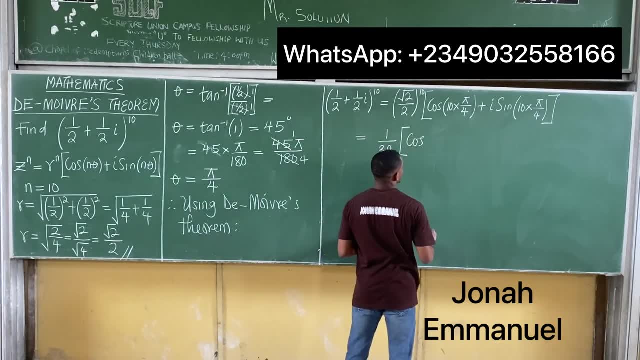 you 1 all over 32.. So you can go ahead and simplify this Next up. this now gives you into: I have cos 10 pi over 4, plus i sine 10 times pi, 10 pi over 4.. 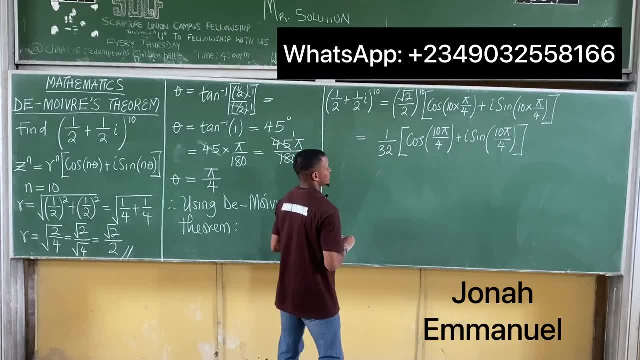 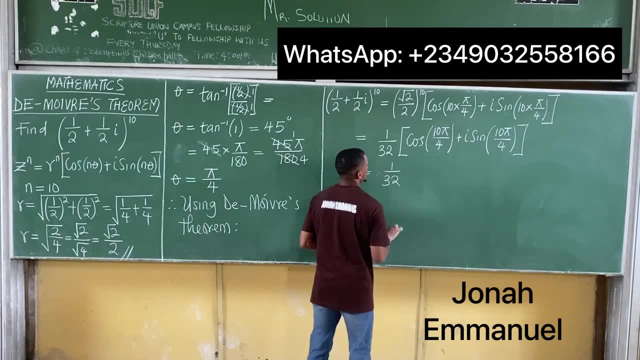 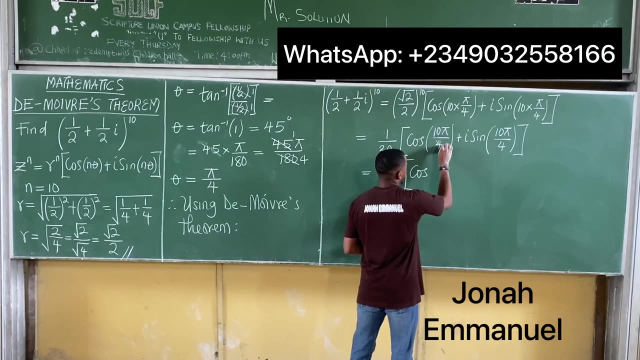 So I have This one here, Alright. So simplify this. What do we have? This is equal to 1 over 32 into cos: 4, 2 here, 2, 2 here 5. That's 5 pi over 2.. 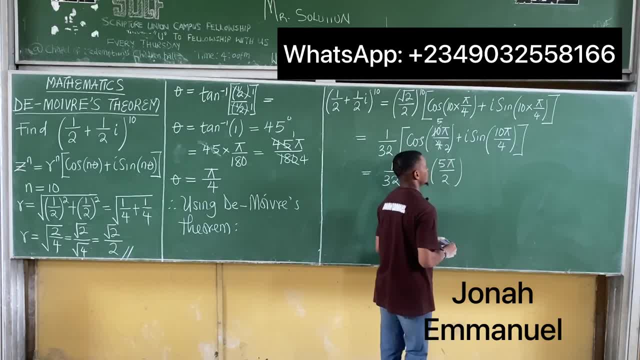 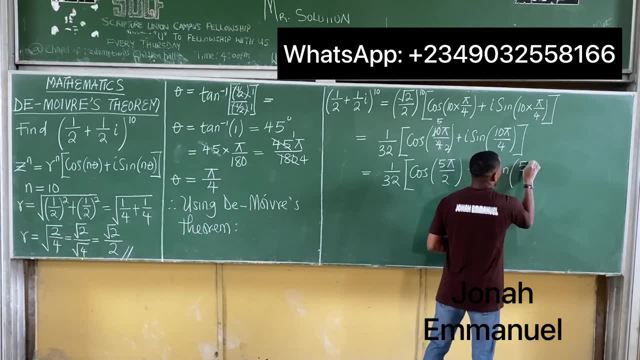 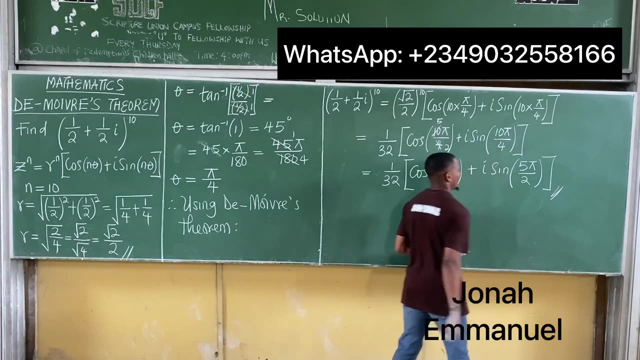 5 pi over 2.. That's in lower stem Plus i sine. Same thing here: 5 pi all over 2 to the lowest stem or to the basic form I have there. So this becomes the answer, This one here is the value of this. 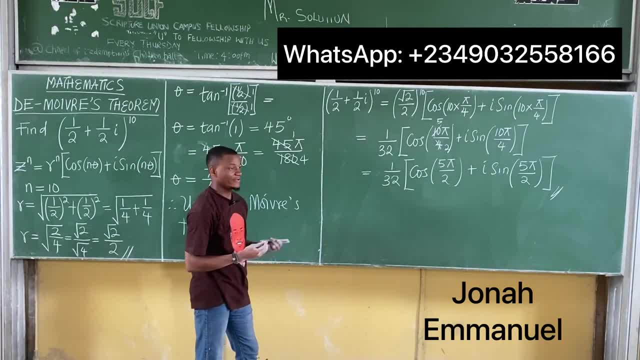 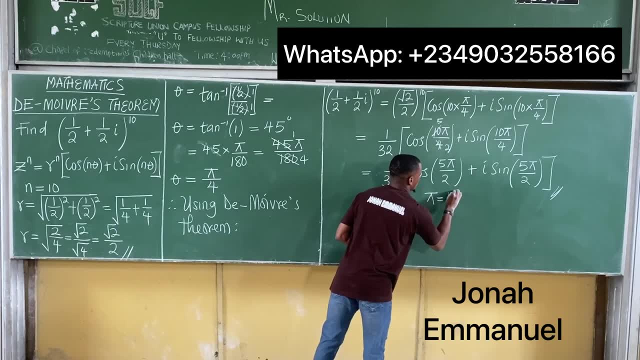 This one is in radians. Let's get this in degrees. So get this in degrees is very simple. Simply put theta, or simply put pi as 180. So pi will be equal to 180 degrees to get this value. So what does that mean? 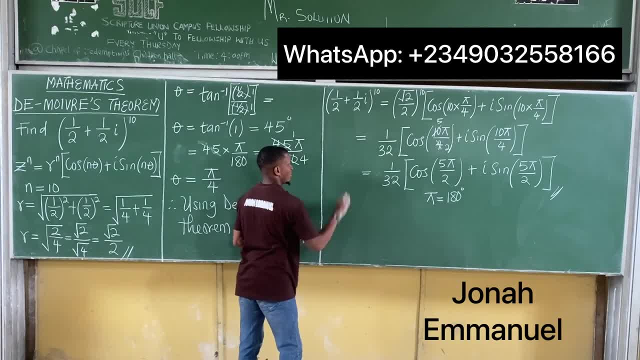 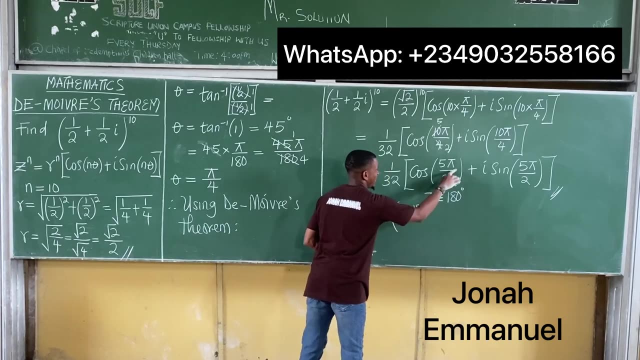 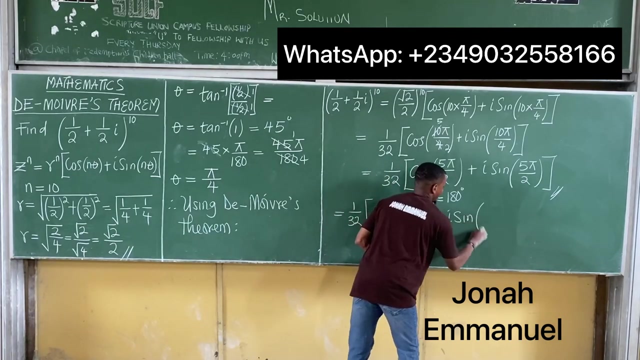 It means that in terms of degrees, This one will be equal to 1 over 32, into cos 5 times 180, pi is 180 degrees all over 2, plus i sine 5 times 180. So 5 times 180 all over 2.. 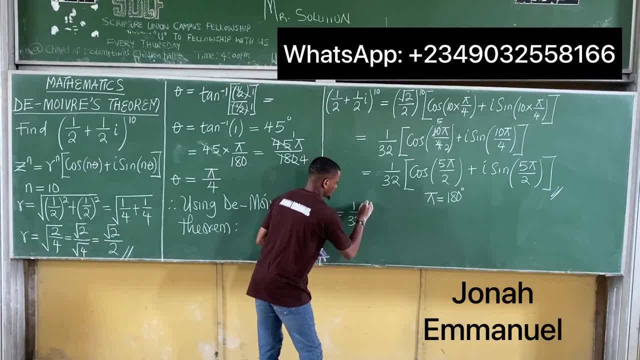 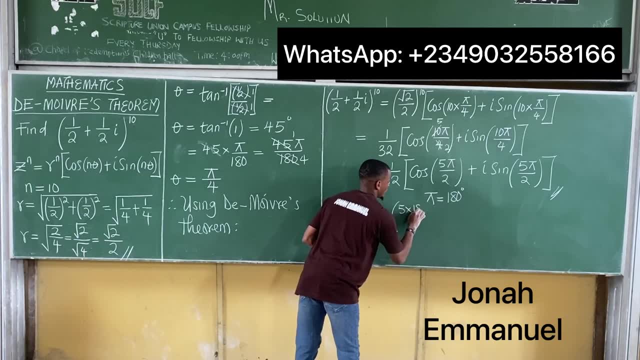 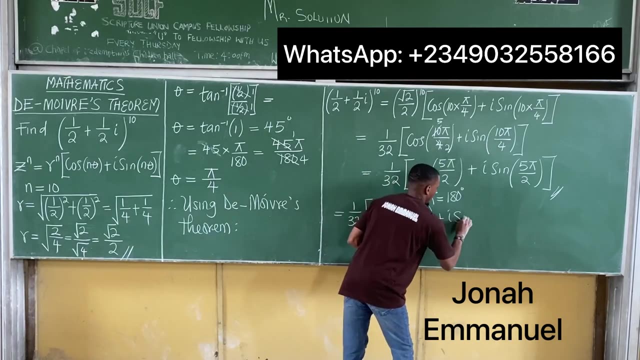 1 over 32 into cos 5 times 180. pi is 180 degrees all over 2, plus i sine 5 times 180. so 5 times 180 all over 2 and I have this Okay. so what do we have here? 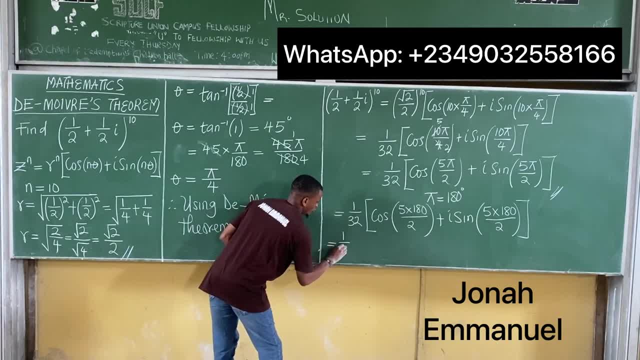 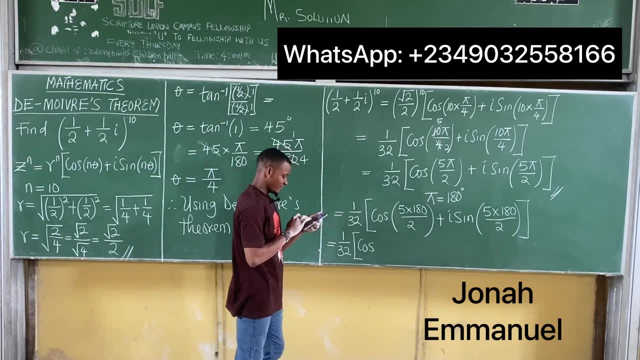 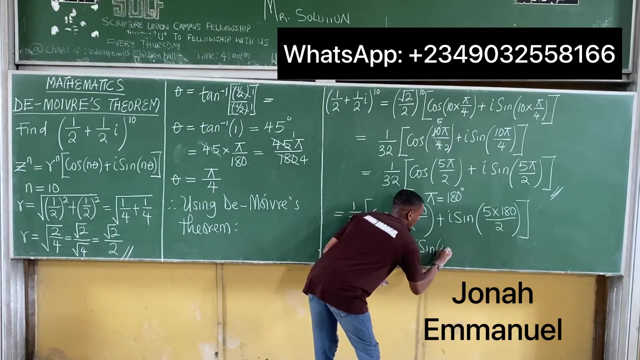 So this would be equal to 1 over 32 into cos. So let's get 5 times 180, that's 900 over 2, that's 450.. That's cos 450 now in degrees, plus i sine 450 in degrees. so I have this. 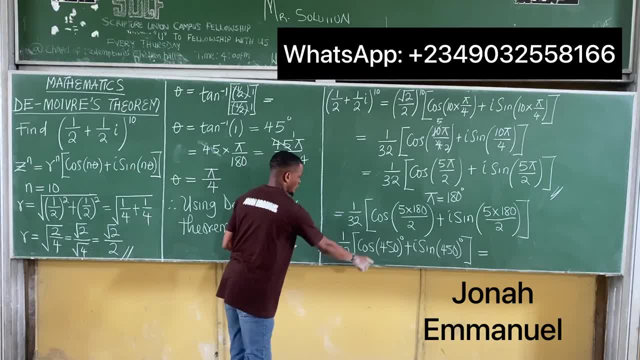 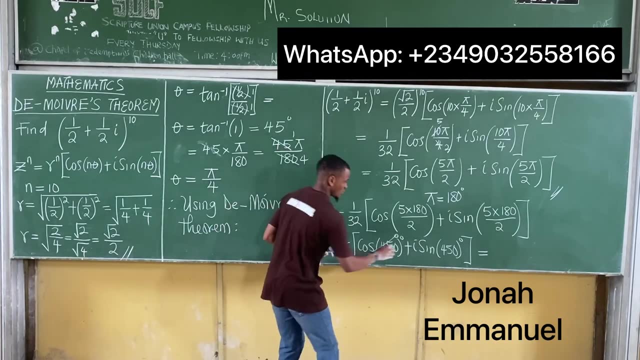 that would be equal to. you can choose to convert this. or let me go straight: cos 450, cos 450. here. if you punch this calculator in degrees, this gives you 0. alright, sine 450 gives 1, so this one gives you 1. so in essence, this is: 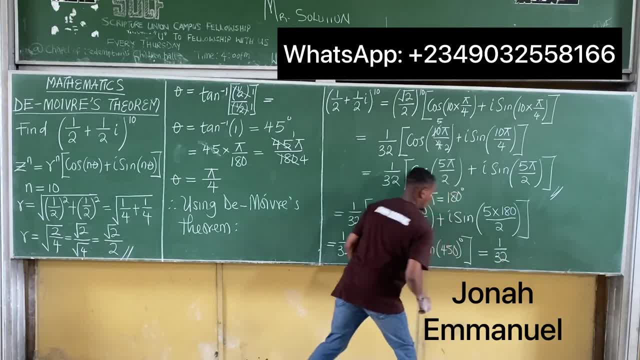 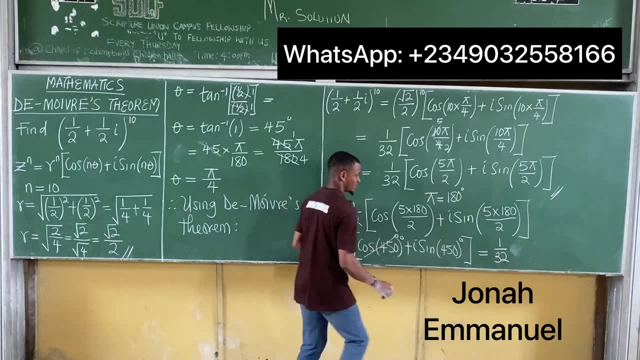 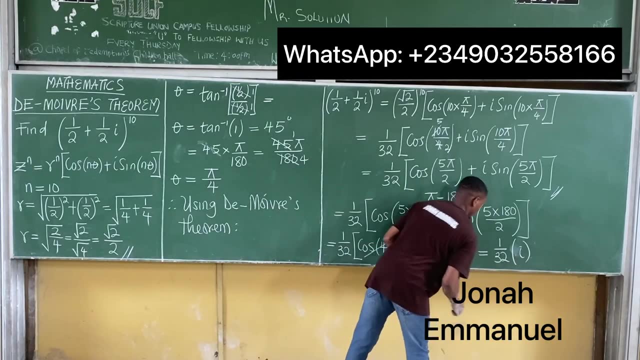 equal to 1 over 32. this one gives 0, so it's off plus- I'm having sorry- multiplied by. so this is 0 plus 32 into 0, it's off, plus i times 1, that's i. so this one gives you i. you can punch this sine 450. 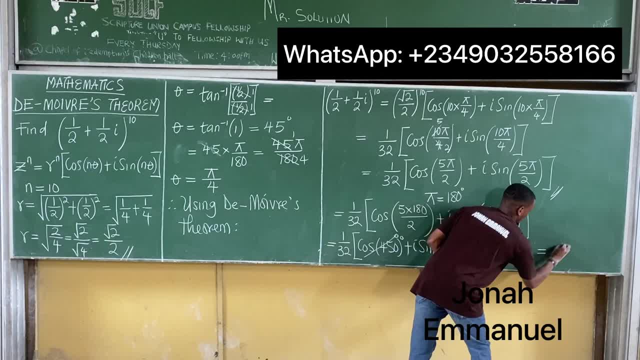 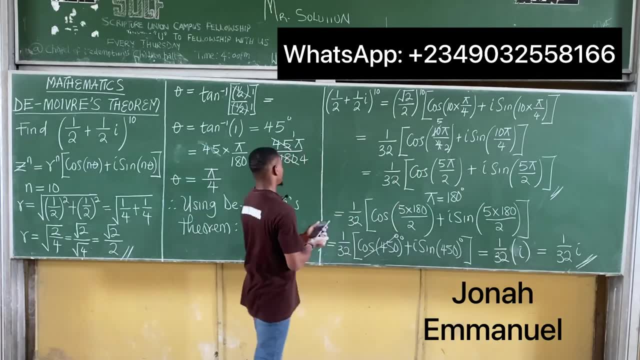 you have i, that's i. so if I multiply this, this is equal to 1 over 32 i. so you have this answer alright. so I've gotten this value alright. so this is how we can use the Moivre's theorem to simplify getting the nth. 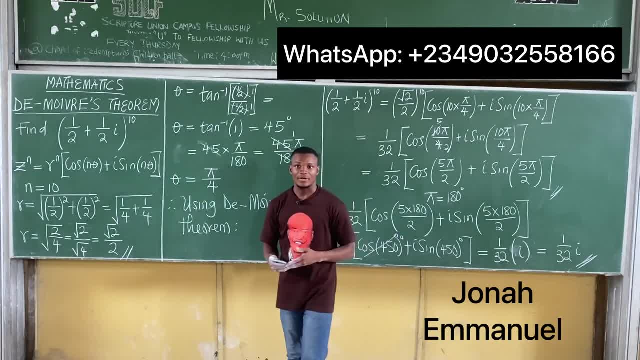 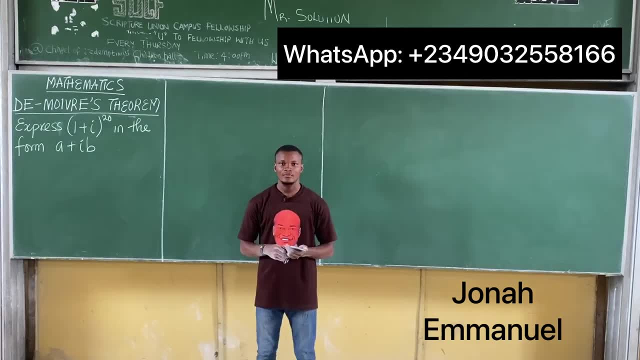 power of a complex number. alright, so this is how it's done. alright, so this is how we work on the Moivre's theorem. alright, so let's take another example on the Moivre's theorem. this question says: express 1 plus i to power 20 in the form: 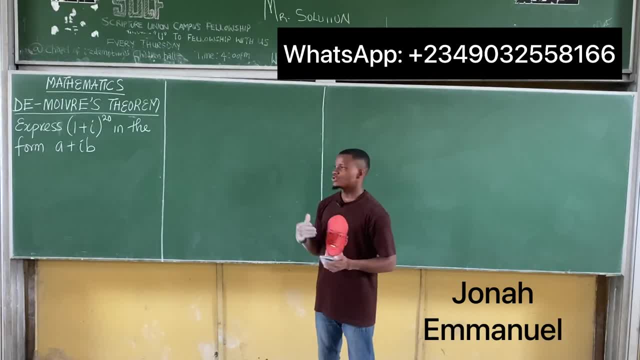 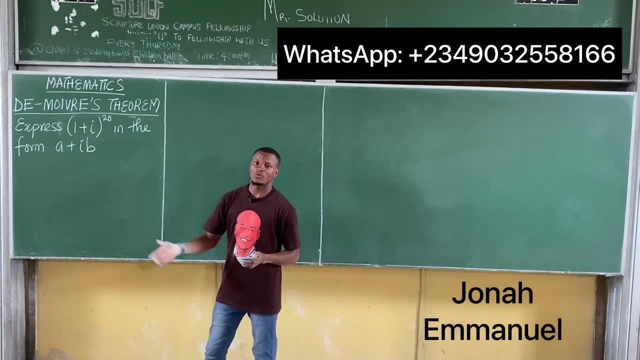 a plus ib now in this case. here we have to use the Moivre's theorem, because the power here is quite large and we can't start expanding this or by multiplying itself one by one. that will waste time. let's use the Moivre's theorem straight up. 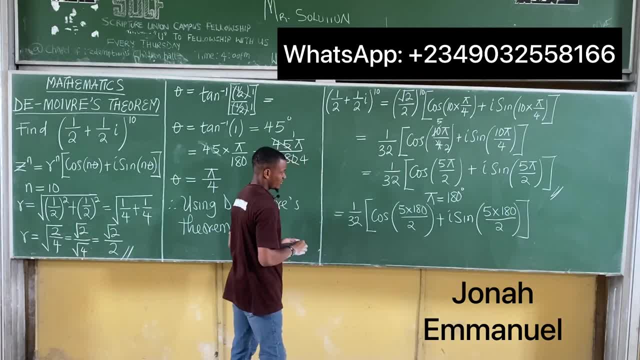 And I have This Okay. So what do we have here? So this will be equal to 1 over 32 into cos. So let's get 5 times 5 times 180.. That's 900 over 2.. 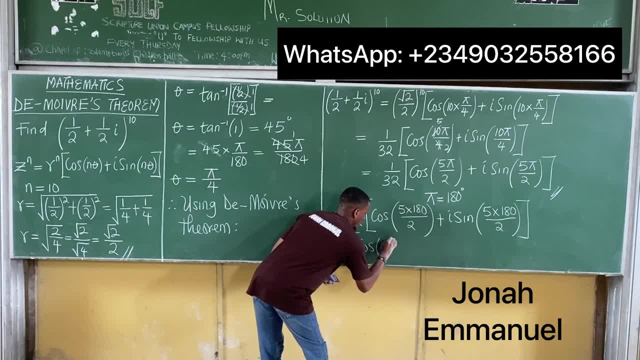 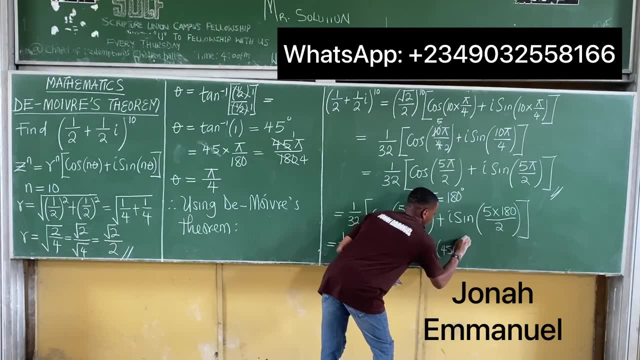 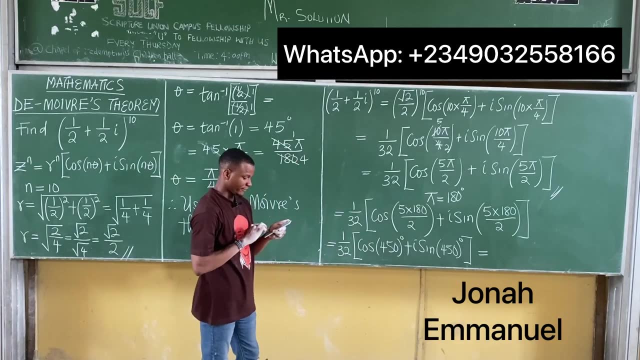 That's 450.. That's cos 450.. Now, in degrees Plus i sine 450.. So I have this. That will be equal to. You can choose to convert this Or let me go straight: Cos 450.. 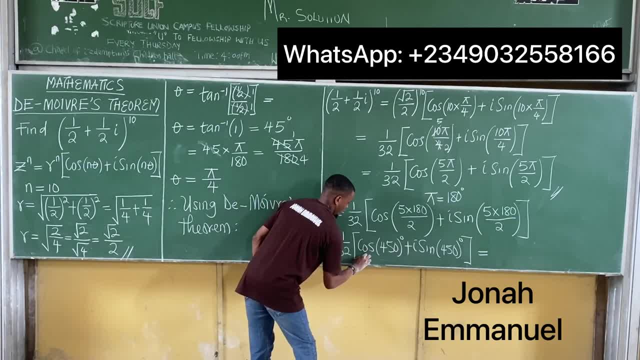 So cos 450 here? If you punch this calculator in degrees, This gives you 0. Alright, Sine 450.. Sine 450 gives 1. So this one gives you 1.. So in essence this is equal to 1 over 32.. 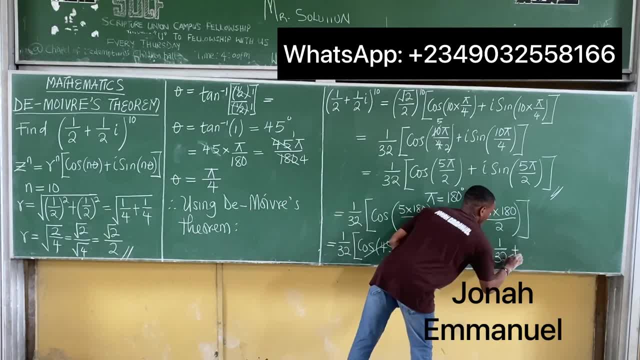 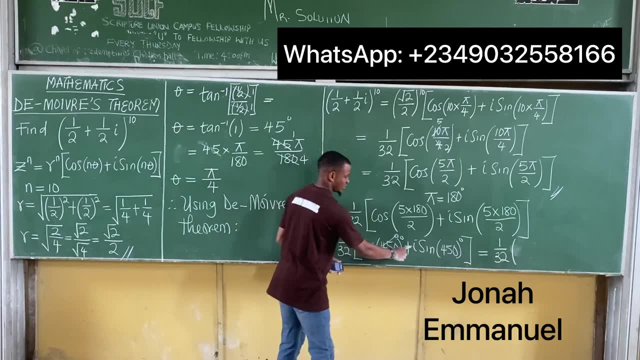 This one gives 0.. So it's off plus I'm having. sorry. It multiplied by. So this is 0 plus 32 into 0.. It's off Plus i times 1.. That's i. So this one gives you i. 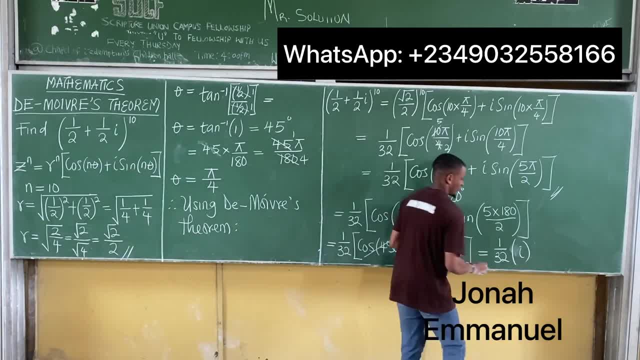 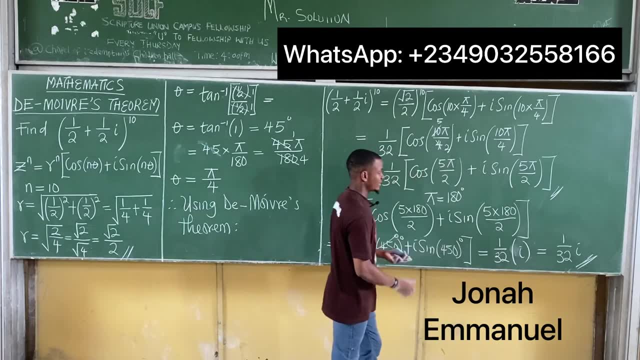 You can punch this Sine 450.. You have i, That's i. So if I multiply this, This is equal to 1 over 32 i So you have this answer Alright. So I've gotten this value. 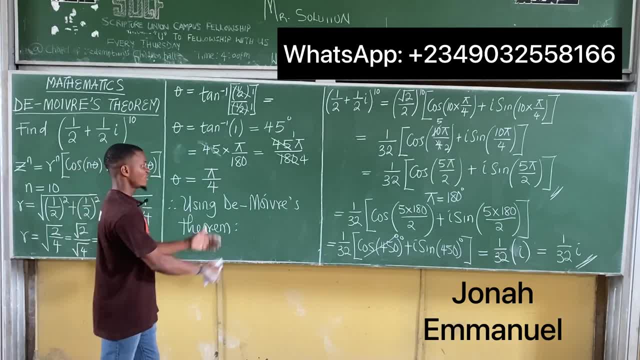 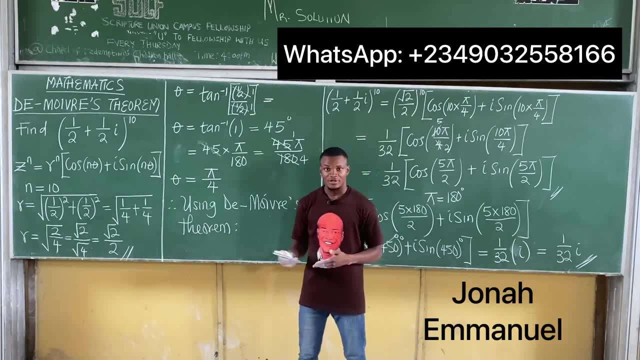 Alright, So this is how we can use the Moebius theorem To simplify getting the nth power of a complex number. Alright, This is how it's done. Alright, So this is how we work on the Moebius theorem. 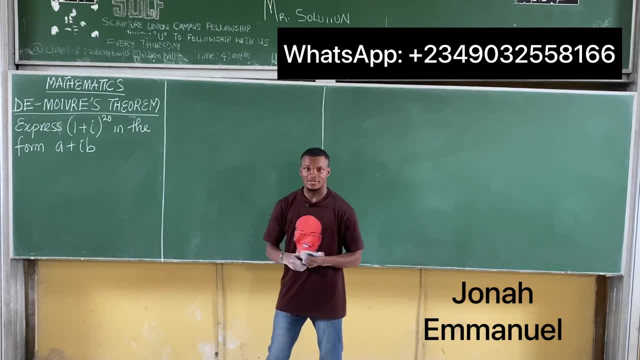 Alright. So let's take another example on the Moebius theorem. This is express 1 plus i to the power 20 in the form a plus ib. Now, in this case, here we have to use the Moebius theorem. 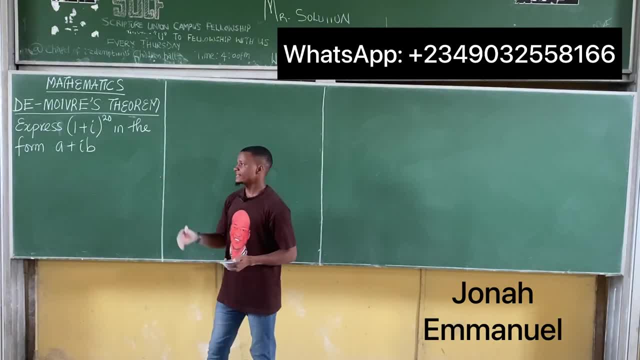 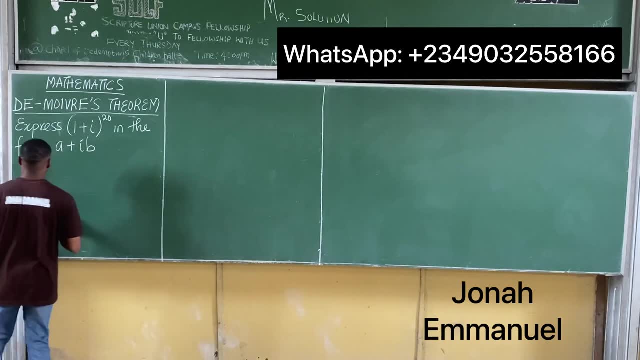 Because the power here is quite large And we can't start expanding this by multiplying itself one by one. That will waste time. Let's use the Moebius theorem straight up. So that would mean: Let's get r first From here, of course. 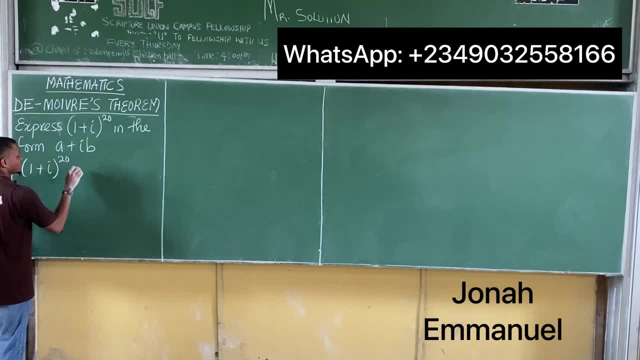 If I have 1 plus i, to the power 20.. It means that n is equal to the power, That's 20.. r is equal to the square root of d, squared 1. squared plus I'm having i Coefficient here is 1.. 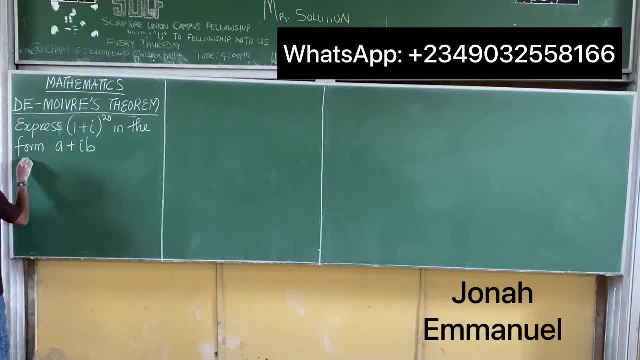 so that will mean let's get r first from here, of course. if I have 1 plus i to power 20, it means that n is equal to the power that's 20. r is equal to the square root of d squared 1 squared plus. 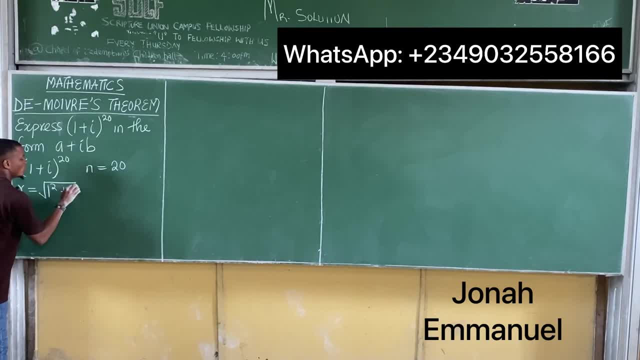 I'm having. i coefficient here is 1, so 1 squared so that's equal to the square root of 1. squared is 1 plus 1 squared is 1, that's equal to root 2. let's get theta. theta is equal to tan inverse of. 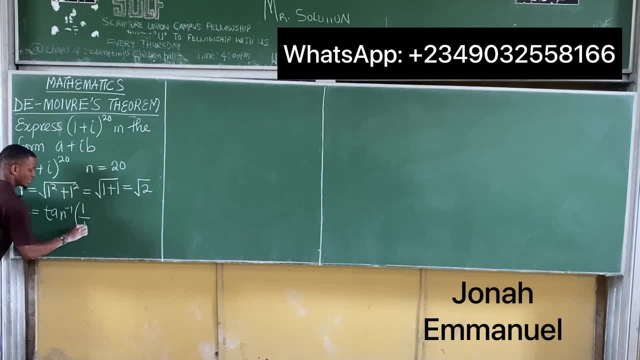 b, that's 1, all over a, that's 1, and that's equal to tan inverse of 1 over 1 is 1, so it becomes tan inverse of 1, which we got previously as 45 degrees, so that's tan inverse of 1. 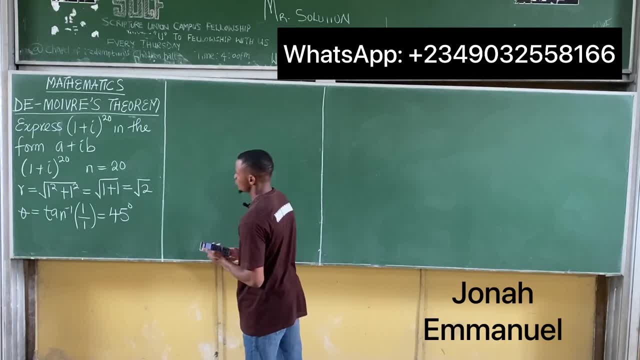 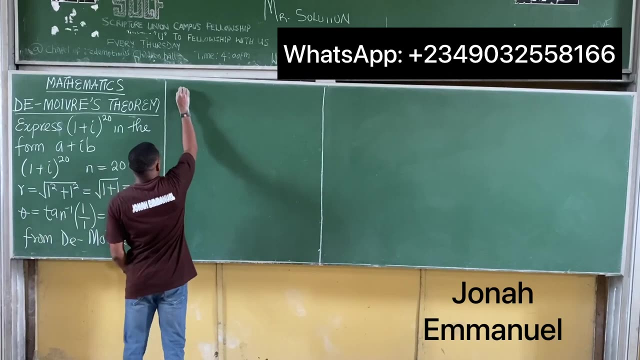 as 45 degrees. so if this is true, let's now do the idea of the Moivre's theorem. so, from the Moivre's theorem, so from the Moivre's theorem, from the Moivre's theorem, what do we have? we have that z to power. 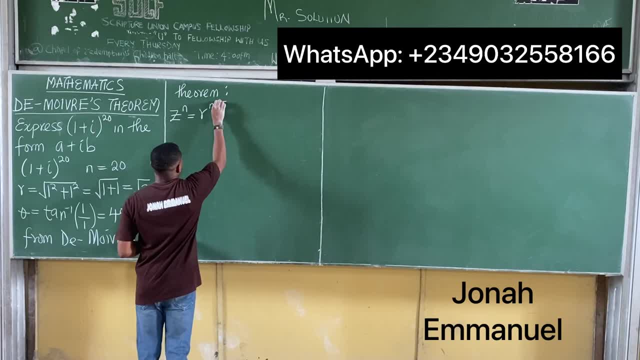 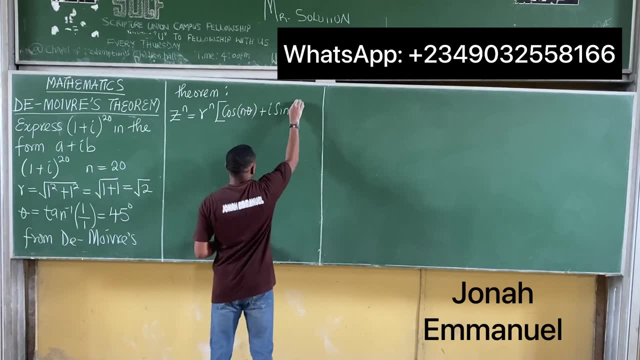 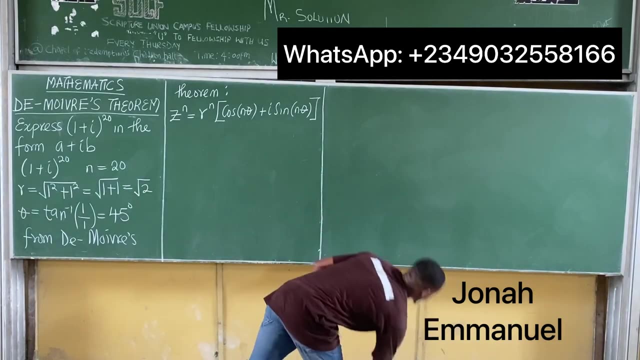 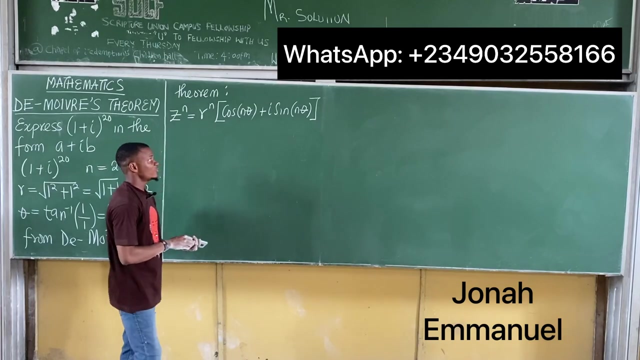 n is equal to r to power n into cos of n, theta plus i sine and theta. so I have this one here, alright. so in our first example we said: let's use theta, let's convert theta to pi and work with radians. but in this case, if I work, 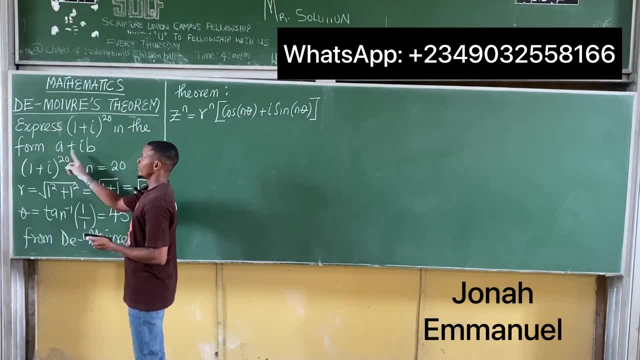 with pi or radians, I won't get my answer in this form. to get my answer in this form, I have to work with degrees. that's the idea. work with degrees. so that means 1 plus 1 plus i to power n, that's tan will be equal to r, r here is 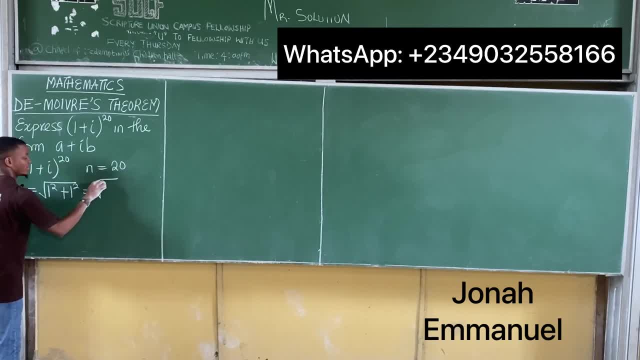 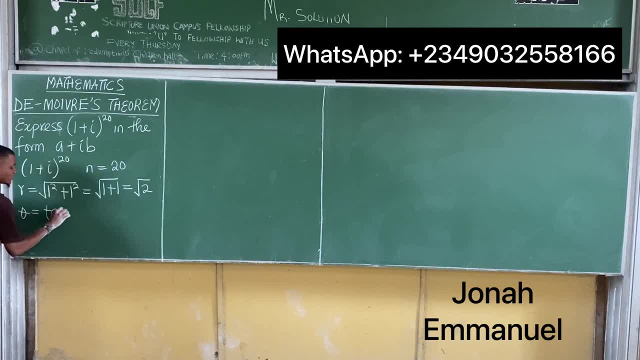 Let's get theta. Theta is equal to tan inverse of b, That's 1.. All over a, That's 1.. And that's equal to tan inverse of 1 over 1 is 1.. So it becomes tan inverse of 1.. 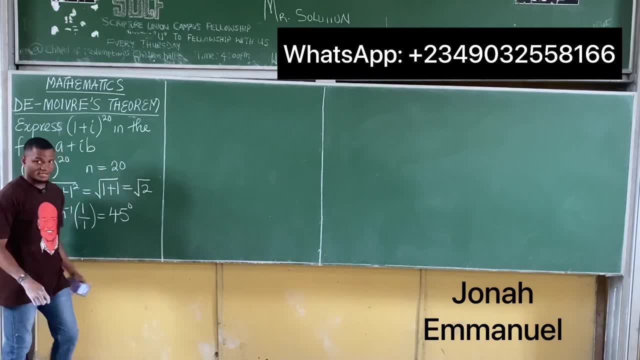 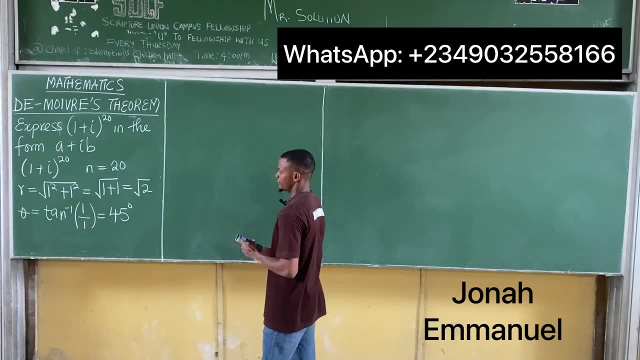 Which we got previously as 45 degrees, That's tan inverse of 1 as 45 degrees. Alright, So this is true. Let's now do the idea of the Moivre's theorem. So from the Moivre's theorem. 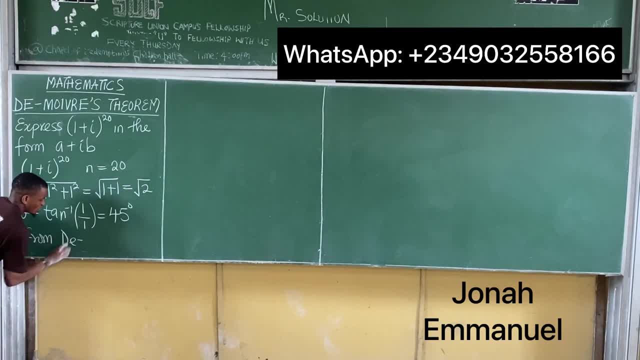 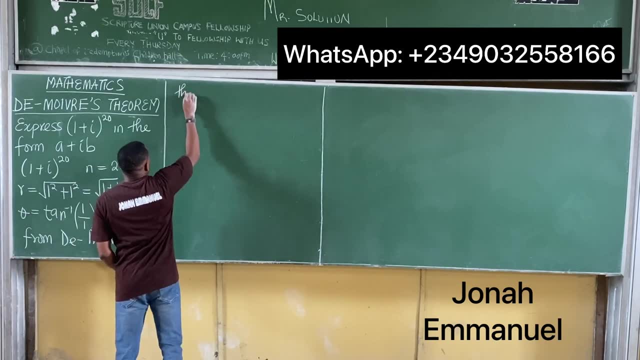 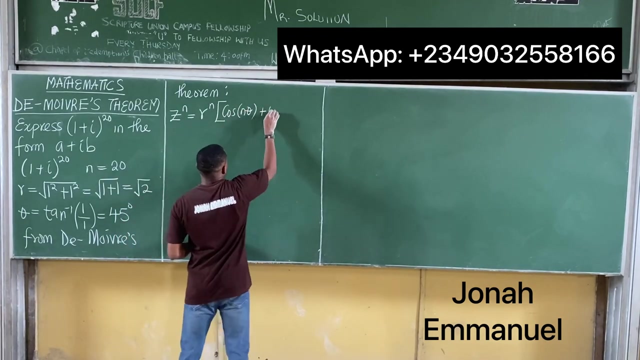 So, from the Moivre's theorem, From the Moivre's theorem, What do we have? We have that z to the power n is equal to r to the power n into cos of n, theta plus r to the power n, i, sin and theta. 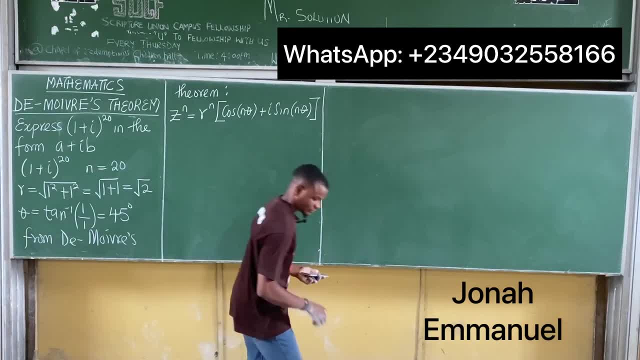 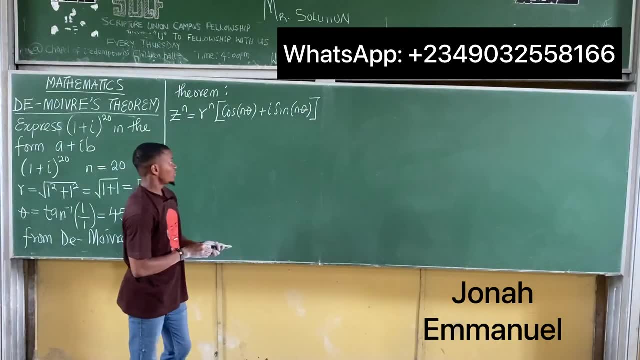 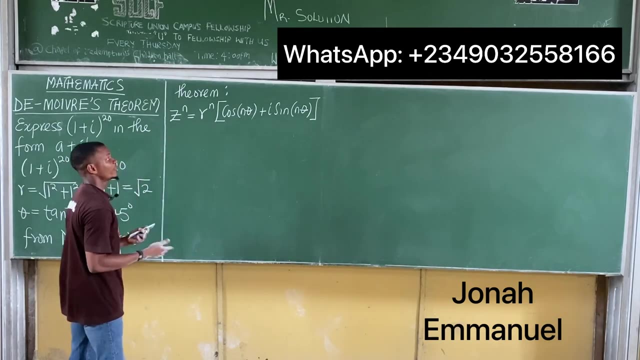 So I have this one here, Alright. So in our first example we said: let's use theta, Let's convert theta to pi and work with radians. But in this case, if I work with pi or radians, I won't get my answer in this form. 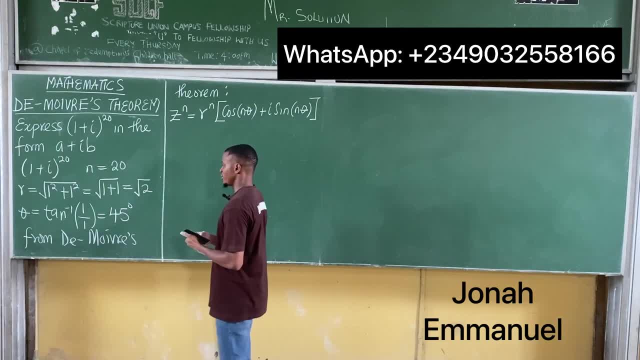 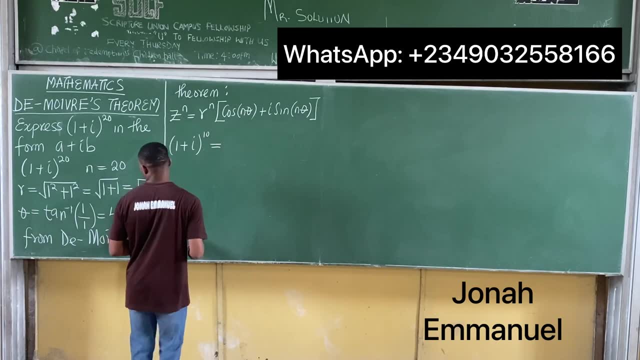 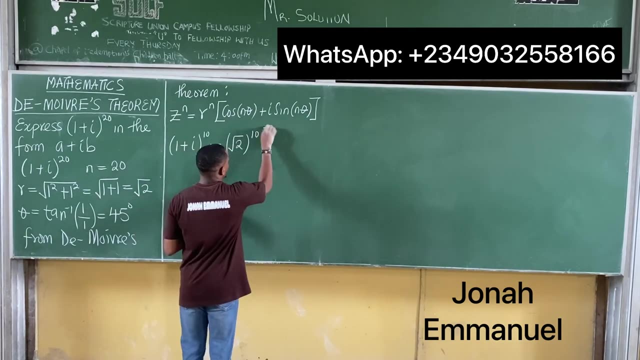 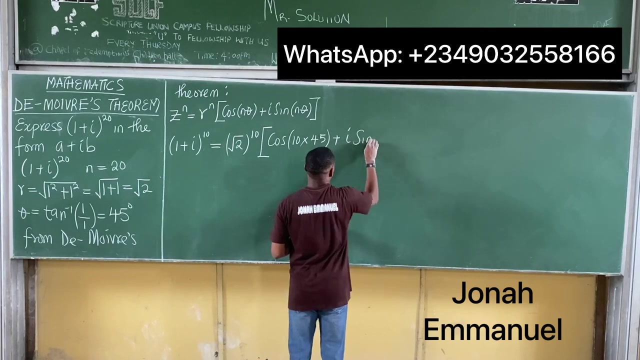 To get my answer in this form I have to work with degrees. That's the idea, Work with degrees. So that means 1 plus 1 plus i to power n, that's 10 will be equal to r. r here is 2 or 2, that's root. 2 to power 10 into cos. so cos n? n, that's 10 times theta, is 45, so 45 degrees plus i sine n, n is 10.. 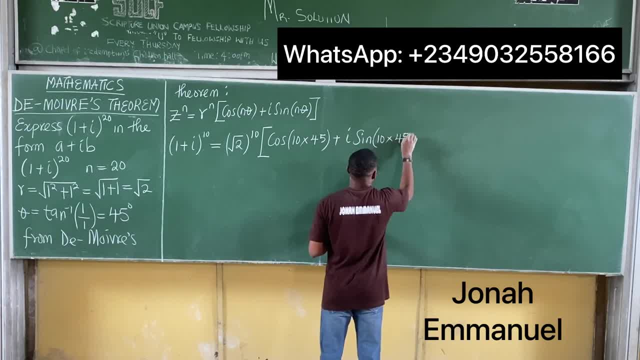 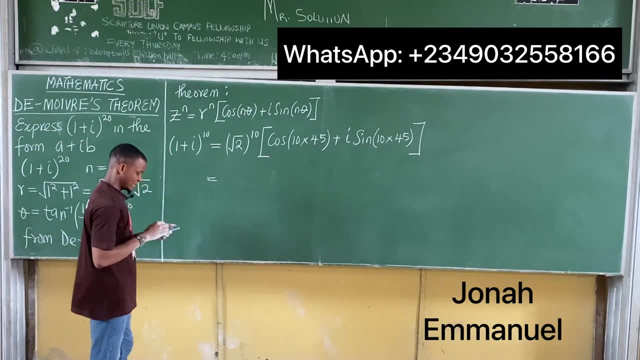 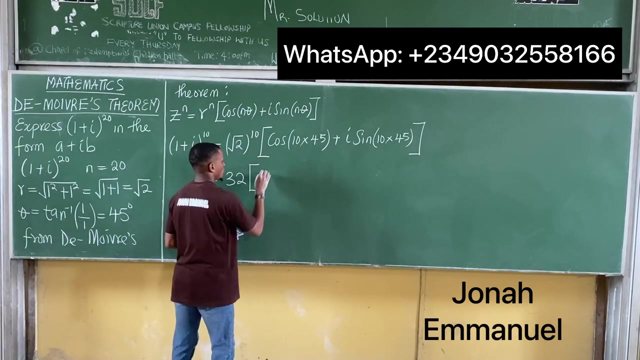 times theta, that's 45 degrees. so i have this one here. alright, so this is equal to root 2 to power 10, let's see the answer: root 2 to power 10, the answer here is 32, so it becomes 32 into here. i have this as cos, that's cosine of 10 times 45 is 450. 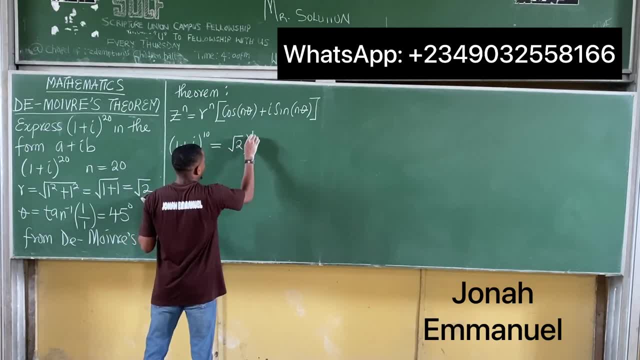 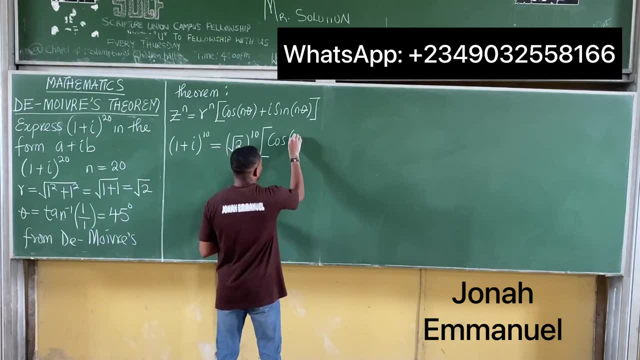 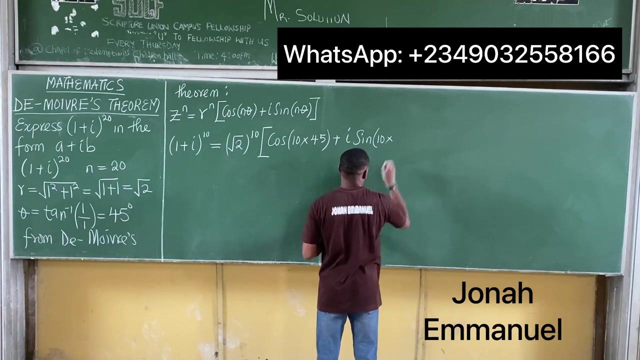 2 or 2, that's root 2 to power 10 into cos. so cos n? n, that's tan times theta, is 45, so 45 degrees plus i sine n? n is tan 10 times theta, that's 45 degrees. so I have. 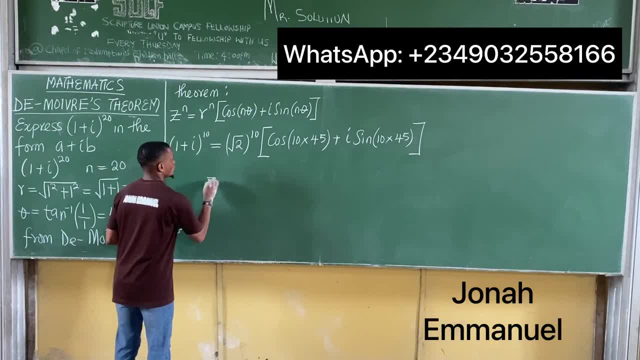 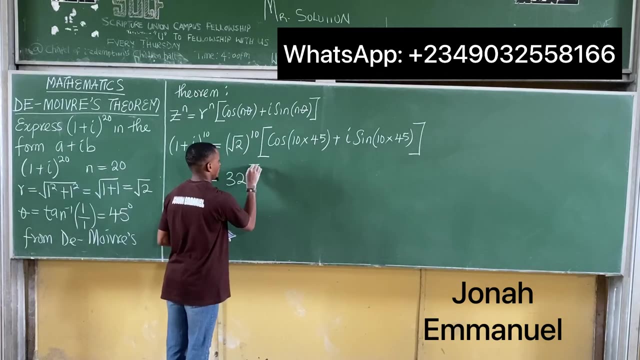 this one here. alright, so this is equal to root 2 to power 10. let's see the answer: root 2 to power 10. the answer here is 32, so it becomes 32 into here. I have this as cos that's cosine of 10. 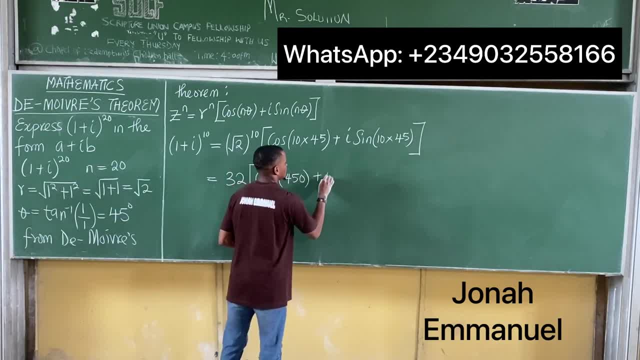 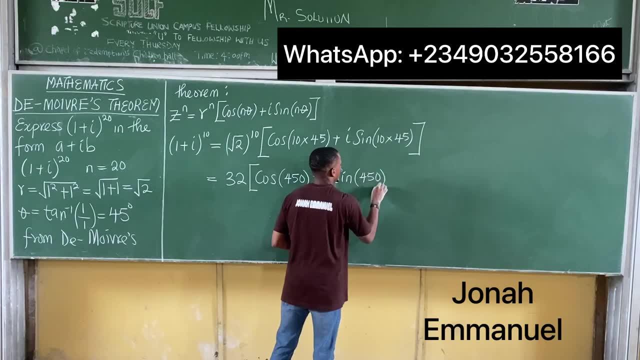 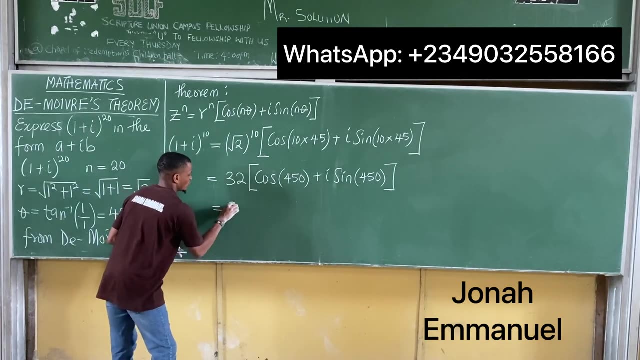 times 45 is 450, plus i i sine 10 times 45 is 450, so I have this alright. so just pause this directly and see our answer. this is equal to 32 cos 450. I thought we got it as 0, yup, so this one here is. 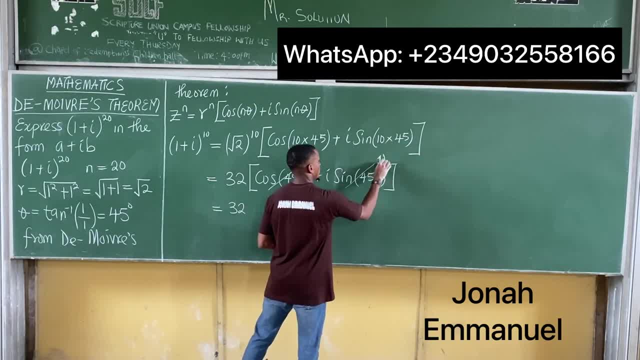 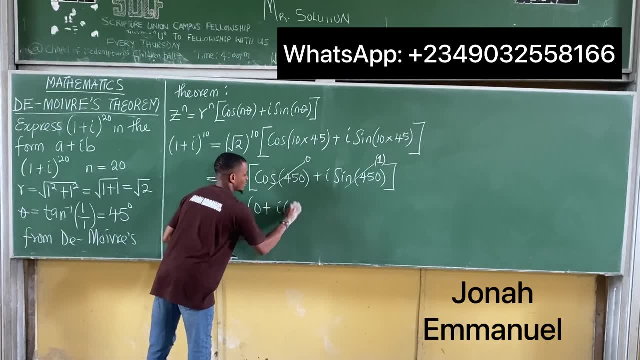 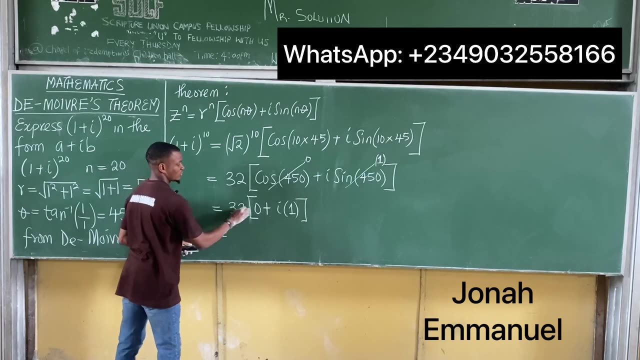 0 sine 450 gives you 1, so that is equal to 32 into 0 plus i times 1, so I'm having this, so that is equal to: of course this one is off. so 32 times 1 times i gives you 32 i. 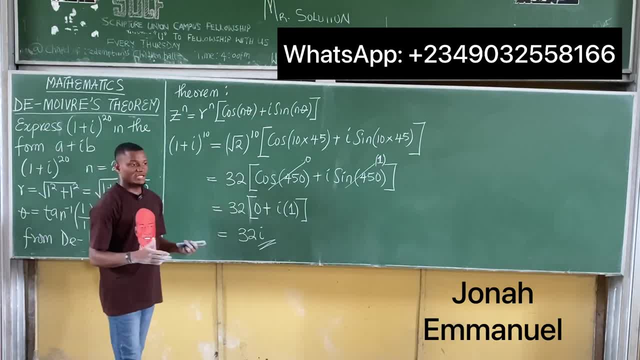 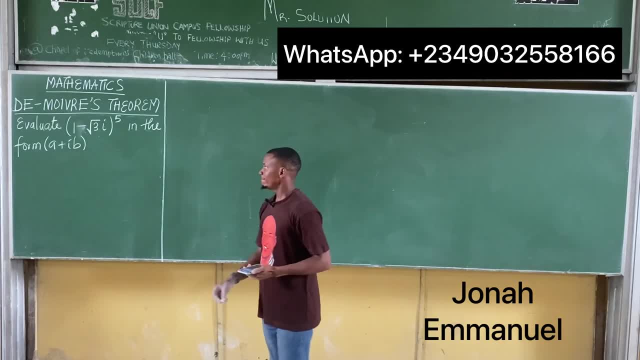 so that's how we solve this question. we'll take a final example on the Moivre's theorem and then we'll look at something else. alright, so let's get a final example on the Moivre's theorem. so this question says: evaluate 1 minus root 3. 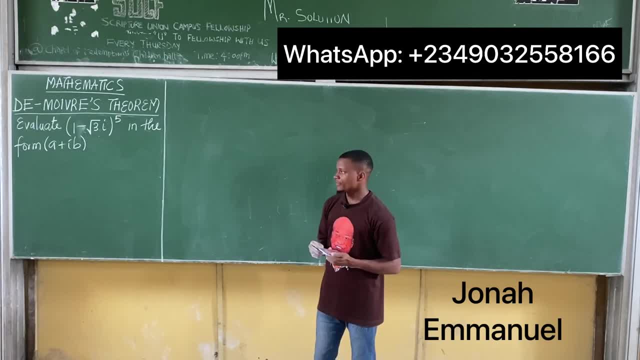 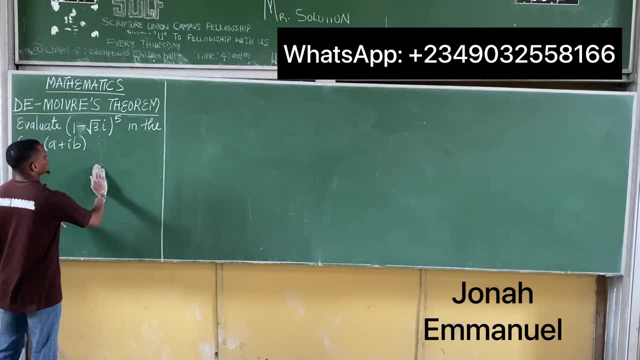 i to power 5 in the form a plus ib. alright, so how do we get this done? very easy: for this we'll have to use the Moivre's theorem. if you have the time, you could choose to expand this 5 times and see if we'll have. 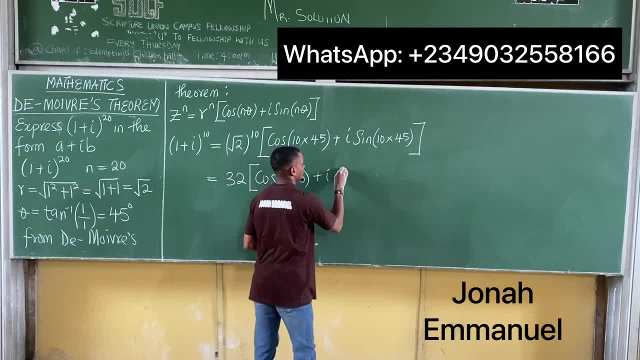 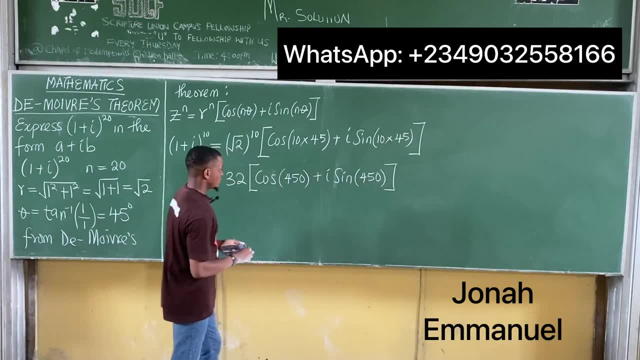 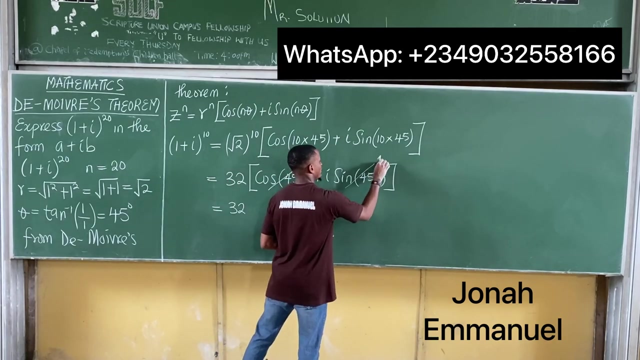 n plus i. i sine 10 times 45 is 450, so i have this alright. so just push this directly and see the answer. this is equal to 32 cos 450,. I don't even got it at 0, yup, so this one here is 0, sine 450 gives you 1, so that is equal to 32 into 0 plus n n. 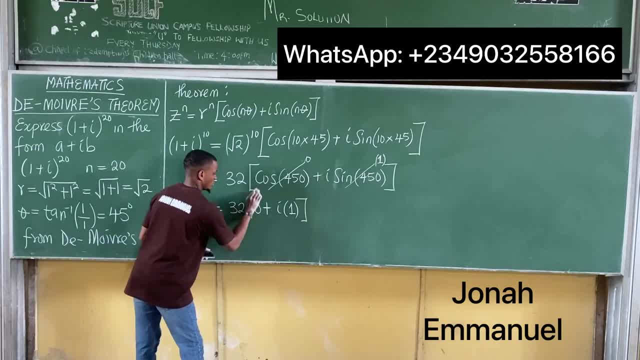 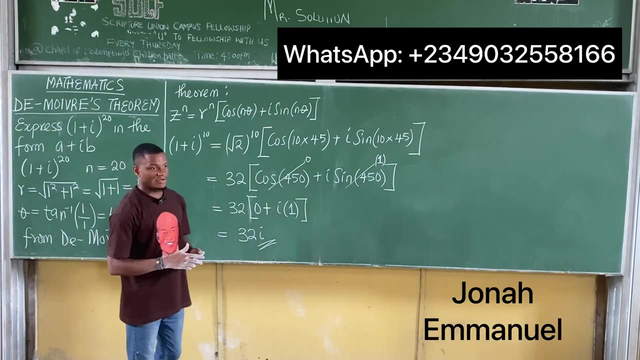 I times 1, so I'm having this. so that is equal to. of course, this one is off. so 32 times 1 times I gives you 32 I. So that's how we solve this question. We'll take a final example on the Moivre's theorem and then we'll 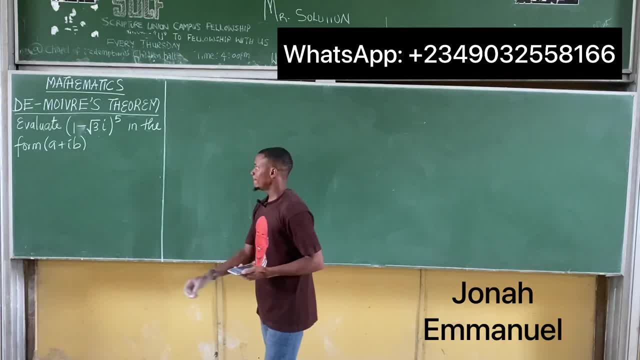 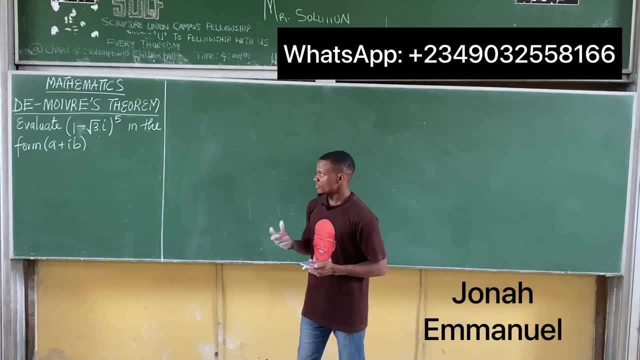 look at something else. Alright, so let's get a final example on the Moivre's theorem. This question says: evaluate 1 minus root, 3, I to power 5 in the form A plus IB. Alright, so how do we get this done? Very easy. 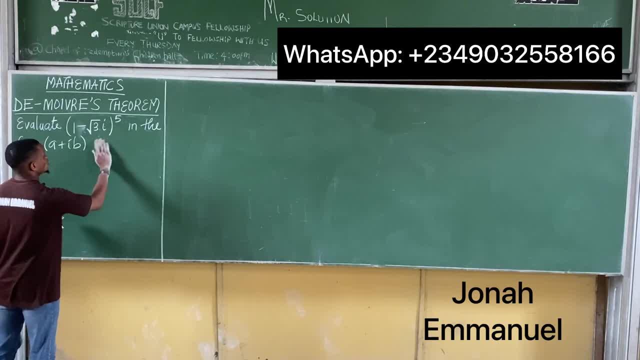 For this one we'll have to use the Moivre's theorem. If you have the time, you could choose to expand this 5 times and see if we'll have the same answer. But then I'm using the Moivre's theorem. so 1 minus 3. 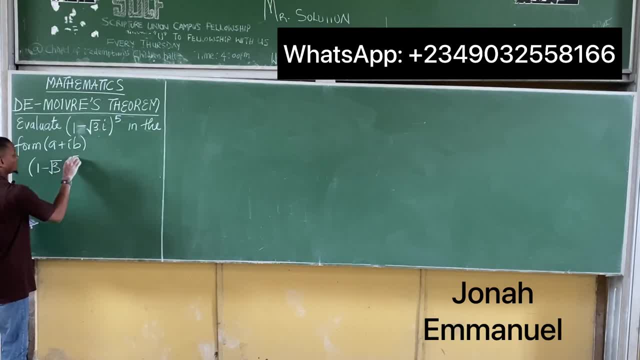 root 3. I okay to power 5.. Let's get this done. So for this case here n is equal to the power, which is 5.. Let's get r, So r will be equal to the square root of. 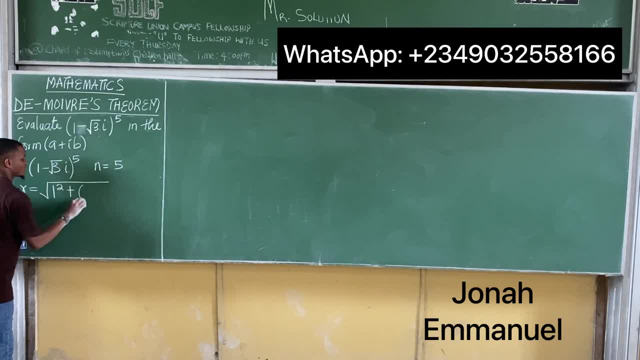 this one here, 1 squared plus this one here, minus root 3. all squared, So r will be equal to the square root of 1, squared is 1 plus. let's get this one done. this is minus root 3, multiplying minus root 3. 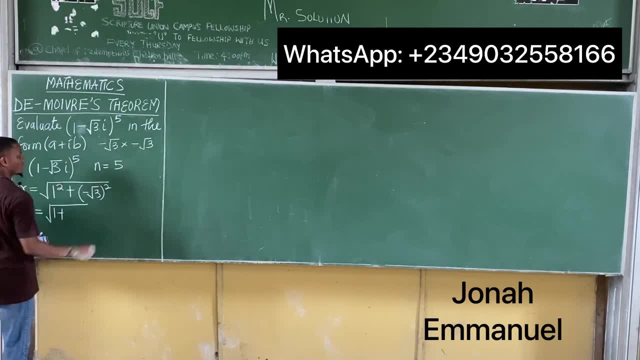 minus minus is plus root. 3 times root 3 is 3.. So my answer is plus 3.. Okay, work on this. That's equal to the square root of 1 plus 3 is 4, and that's equal to. 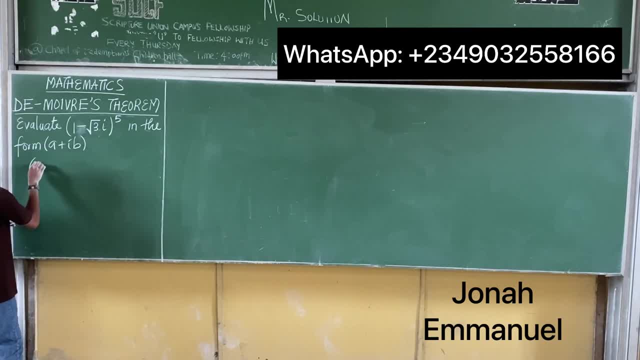 the same answer, but then I'm using the Moivre's theorem. so 1 minus 3 root 3. i okay to power 5. let's get this done. so for this case, here n is equal to the power, which is 5. let's get r. 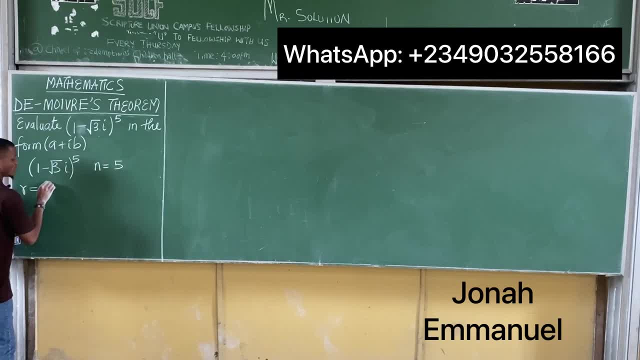 so r will be equal to the square root of this one here, 1 squared plus this one here, minus root 3. all squared, so r will be equal to the square root of 1. squared is 1 plus. let's get this one done. this is minus root 3. 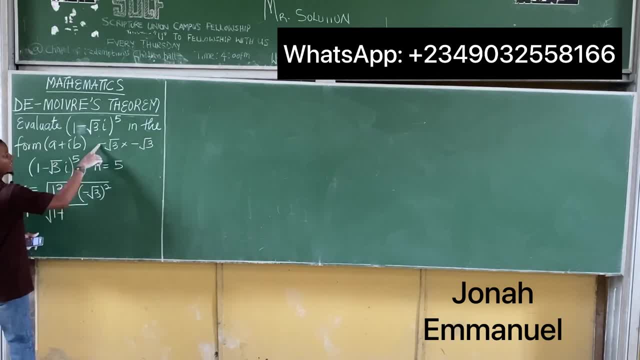 multiplying minus root 3, minus is plus root. 3 times root 3 is 3, so my answer is plus 3. okay, work on this. that's equal to the square root of 1 plus 3 is 4, and that's equal to square root of 4 is. 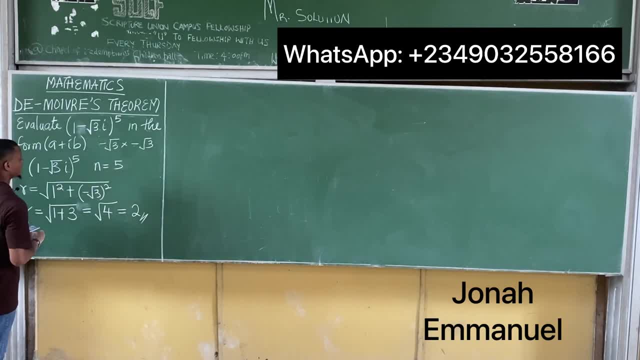 2, so I have this as 2. next let's find the angle so theta is equal to. before you watch this, please make sure you've checked our previous video on how I explained how to get theta and theta reference, so for this one here you should know the. 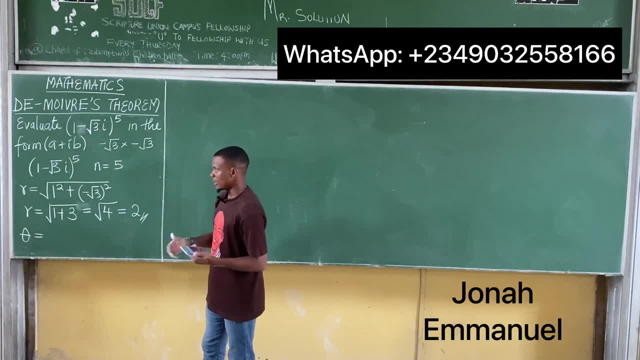 quadrant positive x, negative. i that should be quadrant 4, and you know how to get the reference. I'll leave a link to that video in the description of this video. so just check the description. you'll see a link to the explanation of how to get the. 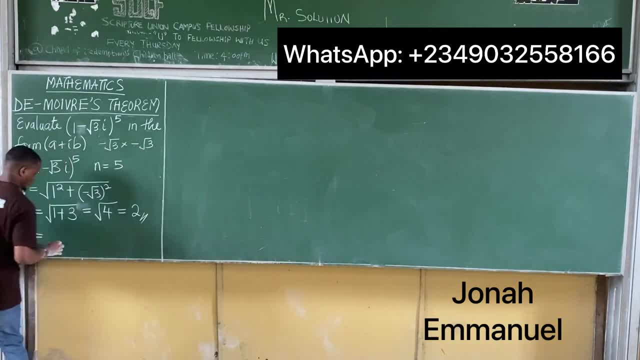 correct angle, but let's proceed with this. so that's equal to theta is equal to tan inverse. so tan inverse of. you said you could forgo the negative sign. I'll just take root 3 all over 1. okay, so b over a. so theta is equal. 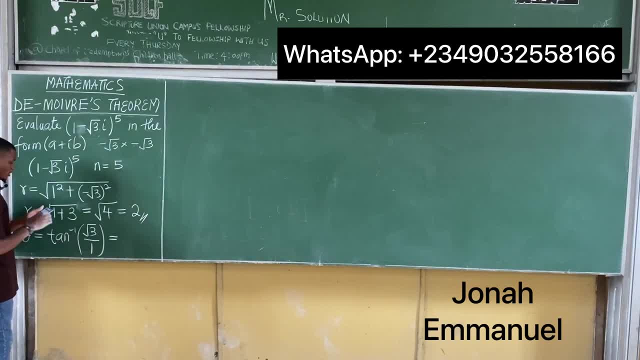 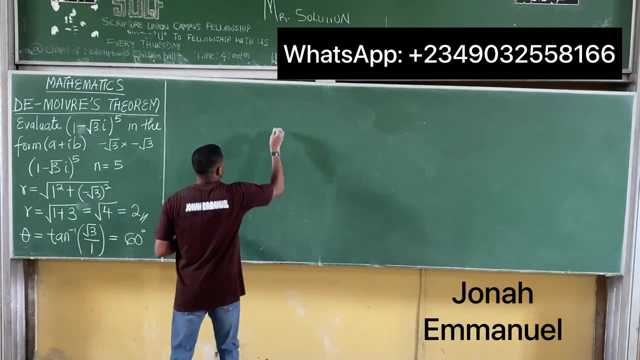 to let me write the answer here. this will give you root 3, so tan inverse of root 3. my answer here is 60 degrees. 60 degrees: here is my reference angle, which I explained in our previous class. so let's get the real value of theta. what will it be? 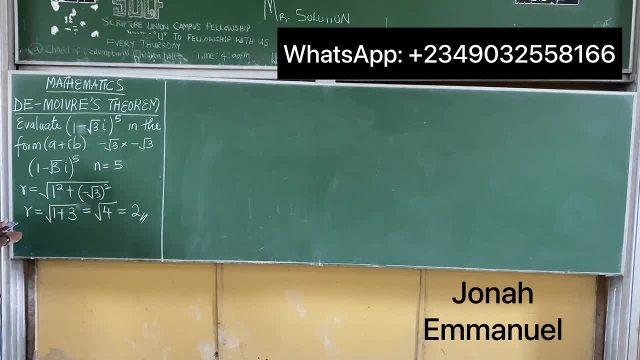 square root of 4 is 2.. So I have this as 2.. Next let's find the angle. So theta is equal to. before you watch this, please make sure you've checked our previous video on how I explained how to get theta and theta reference. 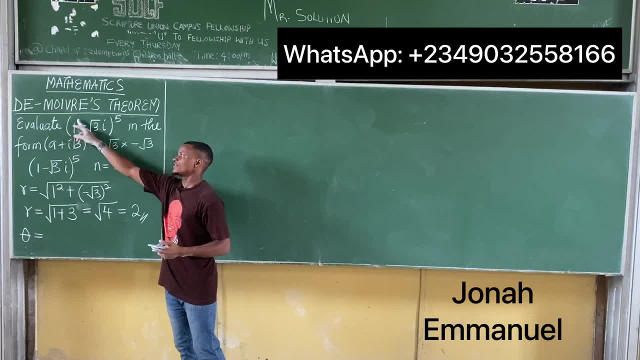 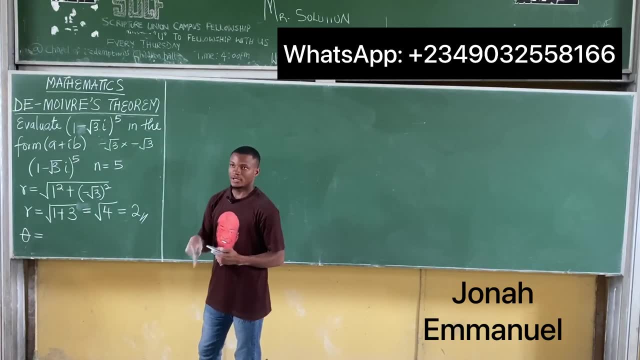 So for this one here you should know the quadrant positive x, negative, i, That should be quadrant 4.. And you know how you get the reference. I'll leave a link to that video in the description of this video. So just check the description. you'll see a link to the explanation of. 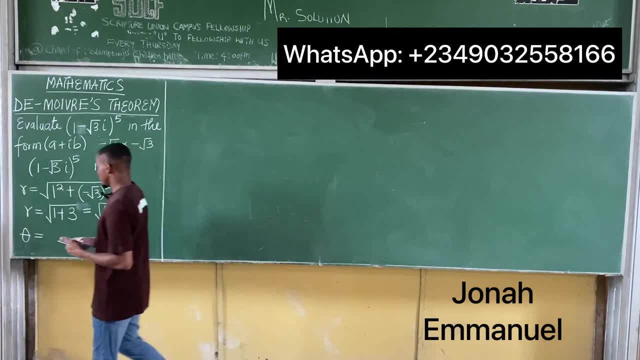 how you get the correct angle. But let's proceed with this. So that's equal to theta is equal to tan inverse. so tan inverse of. we said you could forego the negative sign. I'll just take root 3, only 1.. Okay, so b over a. 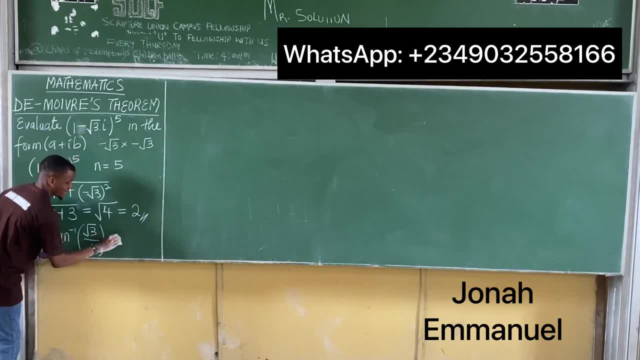 So theta is equal to. okay, let me write the answer here. This will give you root 3.. So tan, inverse of root 3.. My answer here is 60 degrees, 60 degrees. here is my reference angle, which I explained in our previous class. 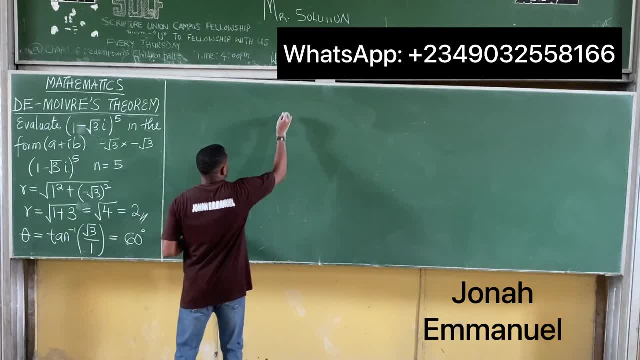 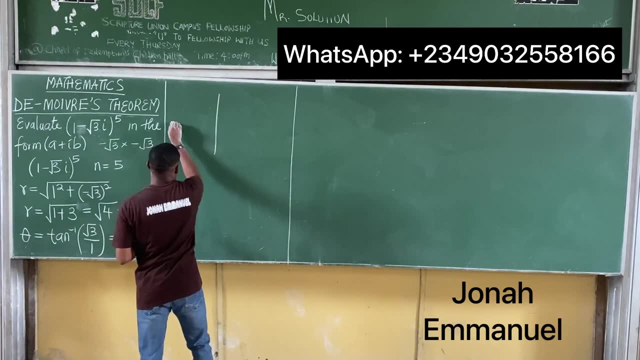 So let's get the real value of theta. What will it be? Let's see this. To explain this: in our previous class we said: you have this from the Adam's diagram, You have this and you have this, So I'm having this one here. 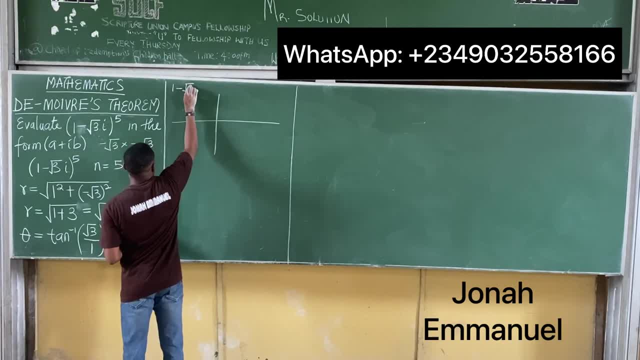 1 minus root 3i would be equal to 1 and minus root 3 here. So that's positive x, negative i. So positive x, that's here, Negative i, that's here. So hence something of this nature That's minus root 3.. 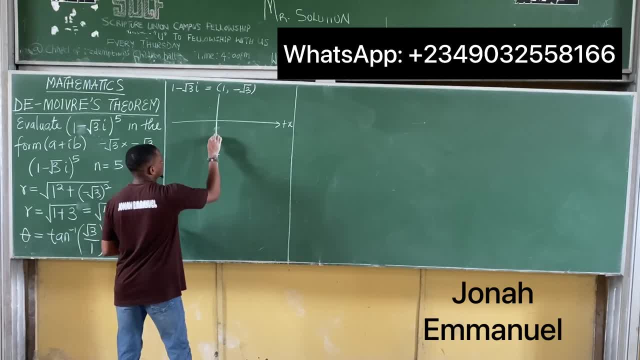 That's minus root 3.. That's about 1 point something Minus 1 point something, Because root 3 is 1 point something. So somewhere here minus root 3.. Then somewhere here 1 for x. So this one comes down. This one goes this way: 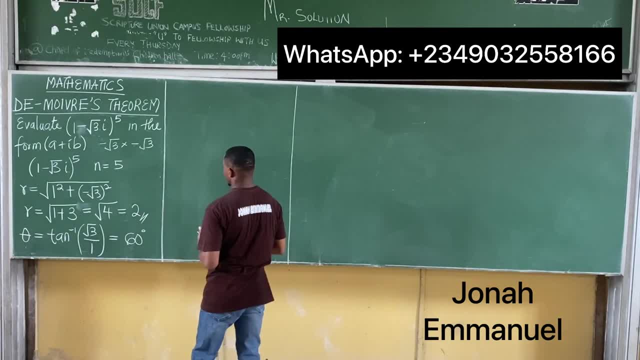 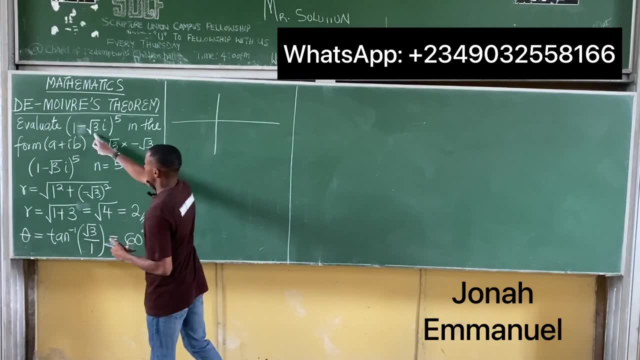 let's see this. we explained this in our previous class. we said: you have this from the other value, you have this, so I'm having this, this one here. 1 minus 1, minus root 3. i would be equal to 1 and minus root 3 here. 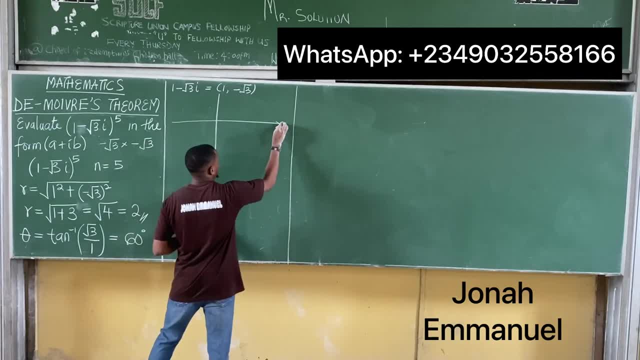 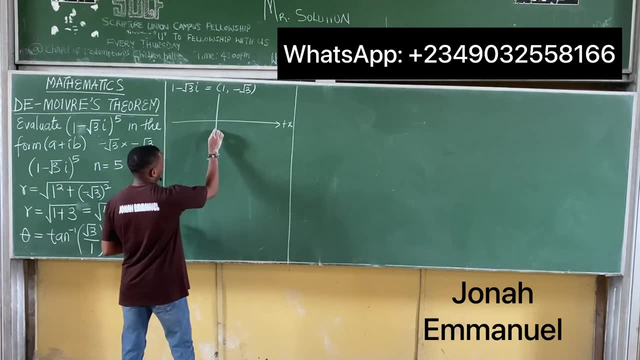 so that's positive x, negative i. so positive x, that's here, negative, i, that's here. so hence something of this nature. that's minus root 3, that's about 1.3 something minus 1. something, because root 3 is 1. something. 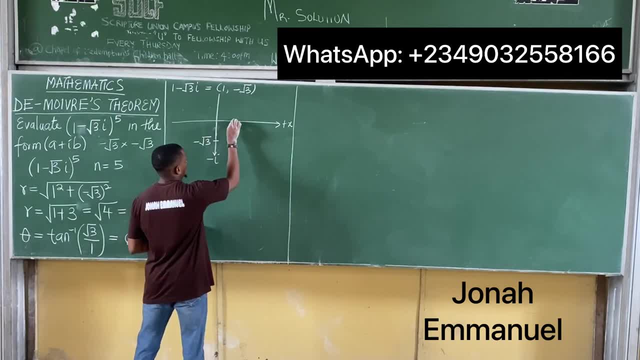 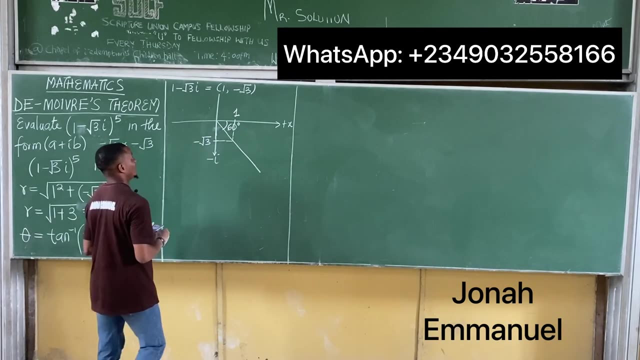 so somewhere here minus root 3, then somewhere here 1 for x, so this one comes down, this one goes this way and it will go like this: the theta you have is this one here: 60 degrees. okay, this is my reference theta. um, so this is not just theta, but theta reference. 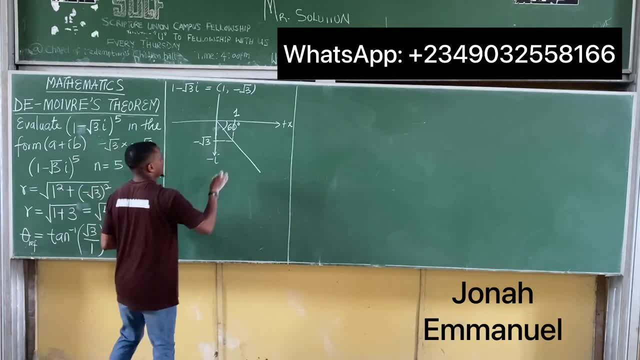 we explained this before now. okay, so my real value of theta would be: from here to this point, here, which, so this is theta reference. at 60 degrees, my real value of theta would be: what? there theta here? so we need to get theta here. we said this theta would be: 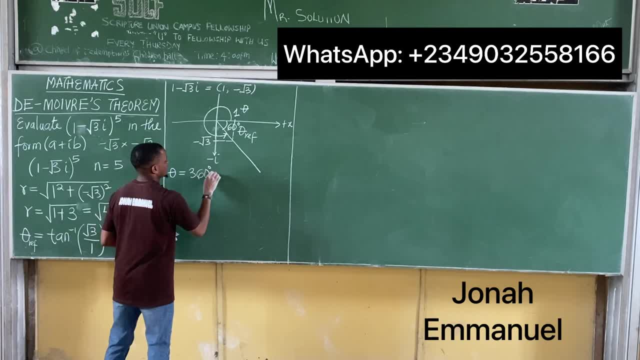 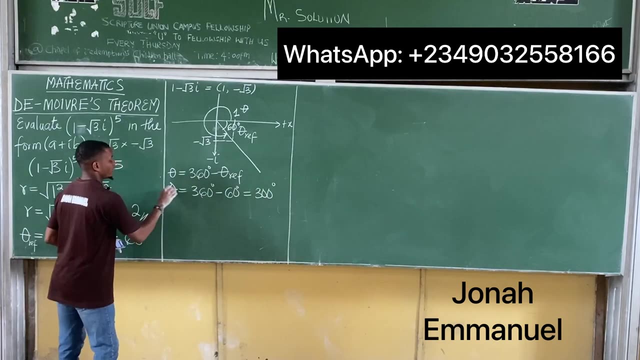 equal to 360, 360 degrees minus theta reference, and that's equal to 360 degrees minus. this value is 60 degrees, so my answer is equal to 300 degrees. this is the real value of the complex number that theta is equal to 300 degrees. 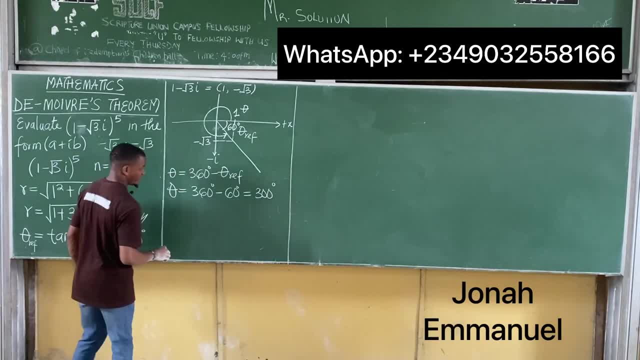 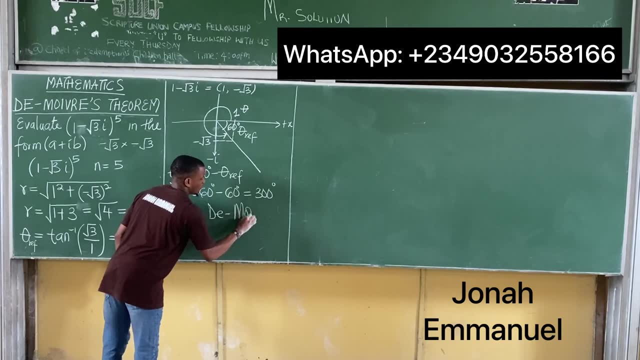 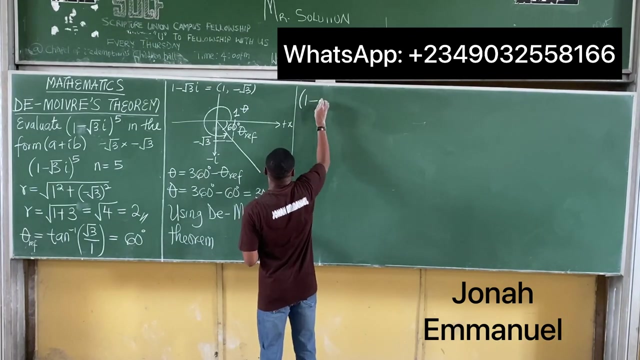 alright, so this is true. we can now use the moivre's theorem. so using the moivre's theorem, using the moivre's theorem, we'll have that, um one minus root 3, i to power 5 is equal to r to power n r here. 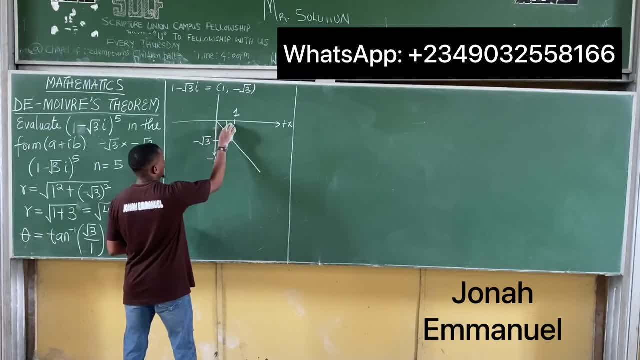 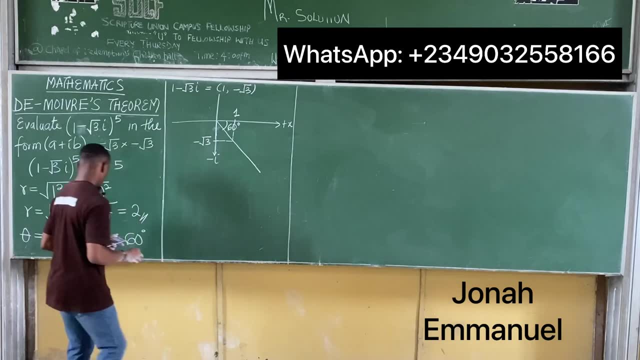 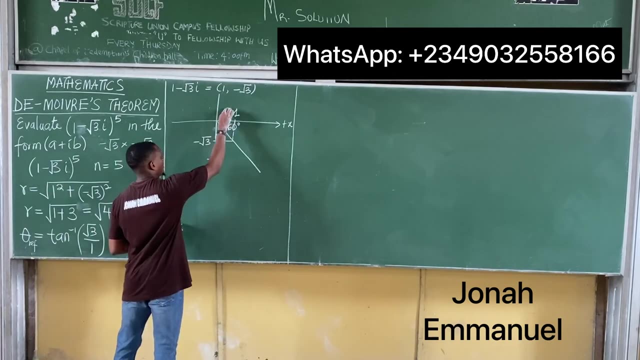 And it will go like this: The theta you have is this one here: 60 degrees. Okay, This is my reference theta. So this is not just theta, but theta reference. We explained this before now. Okay, so my real value of theta would be from here to this point here. 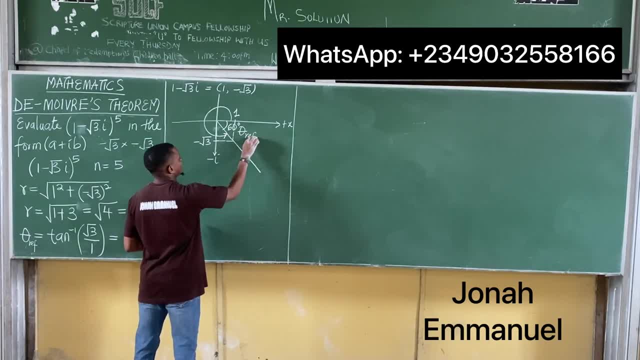 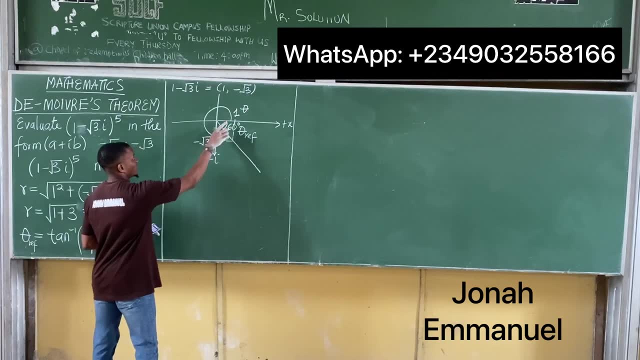 So this is theta reference as 60 degrees. My real value of theta would be: what there Theta here? So we need to get theta here. We said this theta would be equal to 360.. 360 degrees minus theta reference And that's equal to. 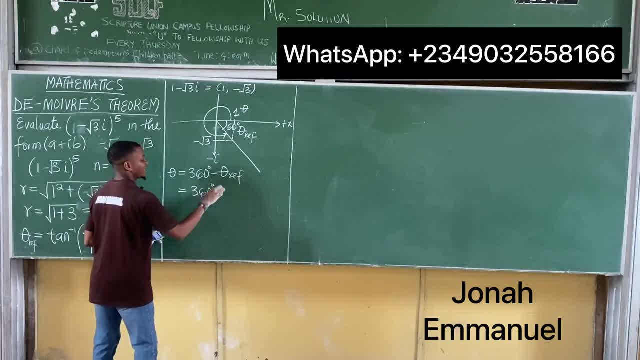 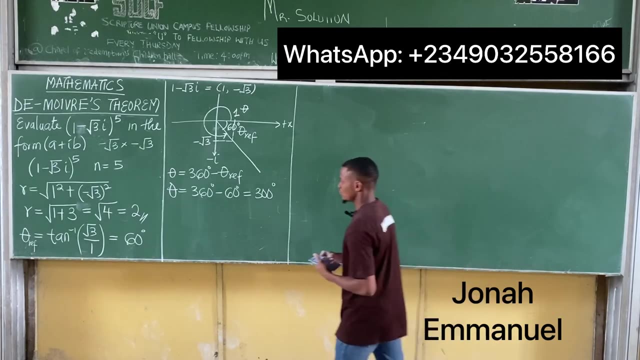 360 degrees minus this value is 60 degrees, So my answer is equal to 300 degrees. This is the real value of the complex number that theta is equal to 300 degrees. All right, so this is true. We can now use the Moivre's theorem. 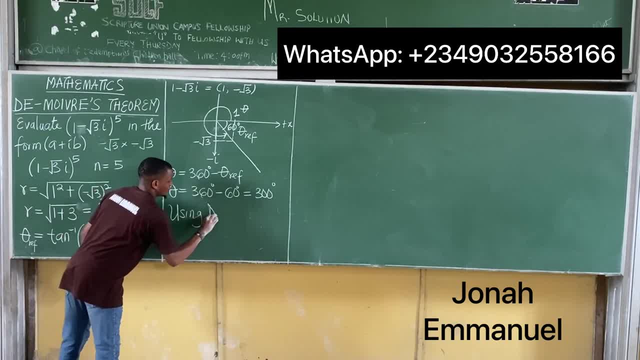 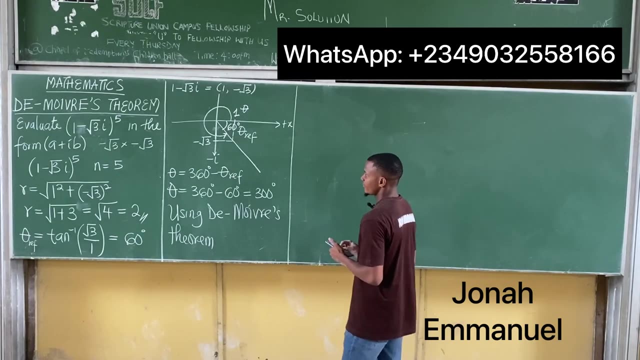 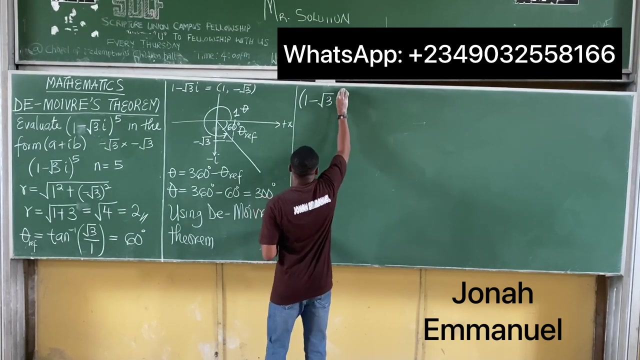 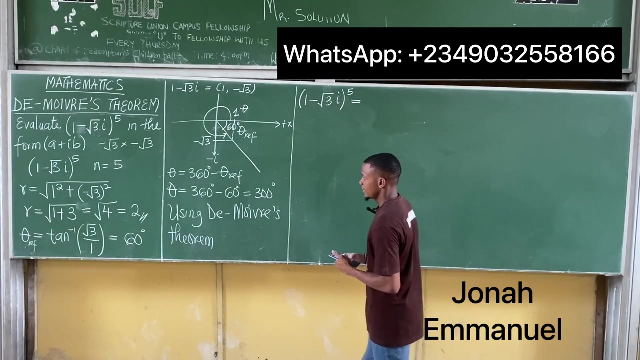 So, using the Moivre's theorem, Using the Moivre's theorem, we'll have that 1 minus root, 3i to the power 5 is equal to r to the power n. r here is 2.. So 2 to the power n, n is 5.. 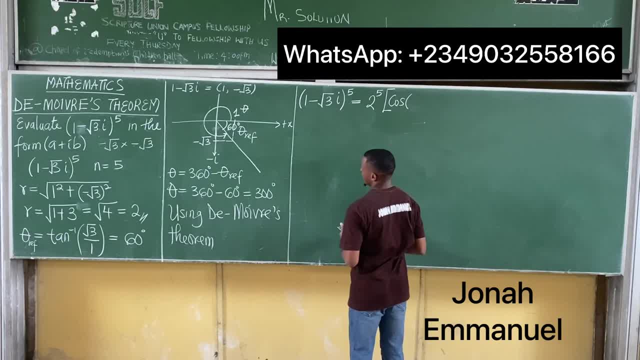 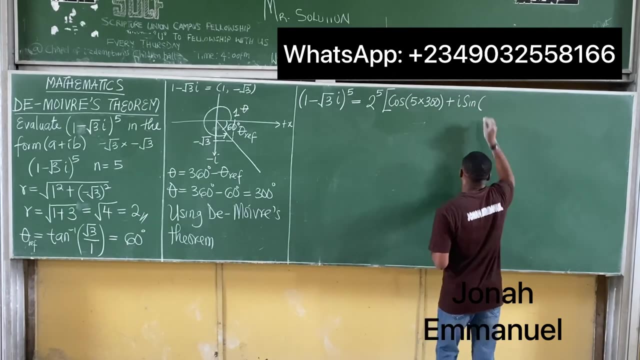 Into cos. So cos n times theta n is 5.. So 5. 5 times theta is 300.. So 300 plus i sine n, 5 times theta 300.. So we have this, This whole concept, here. we've done this in our previous class. 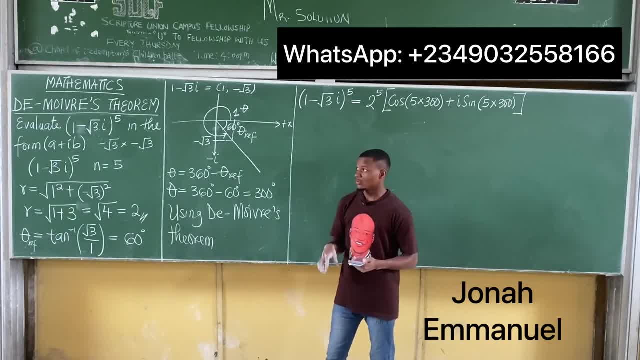 To access this video, simply check the description of this video. So if you check the description of this video, you'll see a link that explains what we just did here. All right, so I have this one here. Let's simplify this. 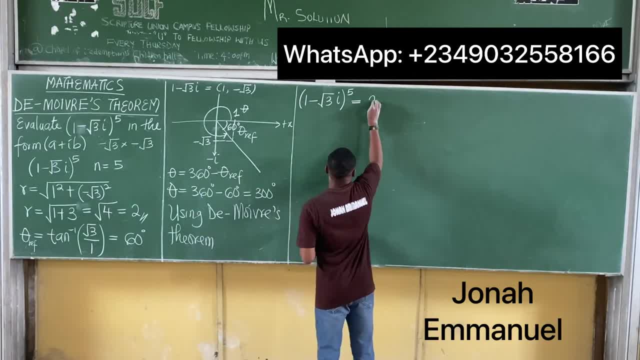 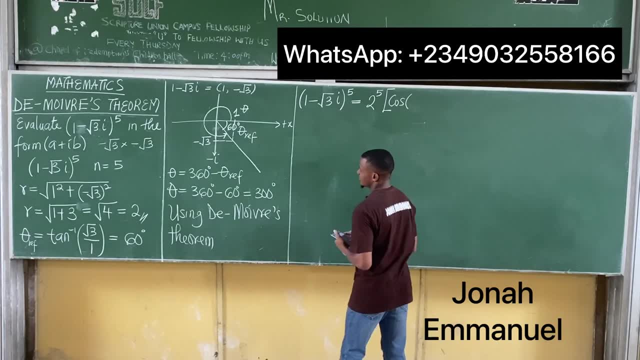 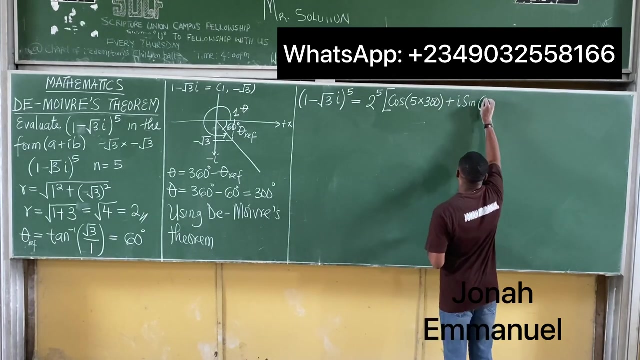 is 2, so 2 to power n n is 5 into cos. so cos n times theta n is 5, so 5 times theta is 300, so 300 um plus i sine n, 5 times theta 300. so we have this: 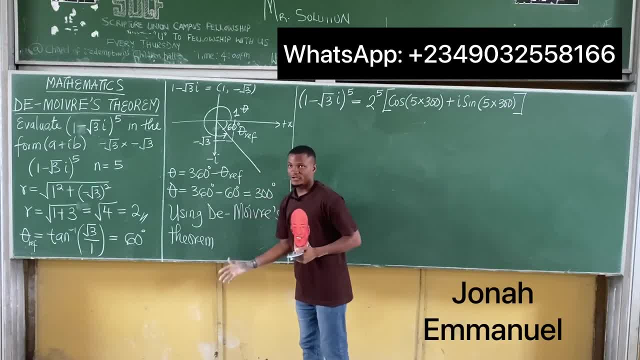 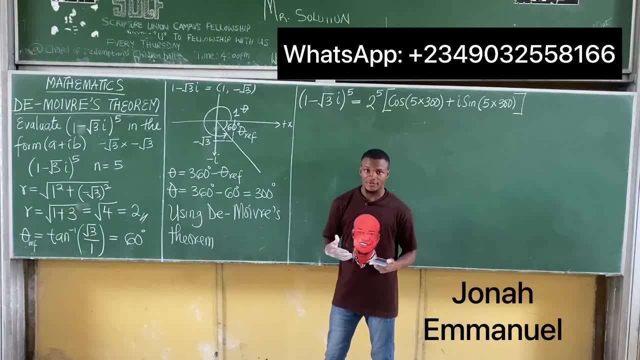 so i'm saying again this whole concept here. we've done this in our previous class. so to access this video, simply check the description of this video, right? so if you check the description of this video, you'll see a link that explains what we just did here. 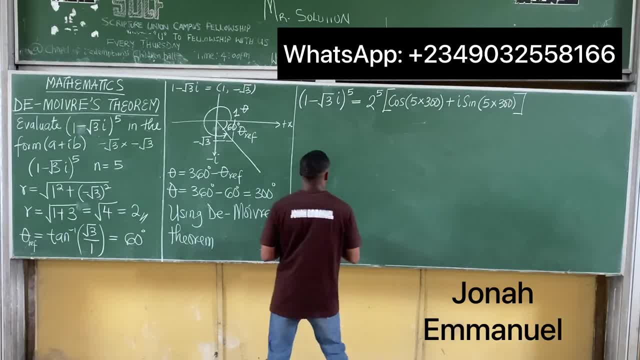 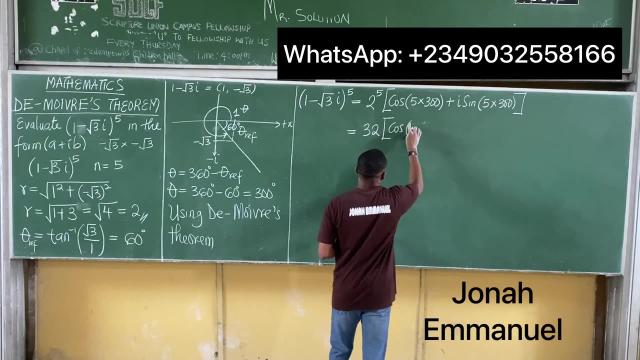 alright, so i have this one here. let's simplify this. so this is equal to 2 to the power. 5, that's um 32. 2 times 2. 4 times 2, 8, that's 32. so 32 into um cos. this gives you 1500. 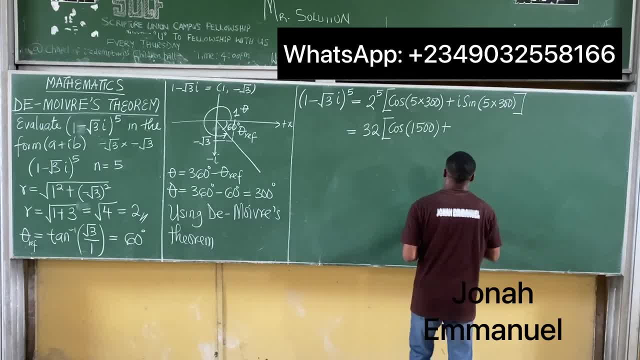 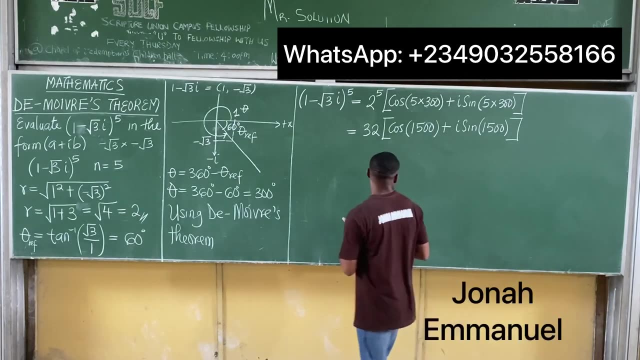 plus i sine 1500. so i have this, so we can go ahead and punch cos 1500. okay, so we have an answer here. so this is equal to 32 if i punch cos 1500. this is in degrees. this is in degrees, okay, degrees. 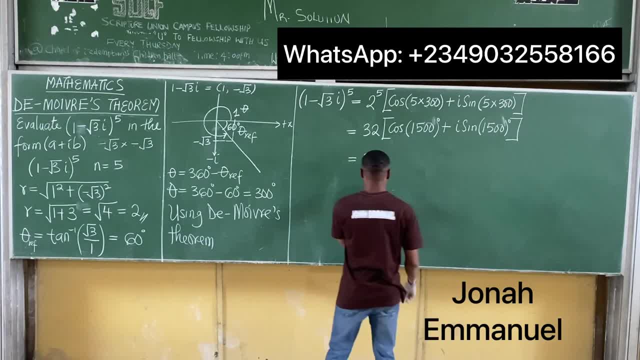 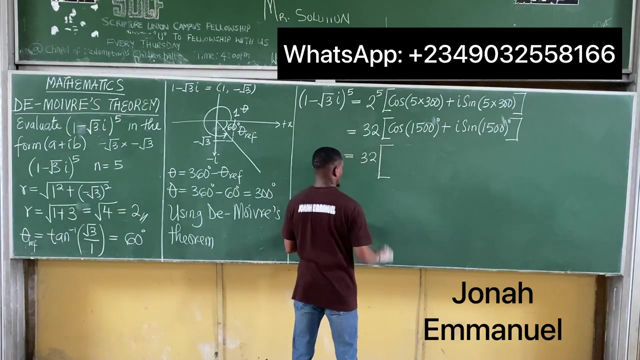 degrees. this way, alright, cos 1500 is equal to minus root 3 all over 2 plus. there should be this one here that's equal to 32 into. i'm having this: cos 1500 is equal to 1 over 2 plus i sine. 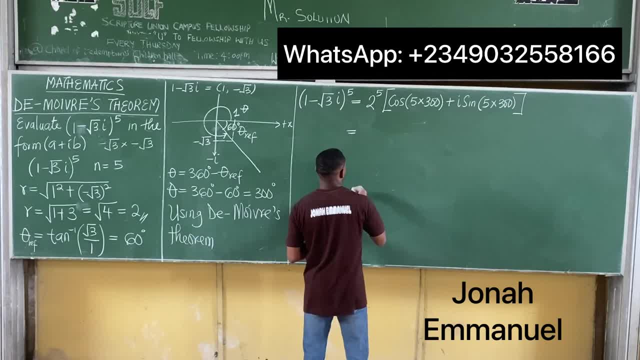 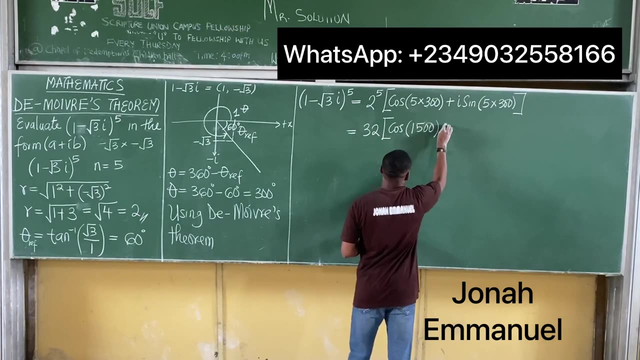 So this is equal to 2 to the power 5.. That's 32.. 2 times 2.. 4 times 2.. 8 times 2. That's 32.. So 32 into cos, This gives you 1,500 plus i sine. 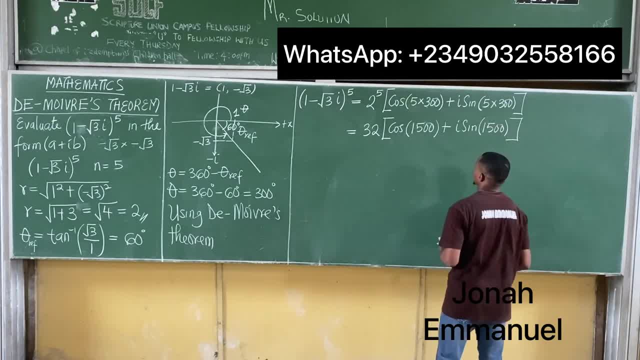 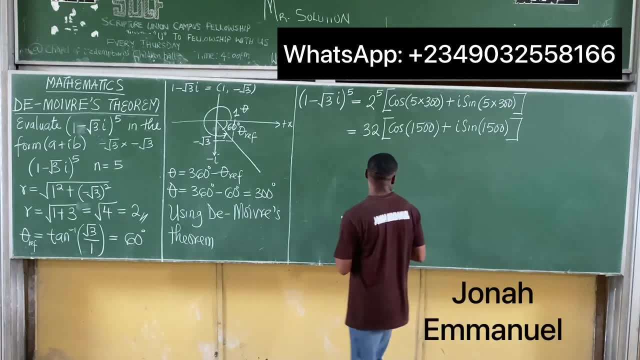 1,500. 1,500. 1,500. 1,500. 1,500. hundred. so I have this, so we can go ahead and punch cost one thousand five hundred. okay, so you have an answer here. so this is equal to thirty two if I. 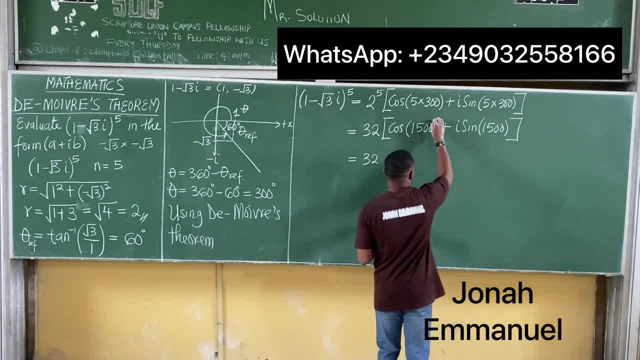 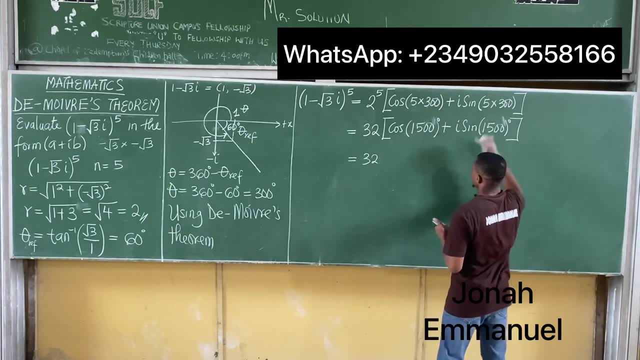 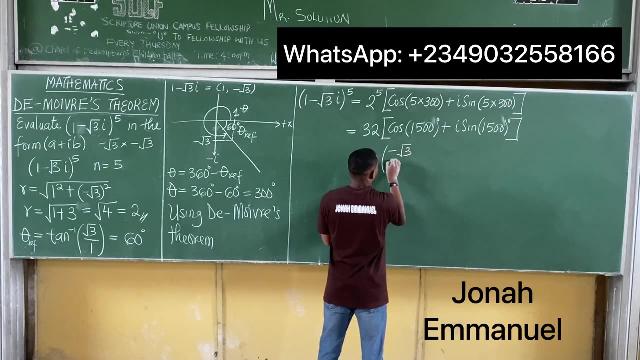 punch cross: one thousand five hundred. this is in degrees, this is in degrees. okay, degrees, degrees, this way, all right. cost: one thousand five hundred is equal to minus root three all over two plus there should be this one here. that's equal to thirty two into I'm having this cost one thousand five. 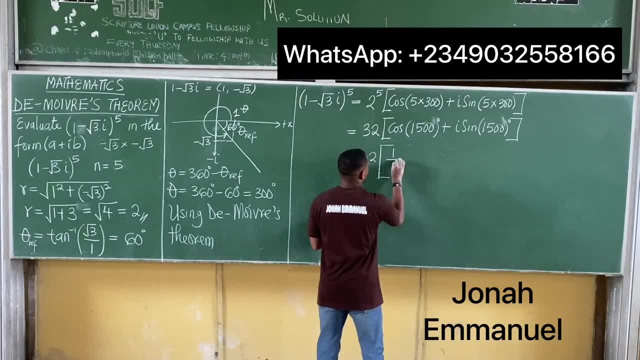 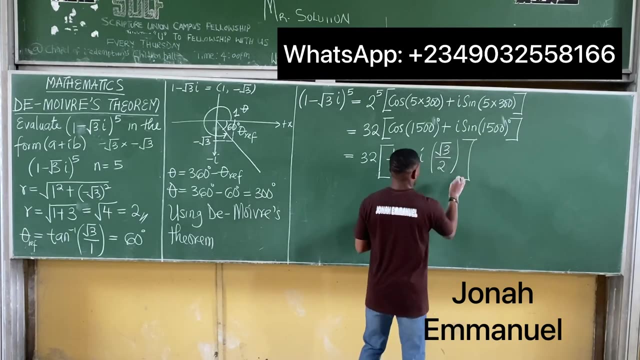 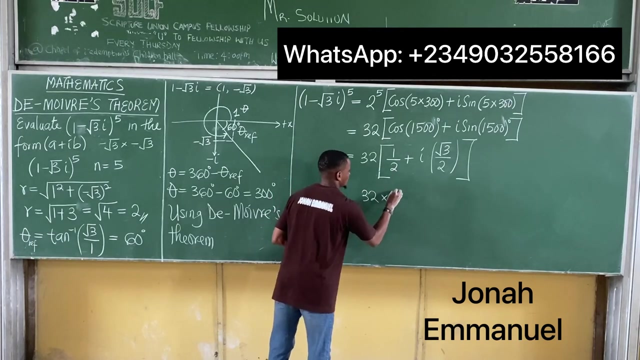 hundred is equal to one over two, plus I sign, one thousand five hundred is equal to three over two. so I have this. what I simply find. this is equal to this time, this thirty two times one over two, plus I, into this time, this thirty two one, and this will give us double x one, без一個乎ζ. 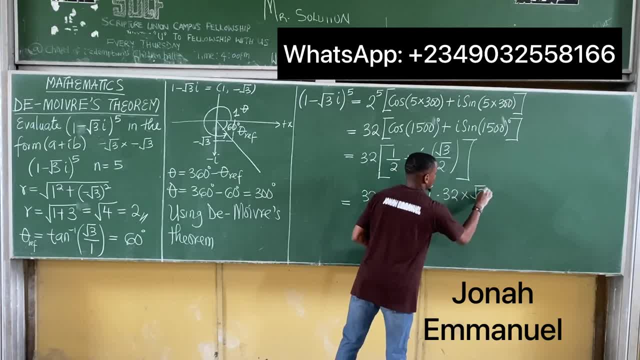 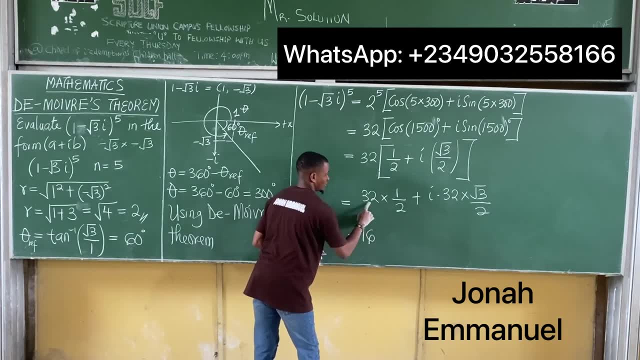 times this, 32 times root X, 1 over 2 is equal to 1 Piece 1 Over the lower, 3 over 2.. This is equal to 16.. So I'm having this as equal to 16.. So 2 times 1 over 2 is 16.. Plus i into. 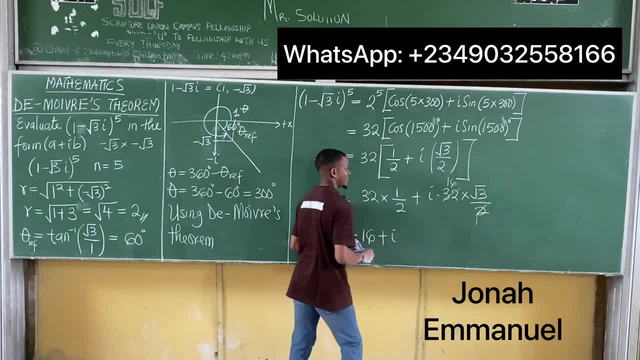 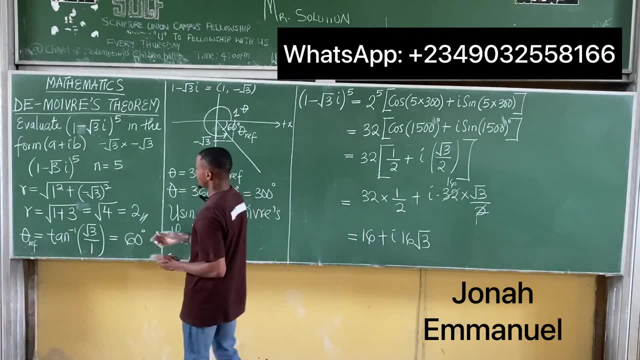 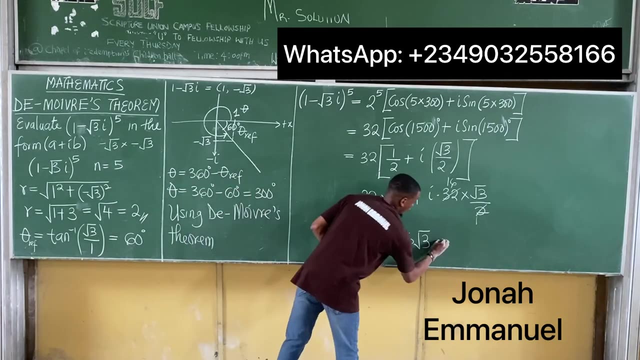 this here 1, this here 16.. 16 times root 3 is 16 root 3.. So this is the answer. here. The answer is expressed in the form a plus ib, So it becomes 16 plus this one here. Work on this further. This is equal to: 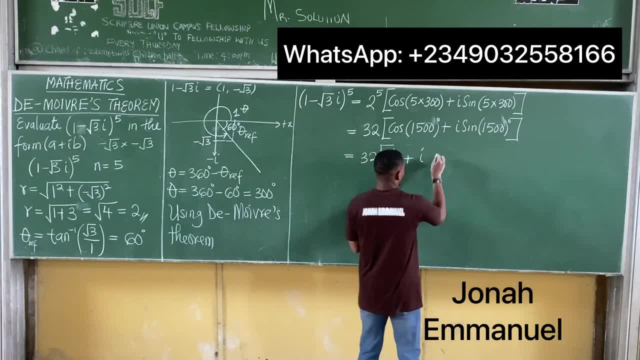 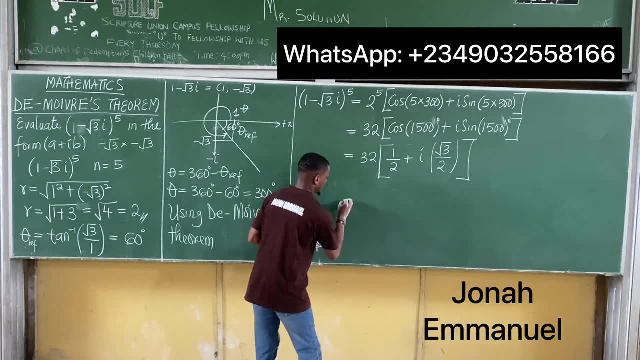 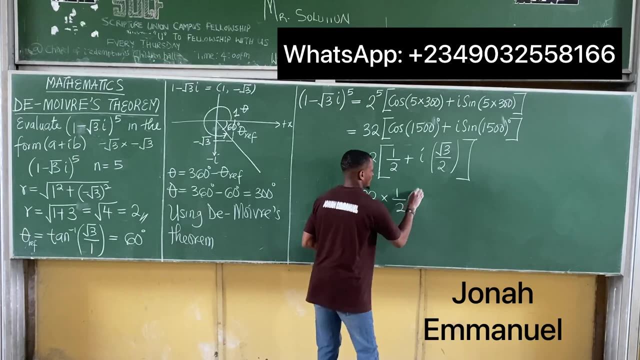 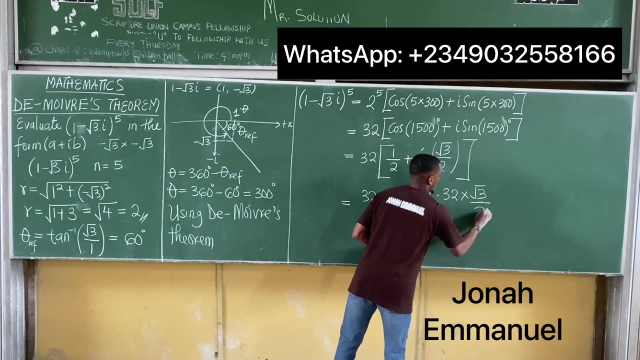 1500 is equal to root 3 over 2, so i have this alright. so simply find this is equal to this times this, 32 times 1 over 2, plus i into this times this: 32 times root 3 over 2, this is equal to 16. 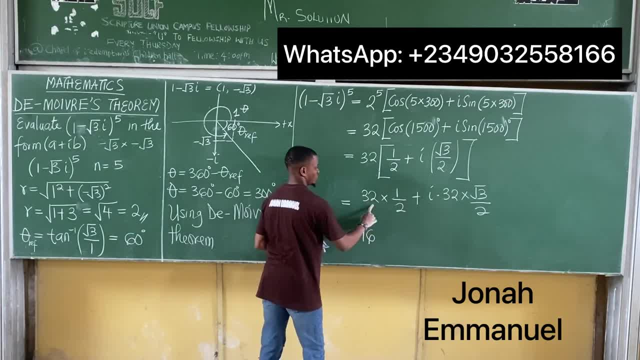 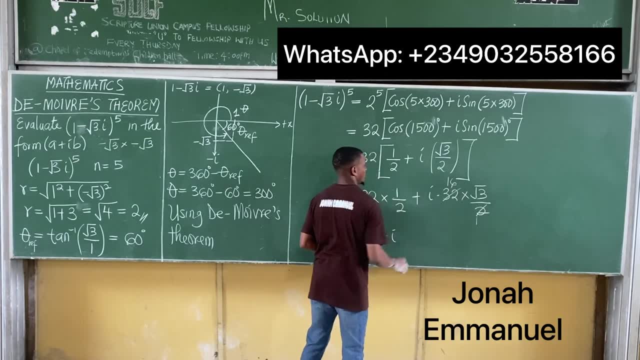 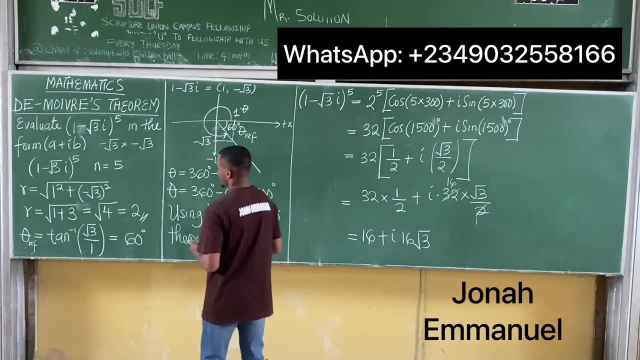 so i'm having this as equal to 16. so 2 times 1 over 2 is 16, plus i into this here 1, this here 16. 16 times root 3 is 16 root 3. so this is the answer here. that's expressing the. 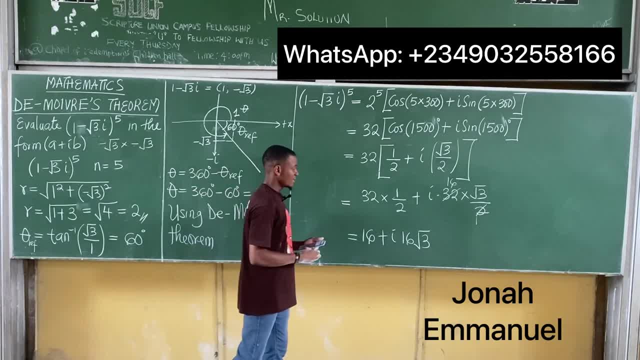 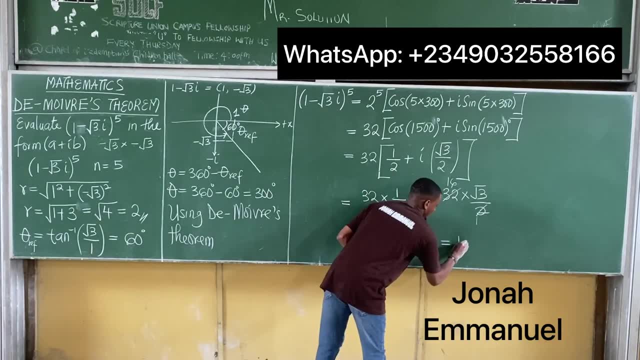 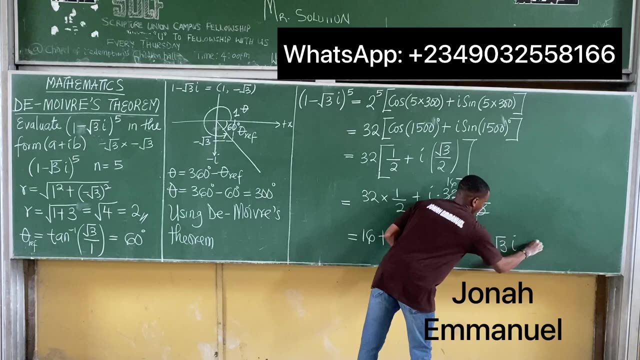 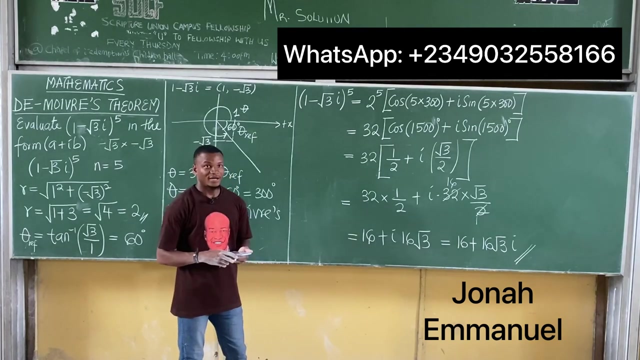 form a plus ib, so it becomes 16 plus this one here. work on this further. this is equal to 16 plus 16 root 3. i alright, so this becomes a final answer. if you want to factorise this, you are free to factorise, but that's a final answer. 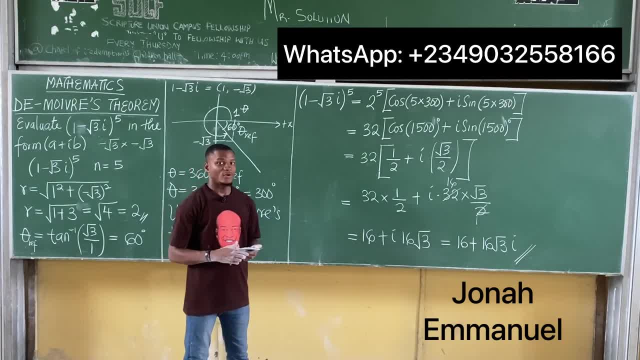 after solving this question. that's how we solve this. just to check this, let's see: 5 times 6300: okay, 300 cost 300, okay. so just to check this out, please. if you still use 60 here, our initial angle was 60 degrees. 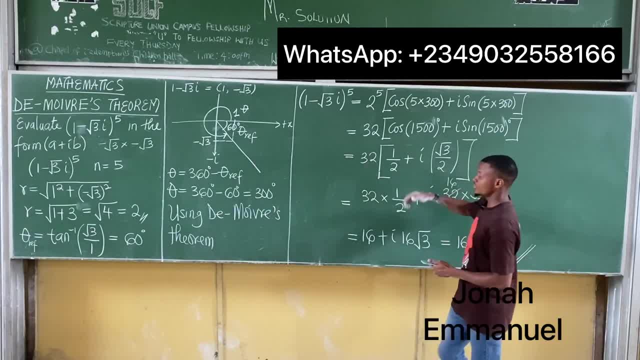 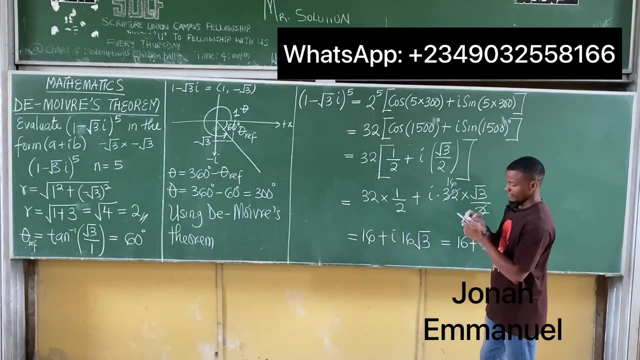 that was this one here. if we choose- if we still choose- to use 60 becomes 5 times 60. that's about 300. so cost 300 will still give you the same value as this sign 300. okay, so 300 gives you a negative. 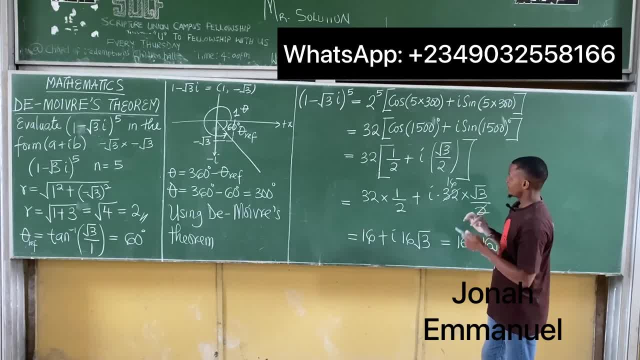 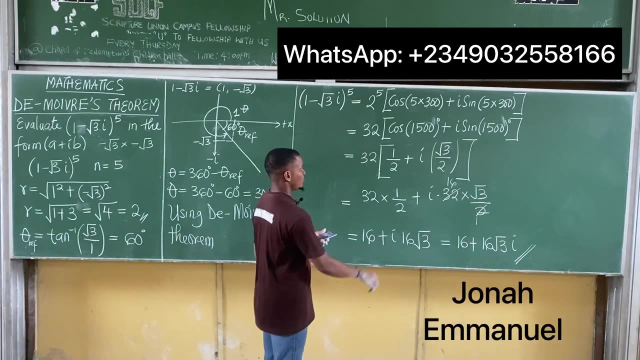 sign 1 500. okay, sign 1 500 gives you positive of this. if i use sign 300, it gives you a negative of this. so that's why this is very important. you get this concept. so if i use sign 1500, i'll have a positive of. 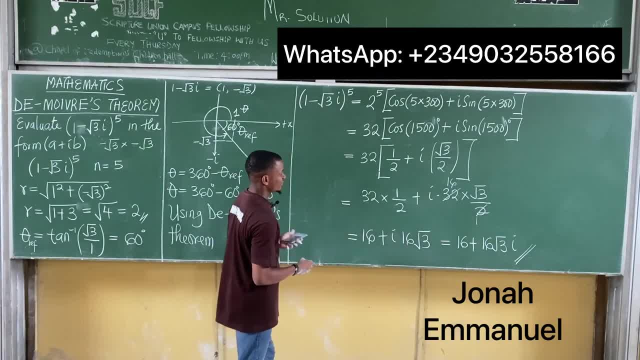 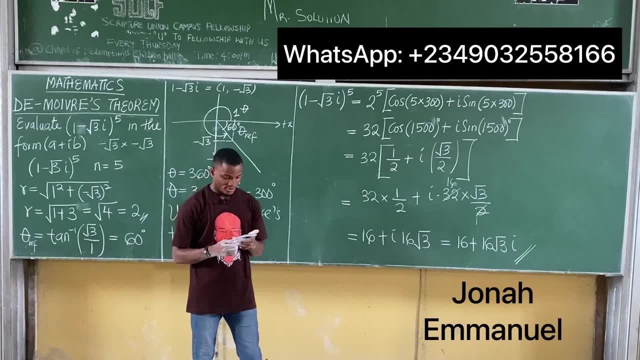 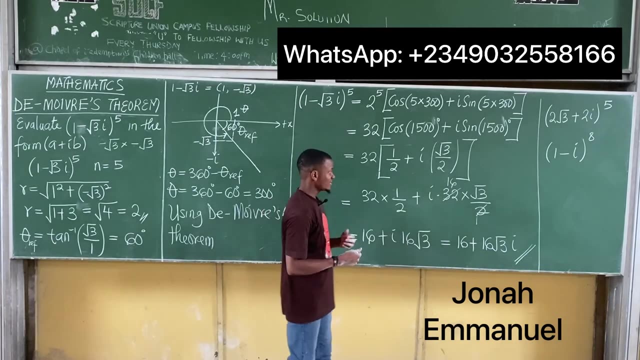 this y sign 300 gives me negative of this, so that's why it's important you have this concept, alright, so this is how we solve this question. we'll leave up two questions for you, so you try these two questions. alright, so this one we get. so observe that if 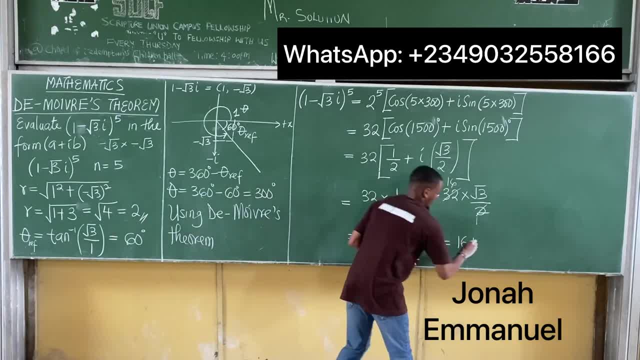 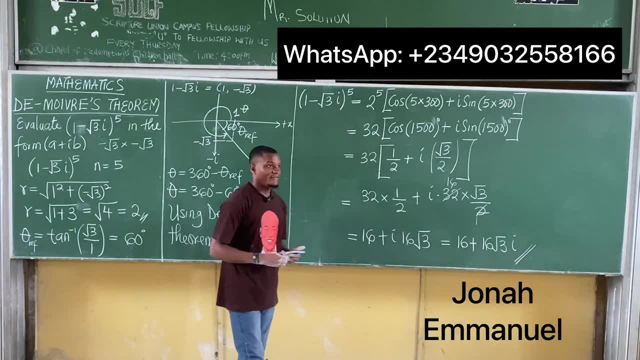 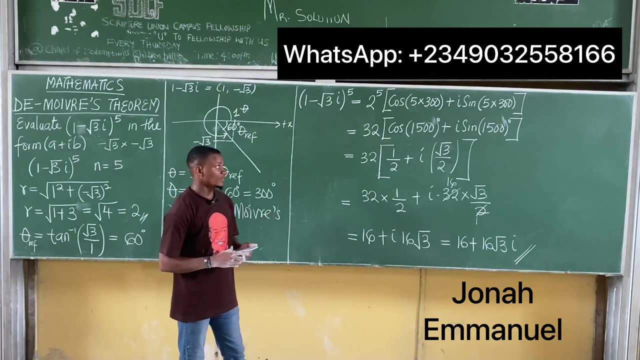 16 plus 16 root 3. i Alright, So this becomes our final answer. If you want to factorize this, you are free to factorize, But that's our final answer after solving this question. That's how we solve this. 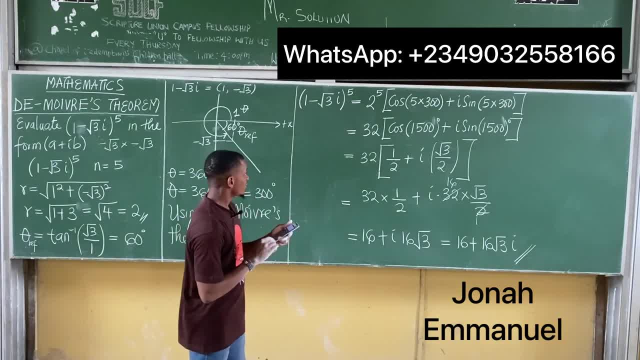 Just to check this. let's see 5 times 60: 300.. Okay, 300.. Cost 300. Okay. So just to check this out, please. If you see 60 here, our initial angle was 60 degrees. That was this one here. 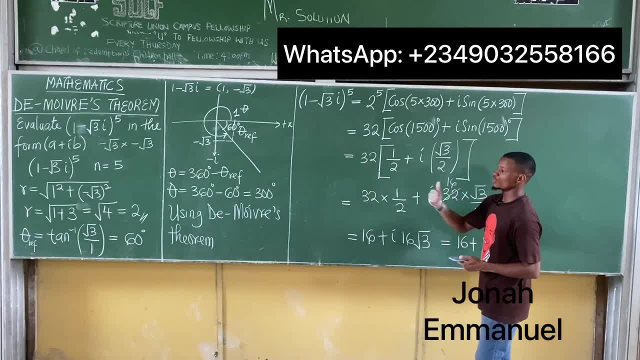 If you still choose to use 60, it becomes 5 times 60.. That's about 300.. So cost 300 will still give you the same value as this Sign 300. Okay, So 300 gives you a negative. 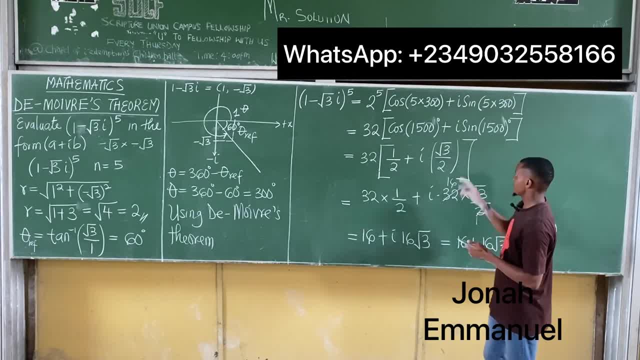 Sign 1 500.. Okay, Sign 1 500 gives you a positive of this. If I use sign 300,, it gives you a negative of this. So that's why this is very important. you get this concept. So if I use sign 1 500, I'll have. 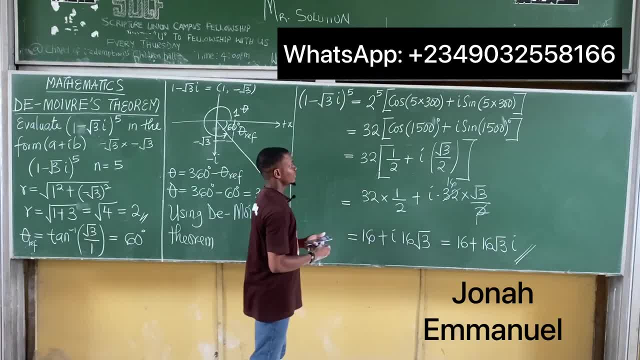 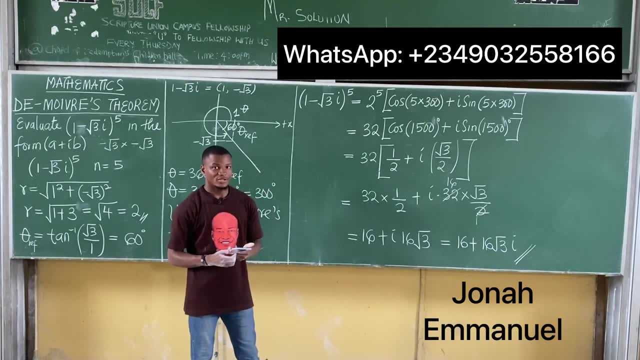 a positive of this, Why sign 300 gives me a negative of this? That's why it's important you have this concept, Alright? So this is how we solve This question. We'll leave up two questions for you, So you try these two questions. Alright, So this is what we get. 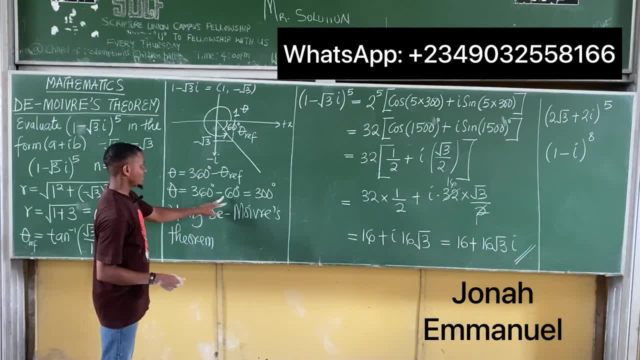 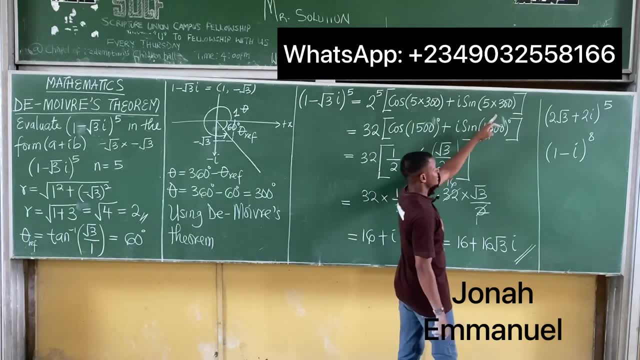 So observe that if I'd used theta 60 degrees here, then this would have been correct. I would have had 1 over 2, which is correct. But if I'd used theta 60 here, this would have been 5 times 60. 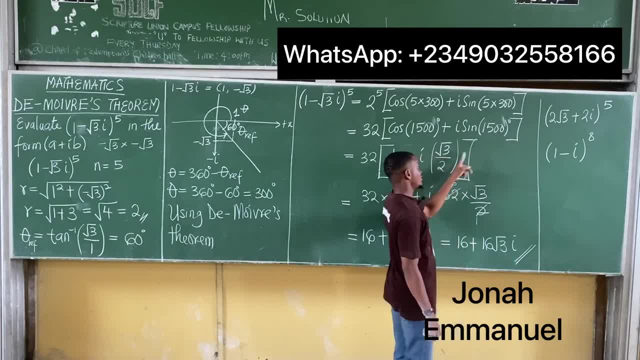 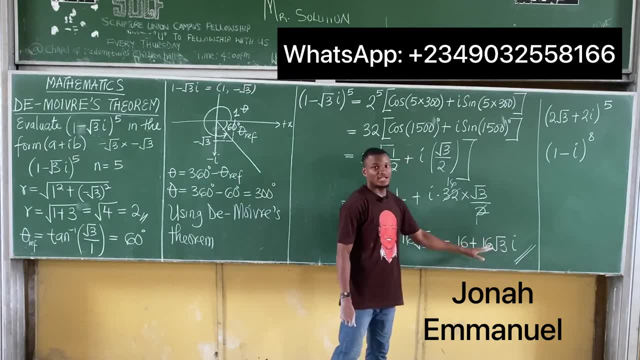 which would give me sign 300, and then this would now be negative of this. So I'll be having 16 minus 16 root 3. Which is incorrect. The answer is actually the plus and not the negative, So that's why Argan diagram is very important in our solution. 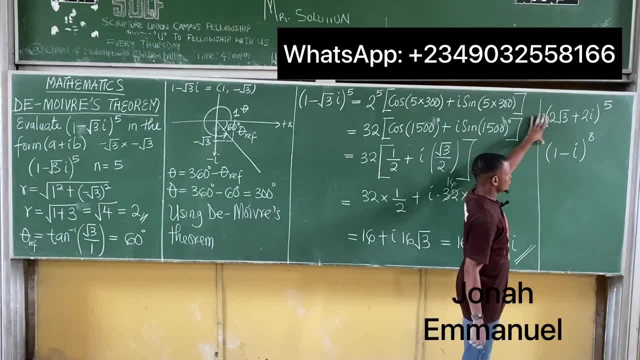 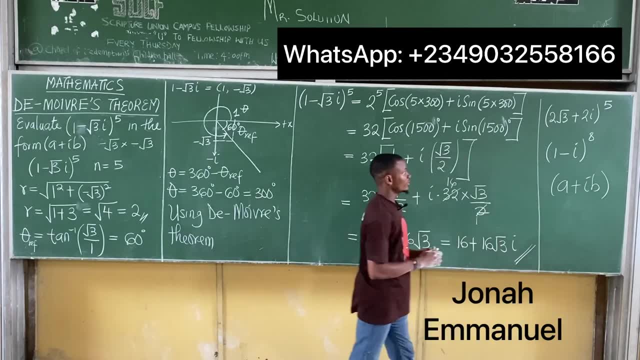 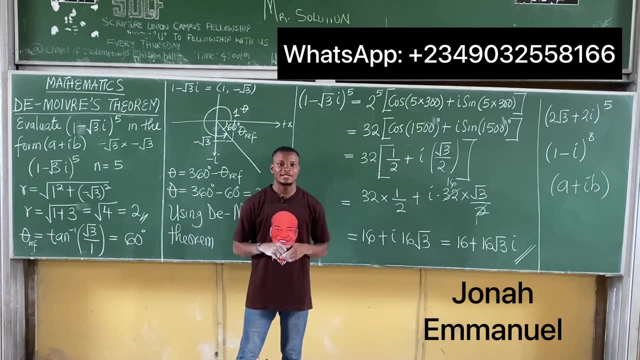 So, if you're done with this, please, please these two examples. solve this and express both of them in the form A plus IB. Please, when you're done, leave your answer in the comment section. Alright, then See you in the next class. We'll be right back.